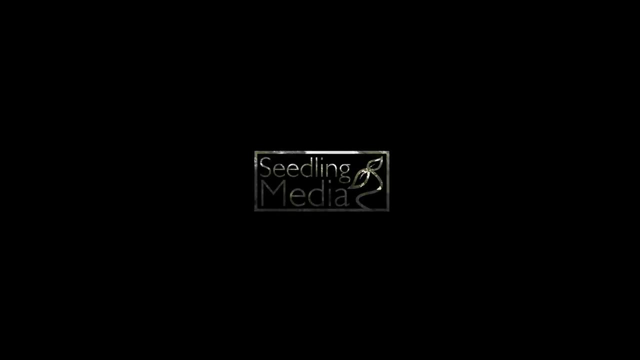 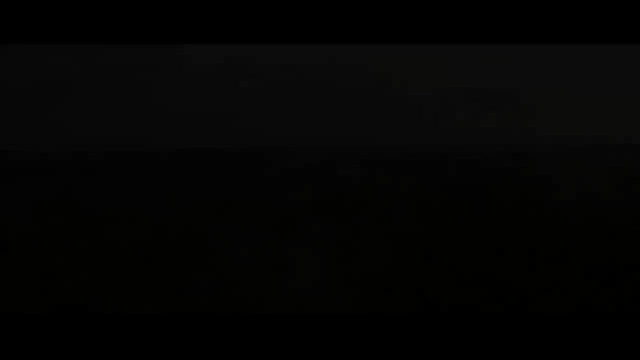 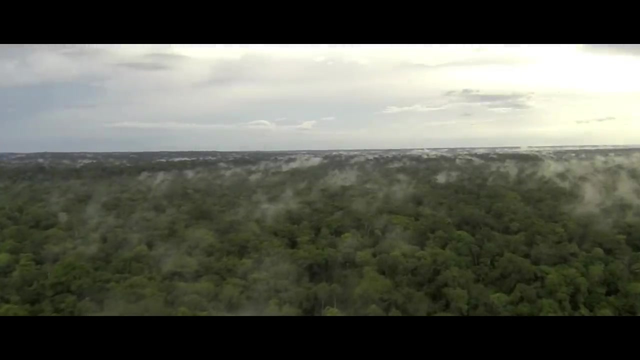 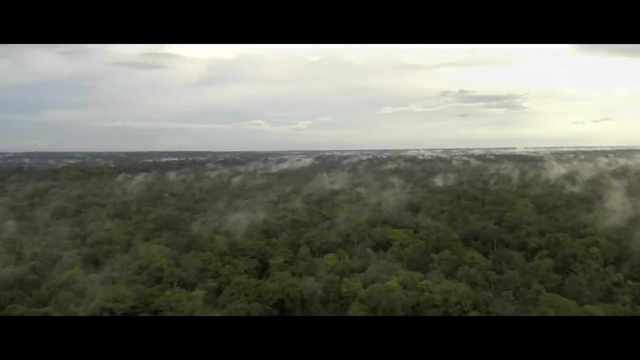 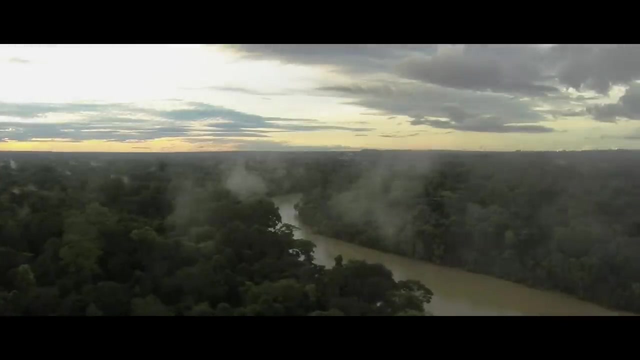 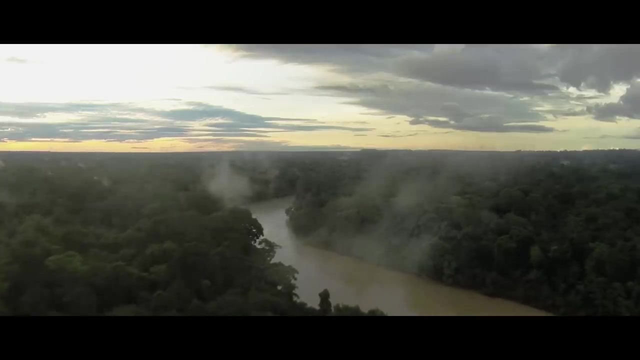 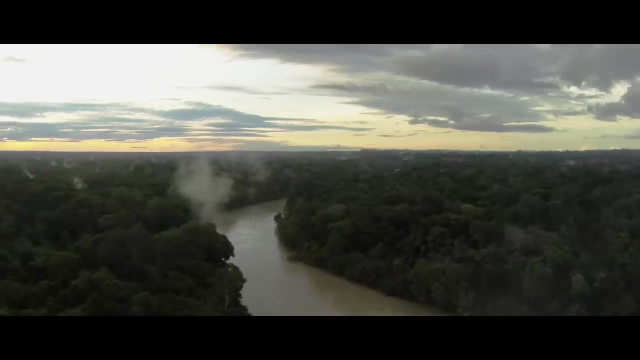 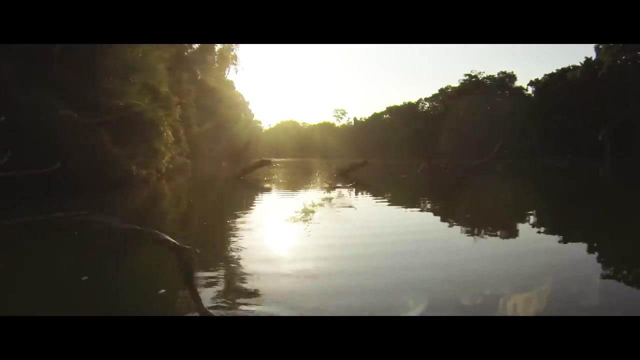 The Amazon Rainforest, the planet's impenetrable green sea. Within these remote depths runs the Las Piedras River, which forms part of the longest tributary to the Amazon. In the jungles surrounding the headwaters of the river, life remains much as it has. 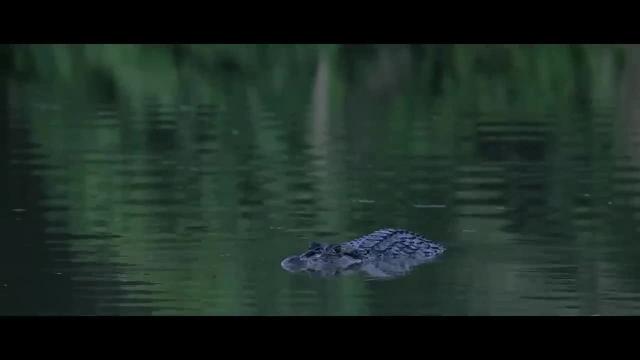 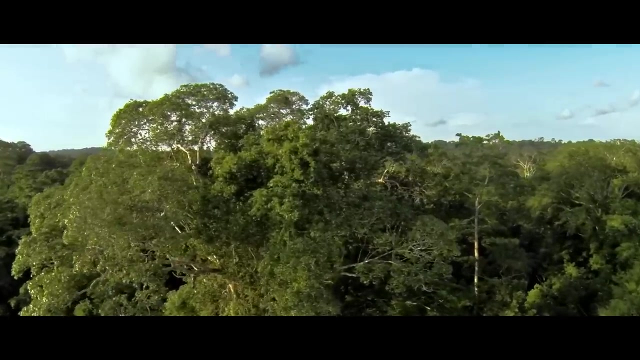 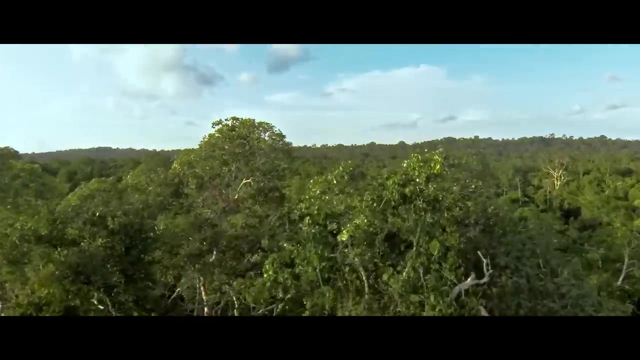 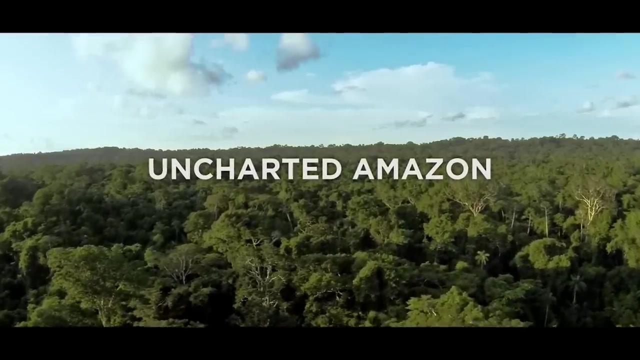 done for thousands of years, But no one knows where it fell or where it will go. The main thing about the Florida River, or the bondage of the river, is that it is a land full of wonderful nature, surrounded by the unique natural beauty of the Pacific. 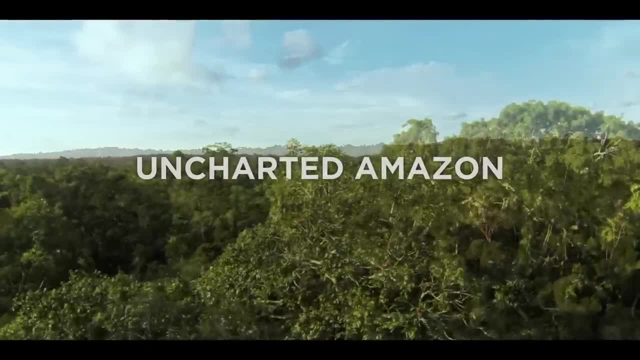 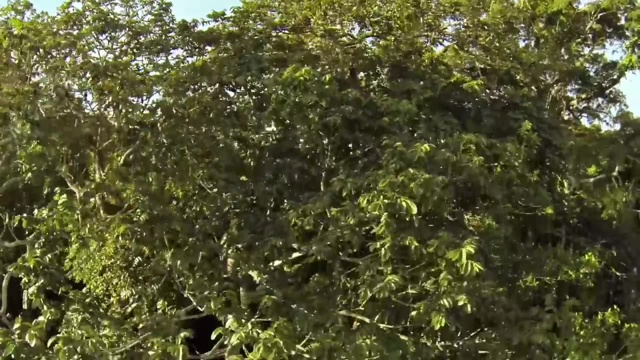 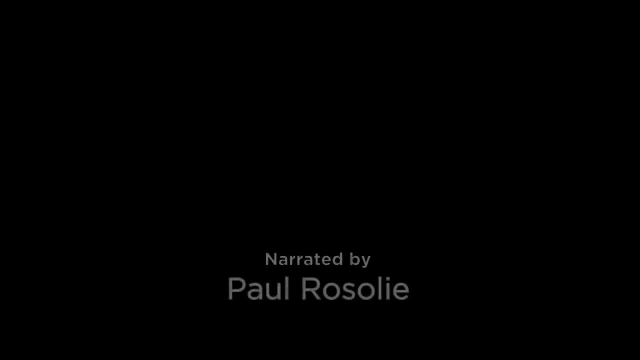 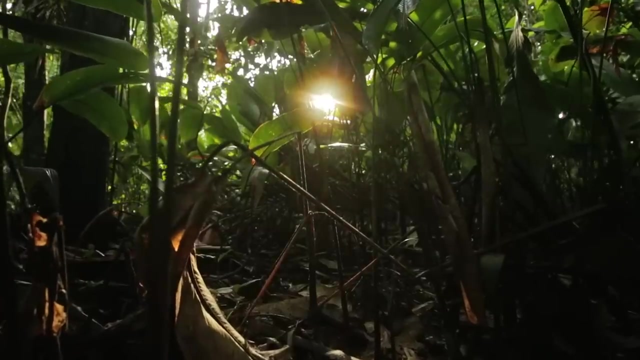 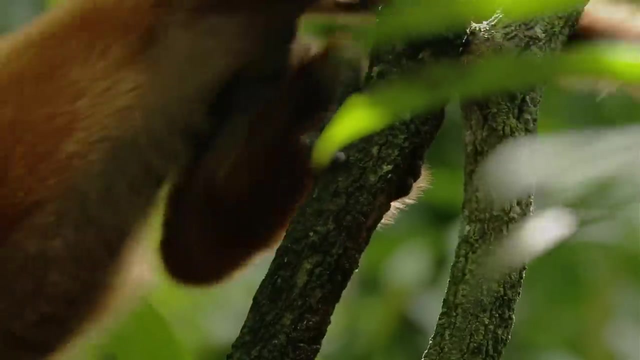 Sea. The riverline is well-intentioned, and now is a perfect place to go for a walk. 5.- 5.. Giants like these form a dense canopy shutting out the lights on those who dwell below. But within these dark halls, life can be found in such extraordinary abundance that only 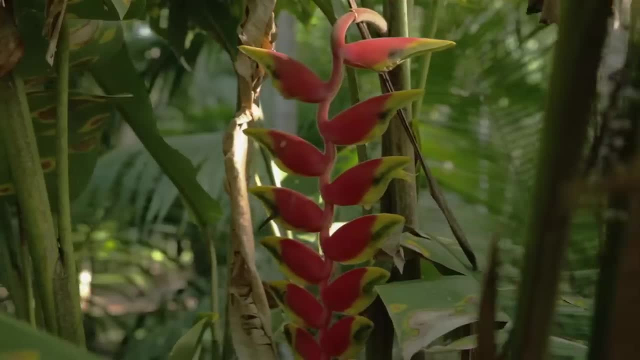 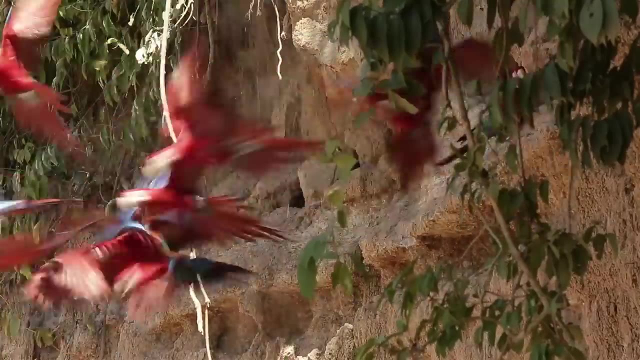 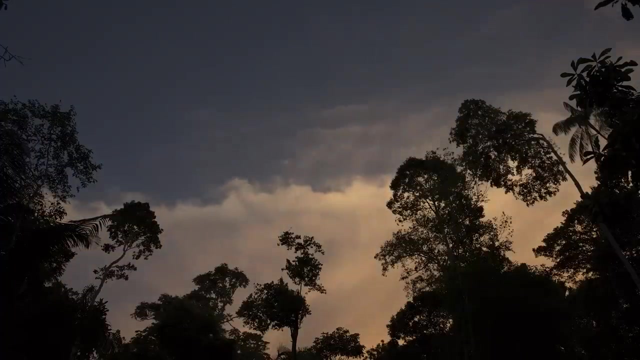 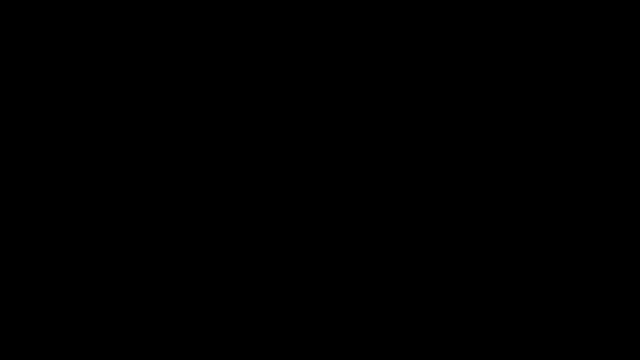 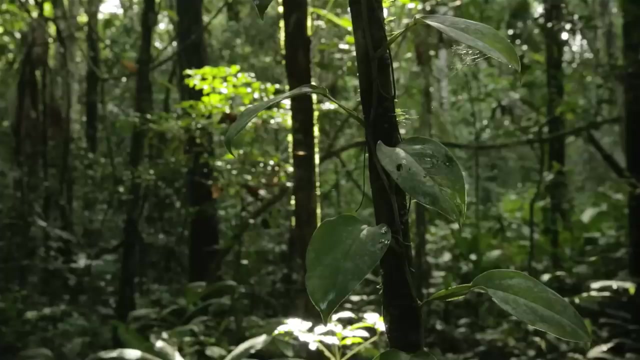 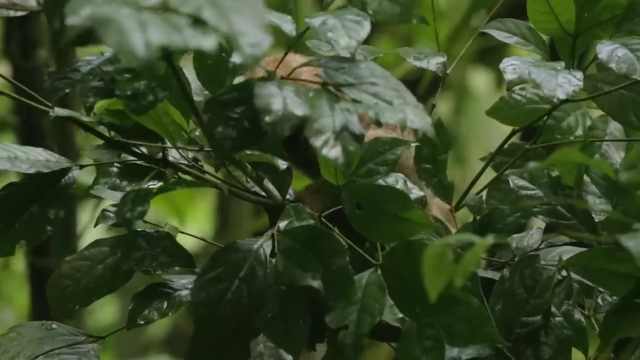 a fraction of its members have been counted, And this is with good reason, because survival below the treetops is often to remain hidden, And for much of her life this creature will remain so curled up amongst dense tangles of vegetation and rarely moving during the day. 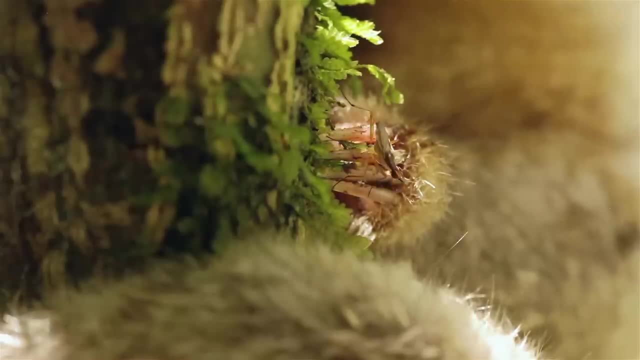 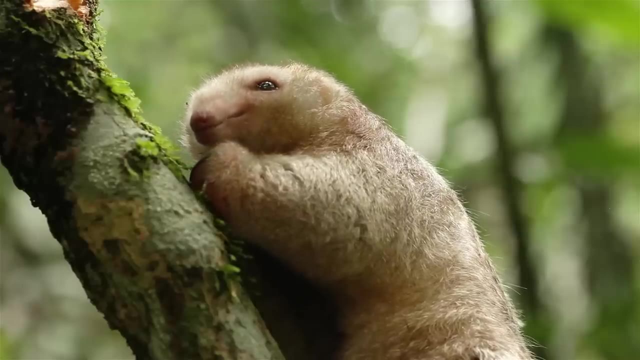 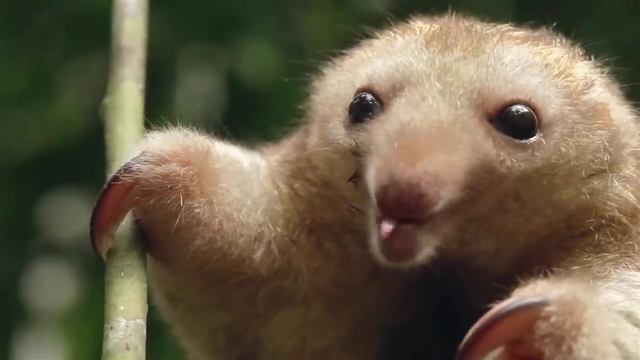 Her local name is Osito Oro, which means tiny golden bear. But while she might be both tiny and golden, she is certainly not a bear. She is a silky anteater. But don't let appearances fool you. The claws on her front feet can inflict serious wounds on anything that might try to harm. 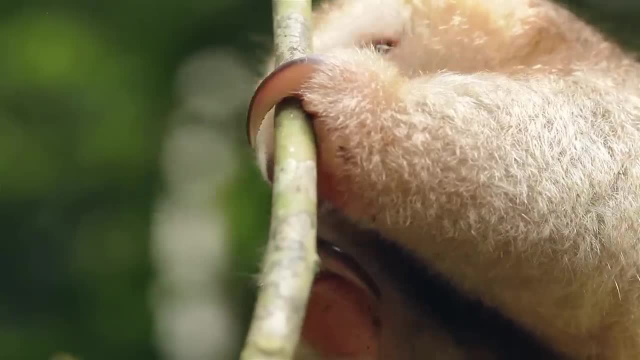 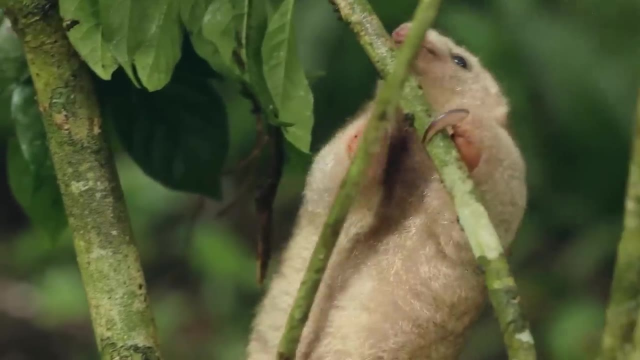 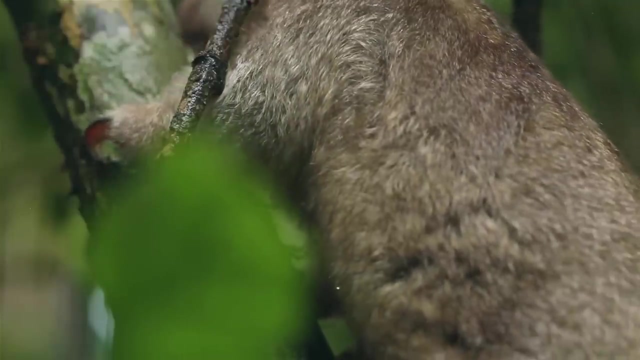 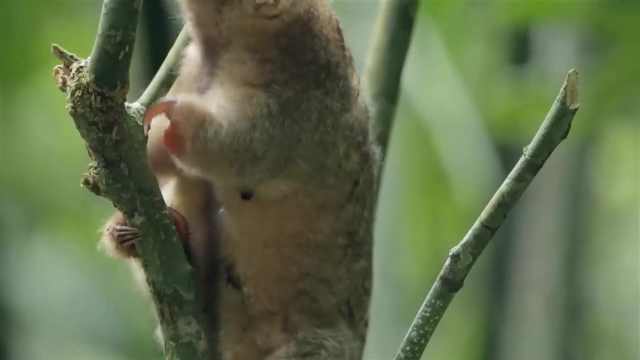 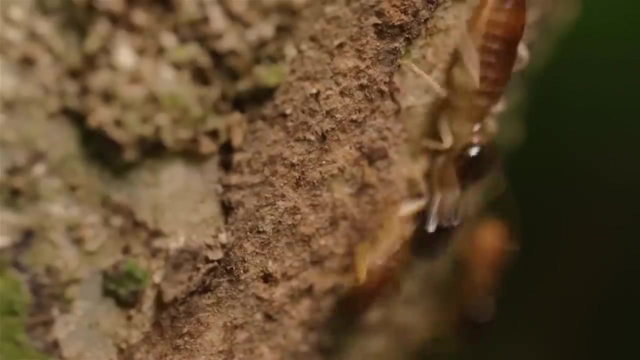 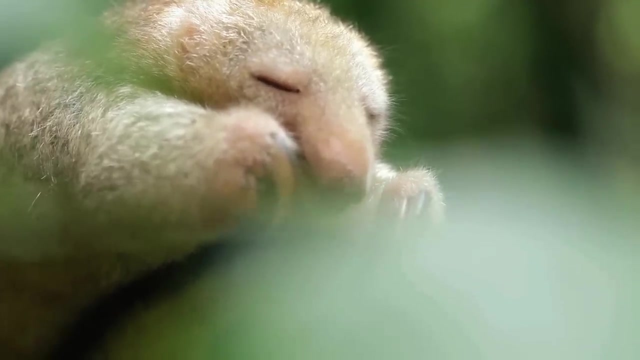 her. They are her only defense when she leaves her hiding places in search of food. And that's the end of the story. She's sniffing out her prey and being an anteater. this consists of ants and termites, But in order to find them, she has to overcome the considerable challenge of staying awake. 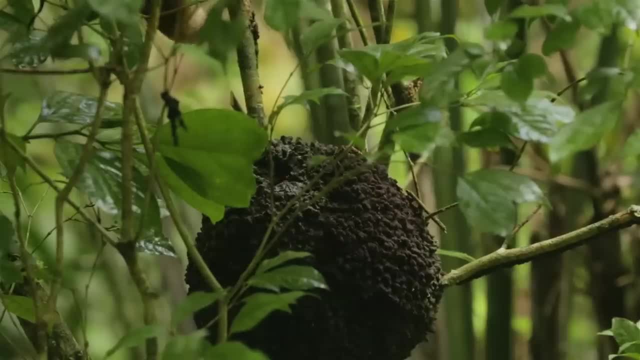 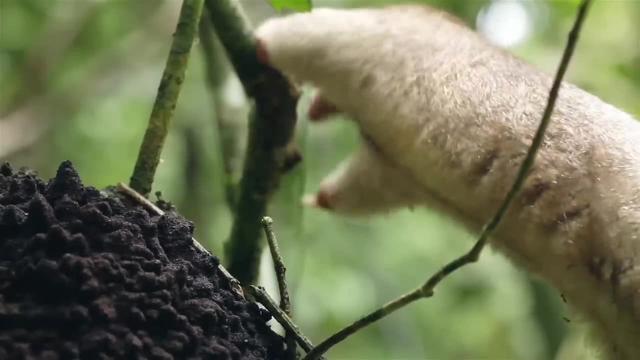 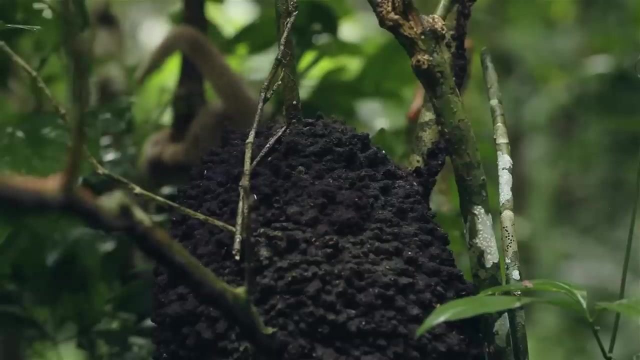 Once she's mustered up the strength to focus on the task at hand, she finds a termite nest and decides that it isn't quite the kind she's looking for. Keeping up appearances is important too, and a good grooming regime is sure to please. 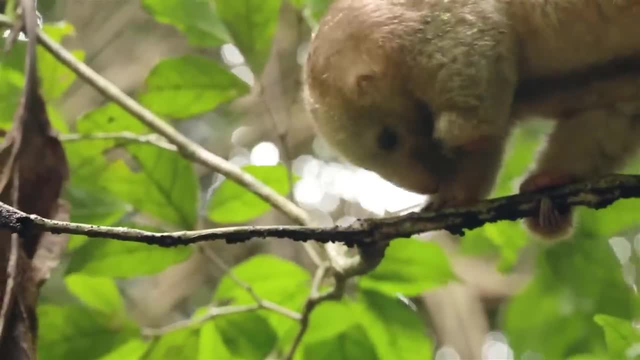 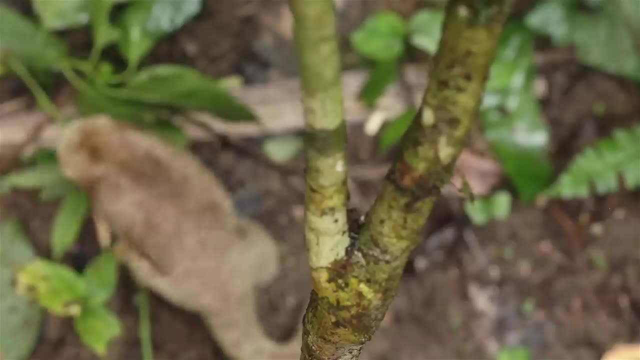 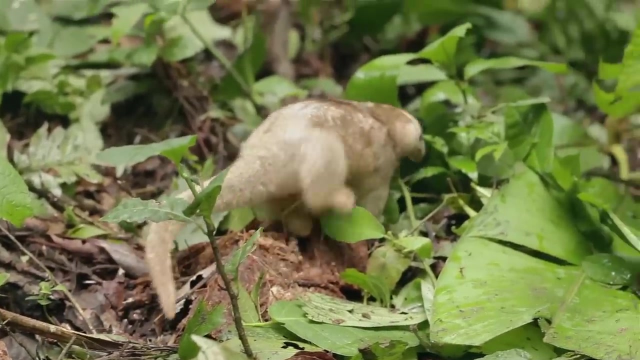 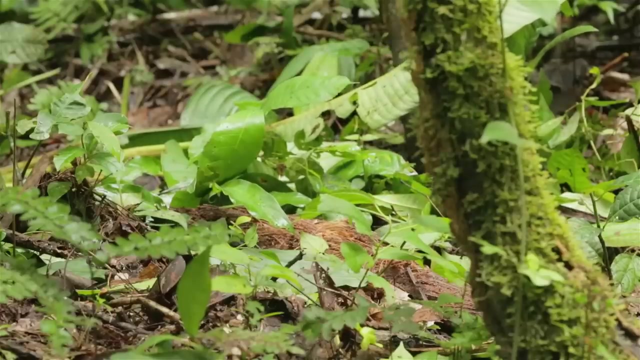 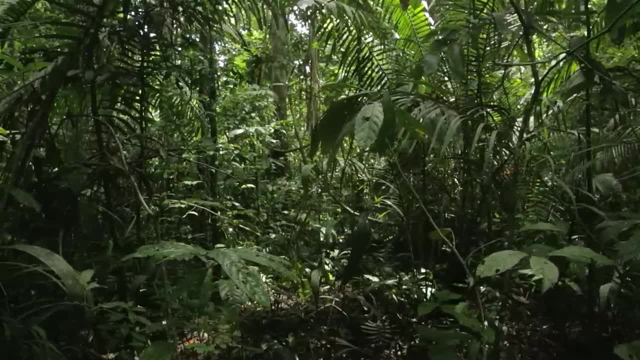 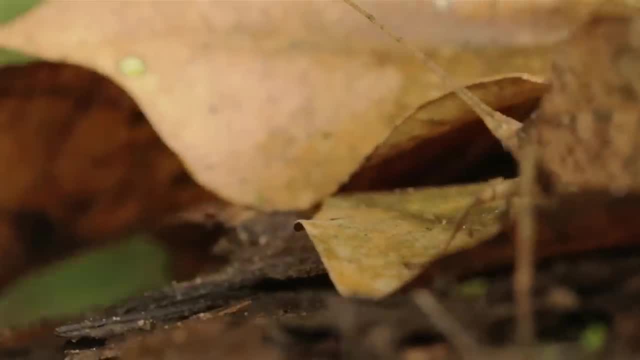 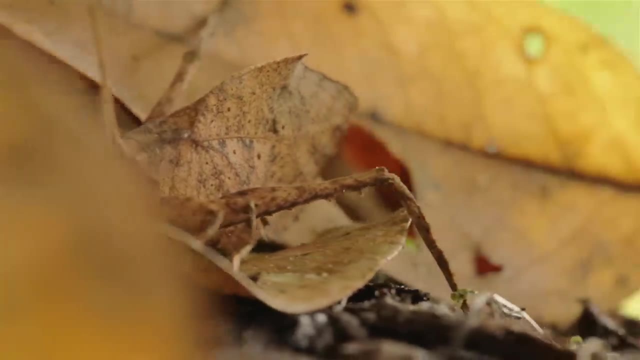 But not all animals avoid predation by hiding away in those hard-to-reach places. Many hide in plain sight. At this scale, nothing is quite what it seems, But I'm aware that this relates to the organisms themselves. You can tell, and your case may differ by a little. 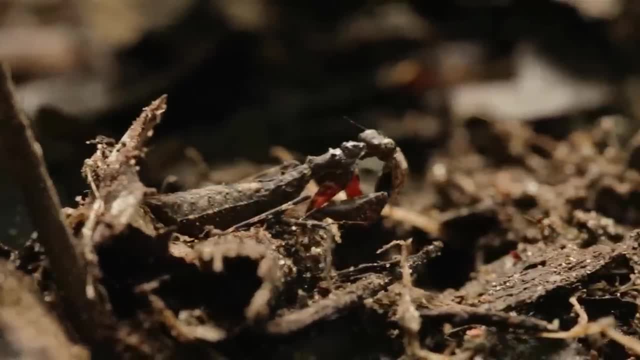 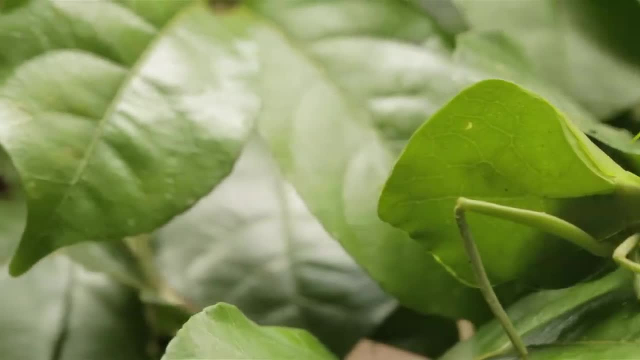 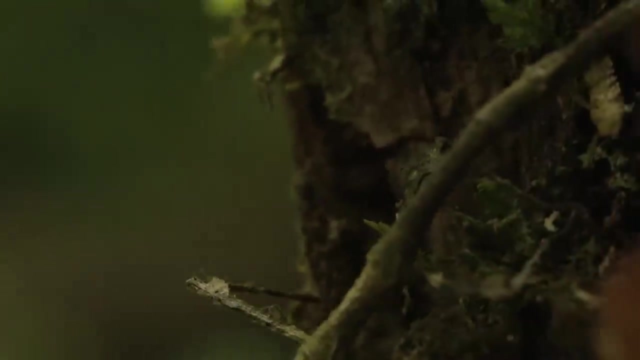 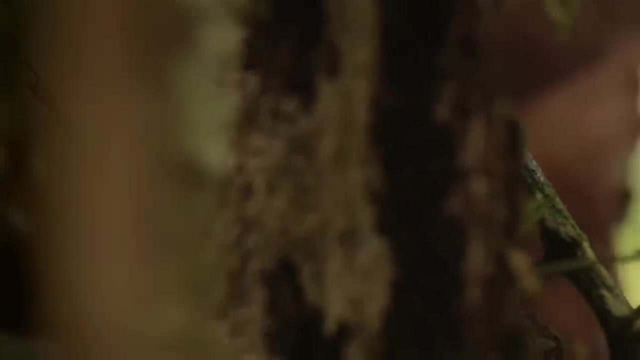 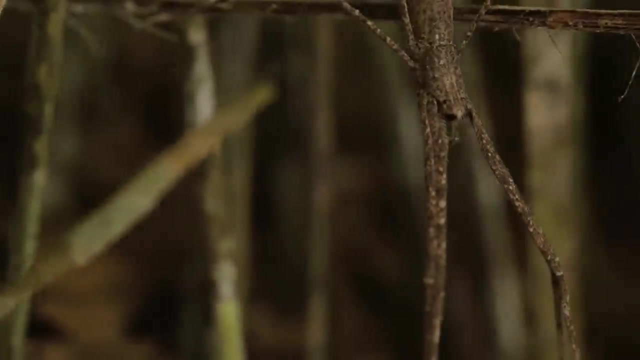 Down to the minute you get stuck on an indoor alloy, the only thing stuck in being F prophecy Lilies. Yeah, Thank you. Some like this arachnid are predators and others will become prey, but all are striving. 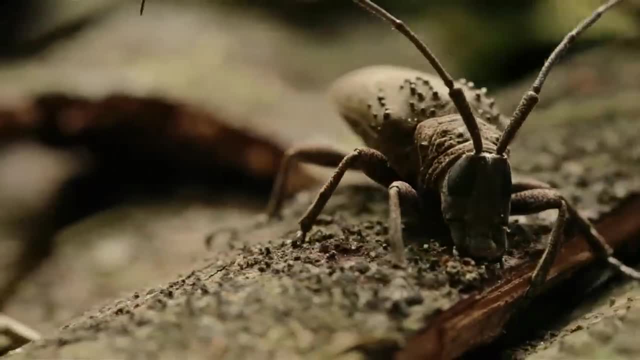 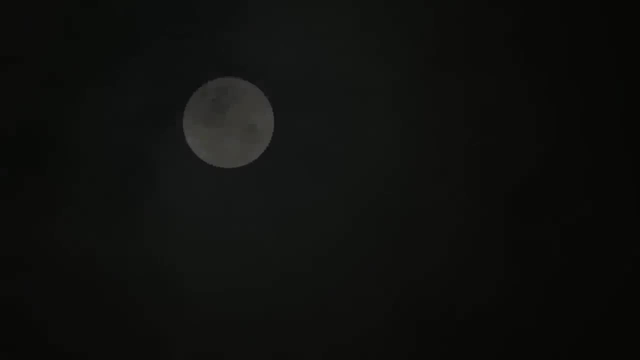 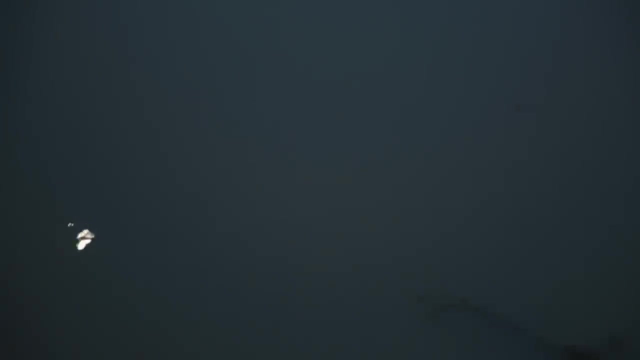 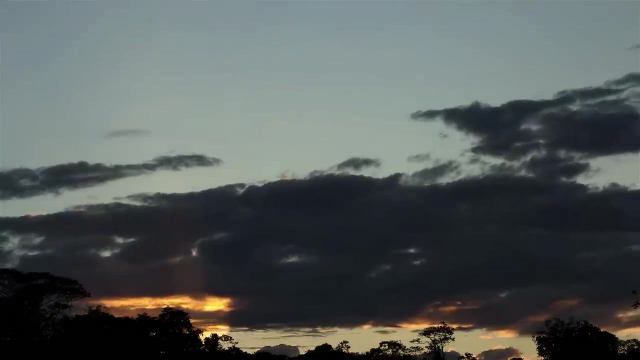 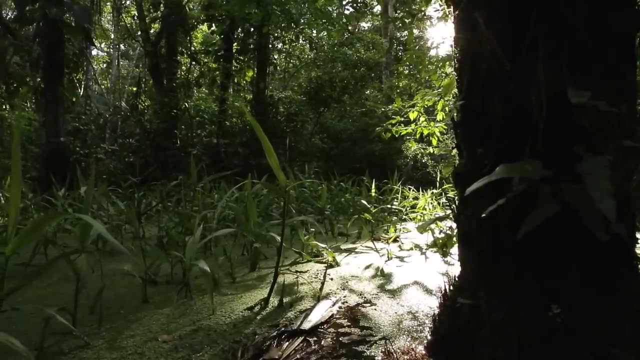 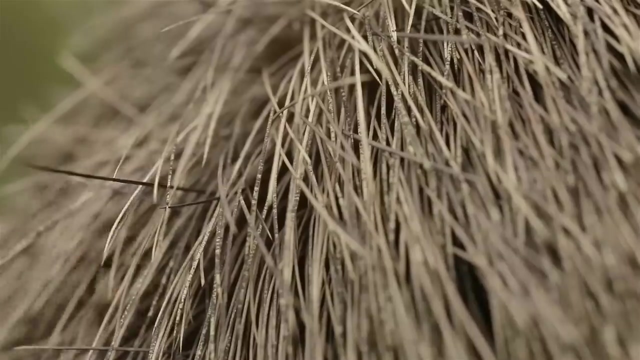 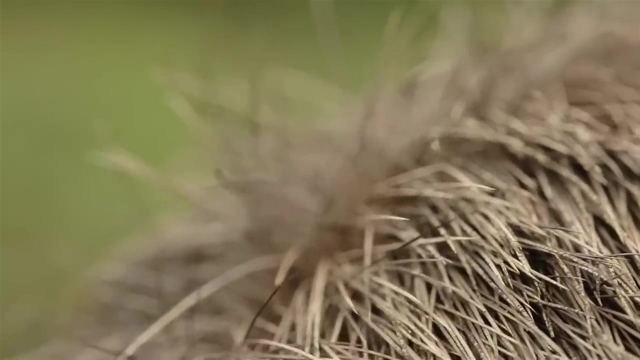 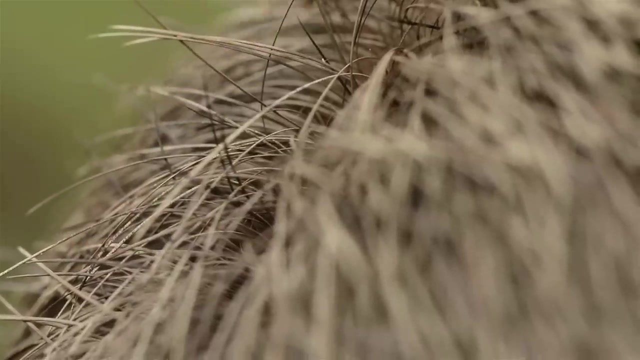 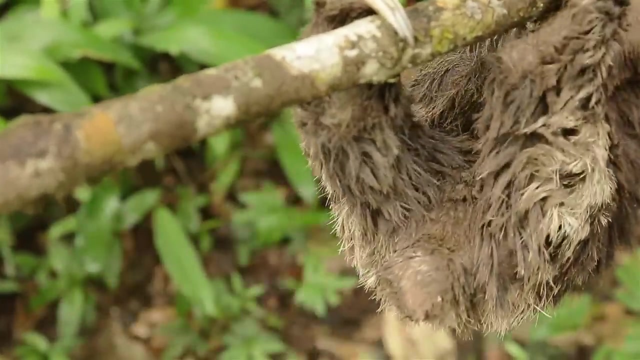 to remain undetected. While many animals avoid predators and catch prey by copying the designs of others, these moths have an entirely different strategy. They hide amongst the hairs of sloths and can't be found anywhere else. The sloth's dense hair supports a variety of algae that help it to blend in with the 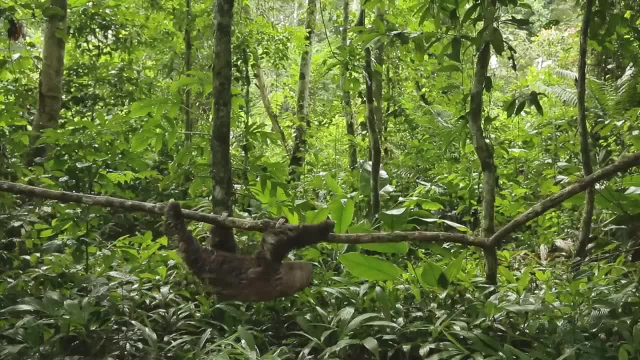 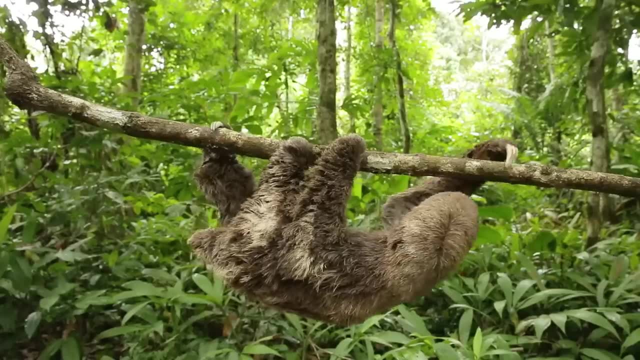 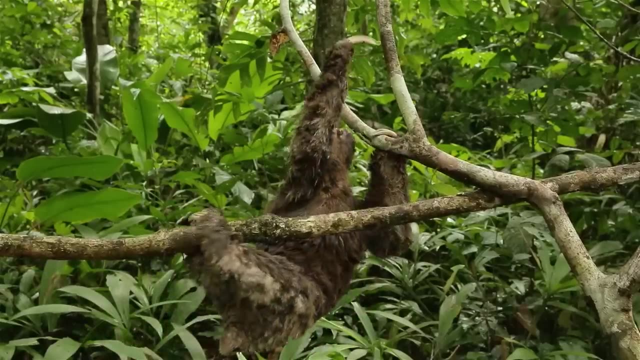 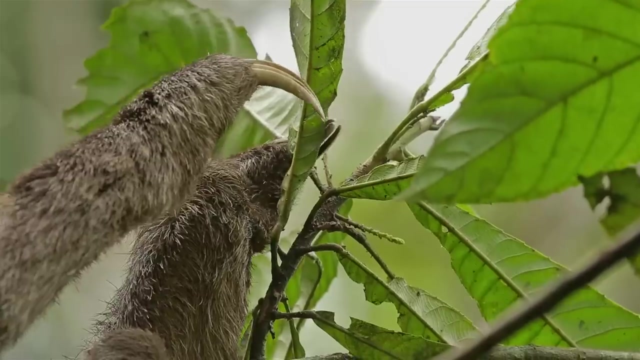 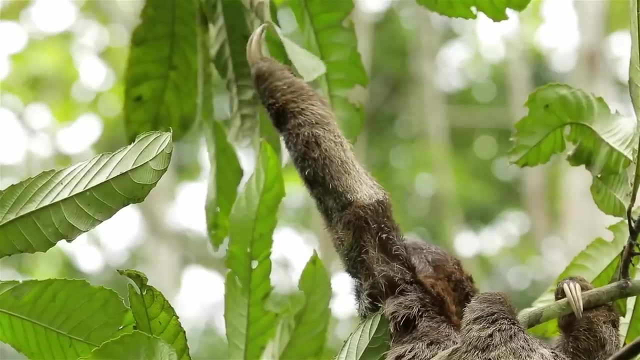 surrounding jungle, And they move so slowly and infrequently that they're rarely spotted by predators. The sloth has a strong sense of smell, so it can smell its prey any time, no matter what the type of species it is and its behaviour. 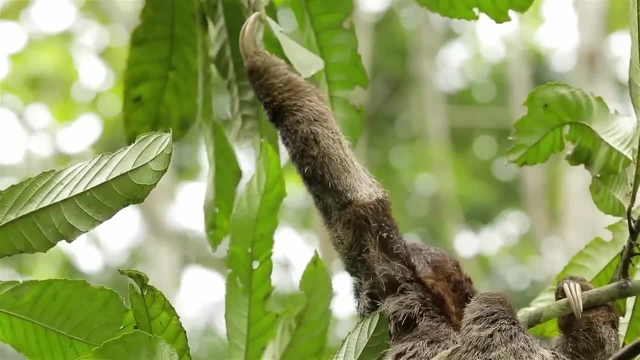 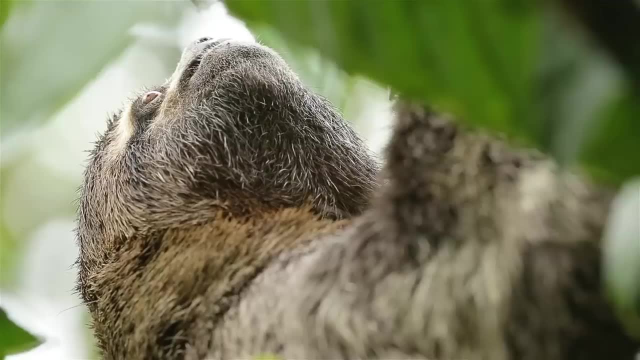 The sloth can't even smell its prey. It can smell its prey when it's on a set of eggs or when it's in a cage. It can smell its prey when it's on an egg too. When it's in a cage, it doesn't taste as good as when it's in a nest. 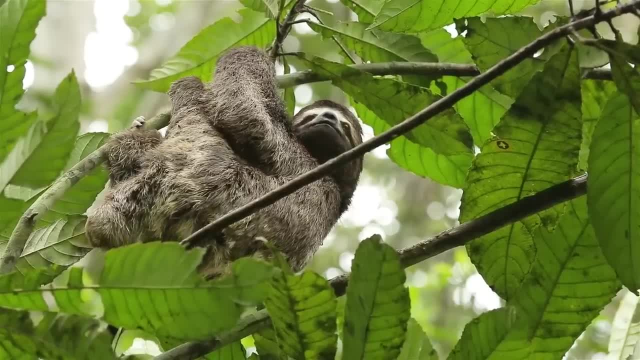 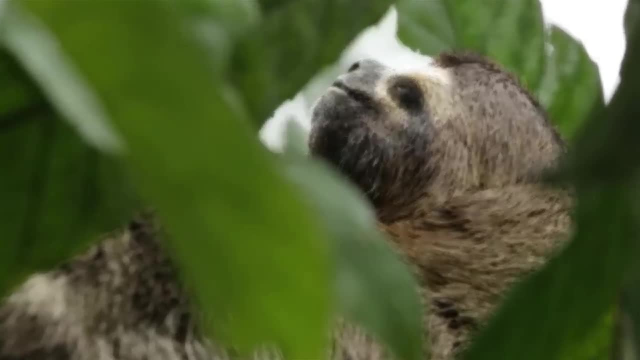 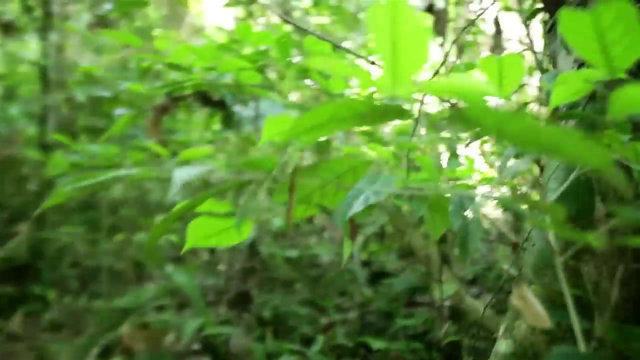 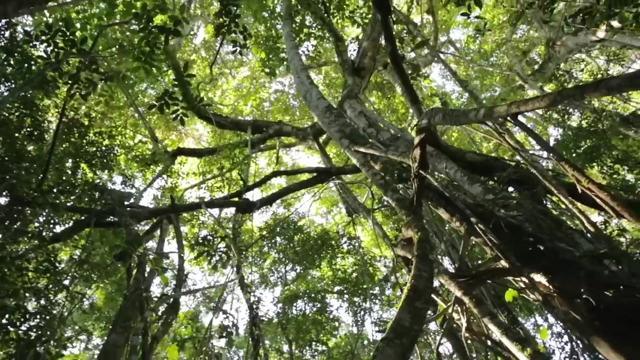 The sloth can't even smell its prey, So this is the only way to stop it. The sloth is a good predator. It's a good predator. It's a good predator. In fact, three-toed sloths spend between 15 and 20 hours of each day fast asleep. 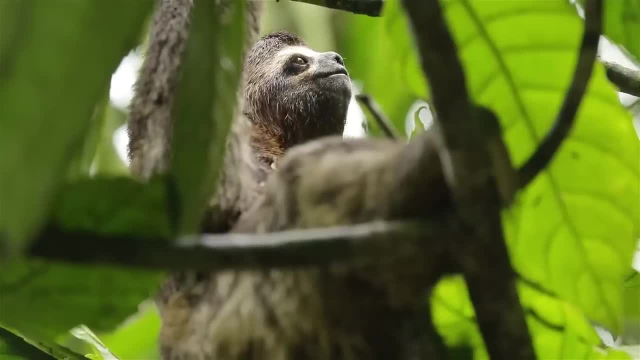 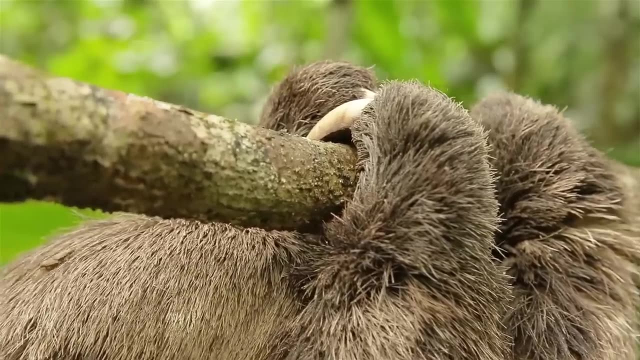 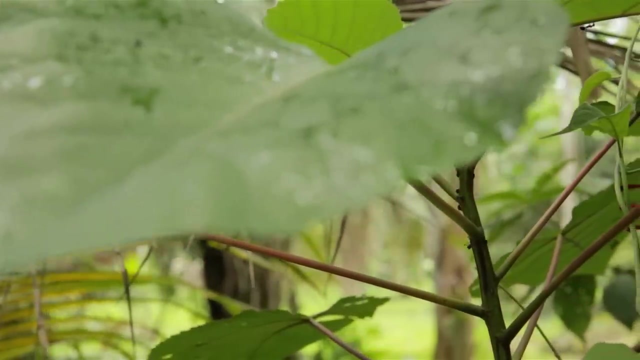 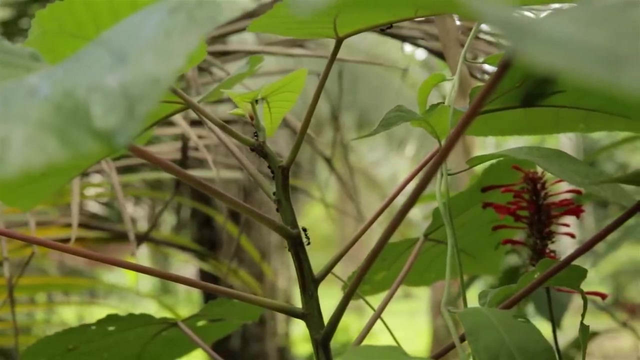 Their leafy diet is simply too poor in calories to keep them going for much longer. The perfect place for moths to make a permanent home. But hiding away and living the solitary life isn't the only way to stay safe in the jungle. Sometimes sticking together can work just as well. 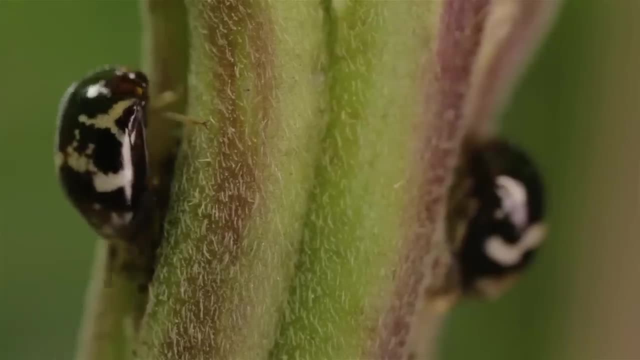 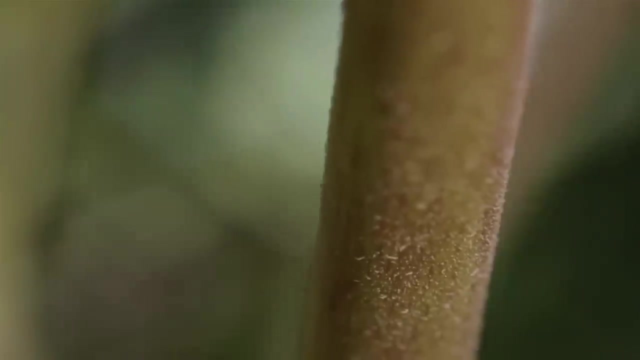 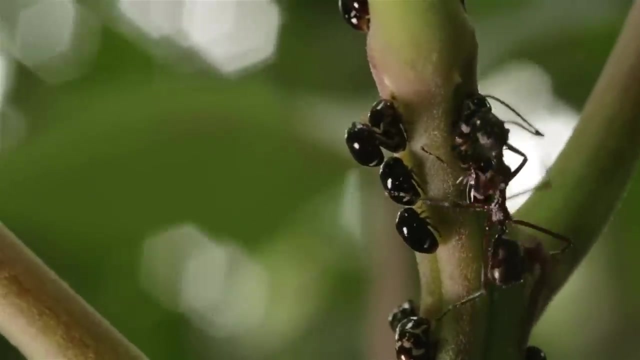 The tip of this young tree is just soft enough for the probing mouth parts of these tree hoppers to break through And feed on the sap that runs through its veins. Aside from a thin shell, the tree hoppers are completely defenseless For protection. they've forged an unlikely alliance. 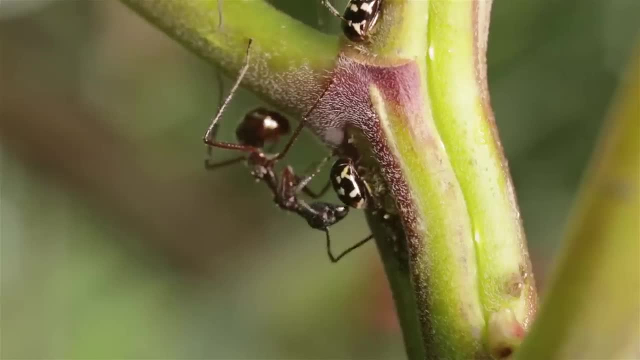 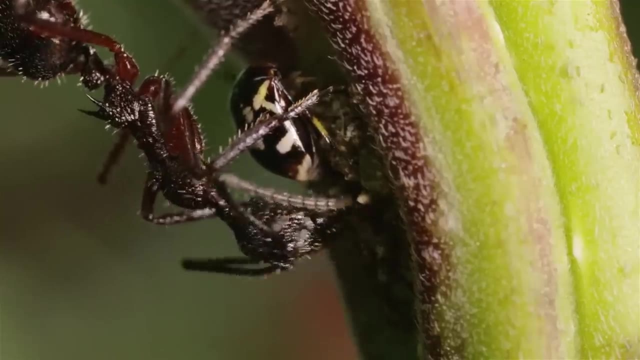 These ants are their defenders and they're paid for their services. Luckily for the tree hoppers, their honeydew or sugary excrement is a sufficient reward. The ants keep the tree hoppers free of mites with specialized cleaning mouth parts. 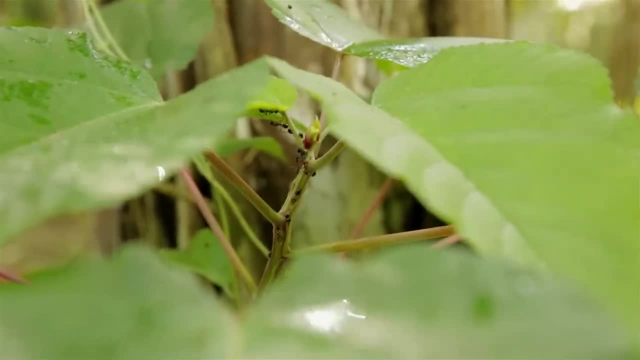 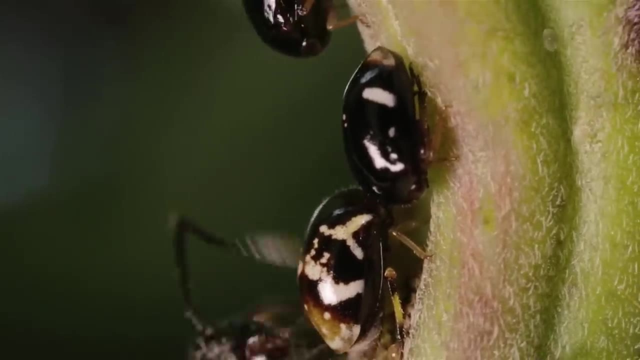 But in THIS jungle there's always a little more happening than first meets the eye. There are actually 2 kinds of tree hoppers here, and one is up to no good. Those with darker shells rarely produce the liquid that feeds their ant protectors, and 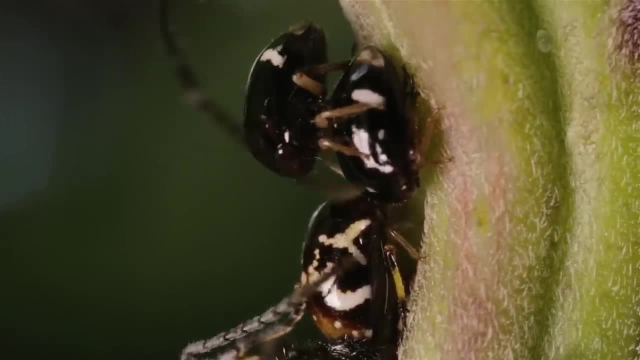 are more resistant to poison than the trunkaze ant��. The anteoliatae are transformable insects and can't be directly infected with insects. they nordic bees are also very tendrilous, But they want to stay clean all the same. 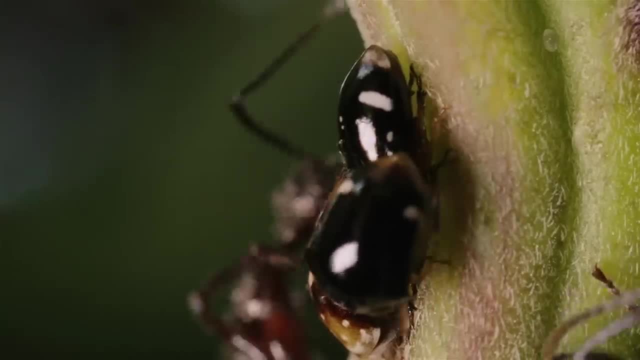 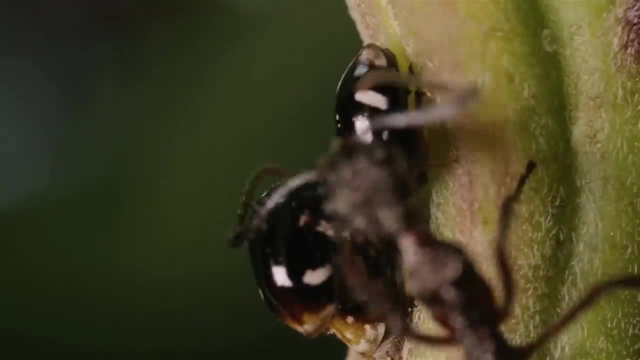 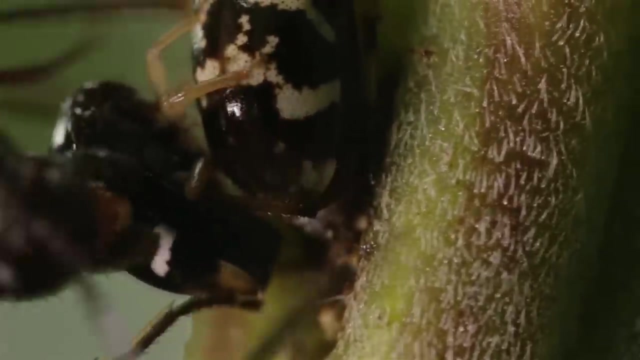 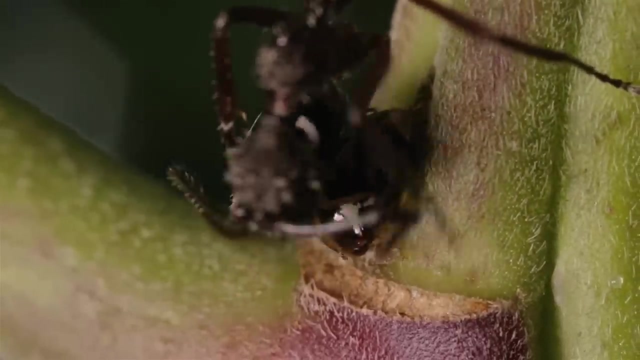 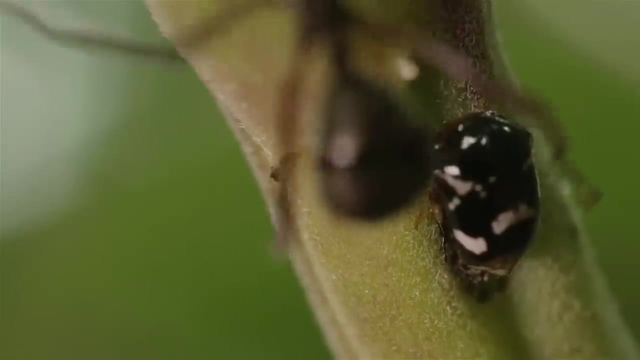 So when they detect an ant ready to clean a lighter colored tree hopper, they simply climb on top and prevent the ant from feeding until they're clean. But they're not the only ones up to no good, Smaller ant species that can't offer the tree hoppers any services in return. 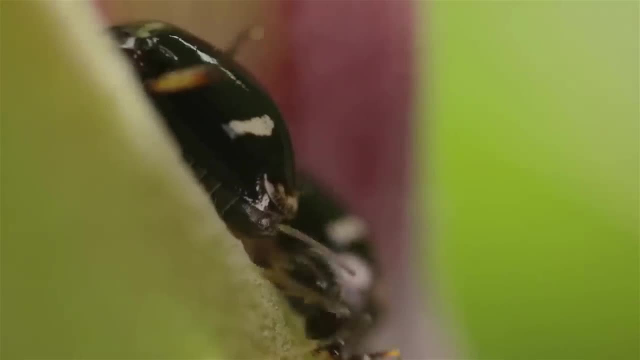 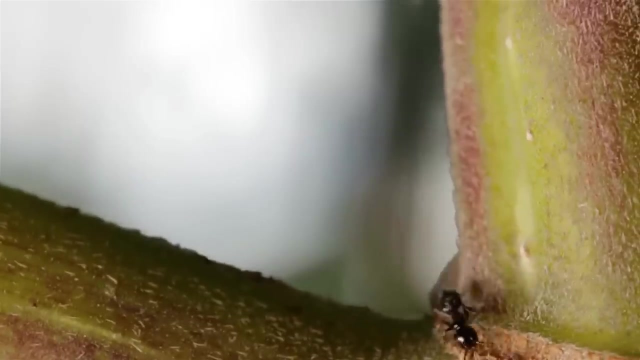 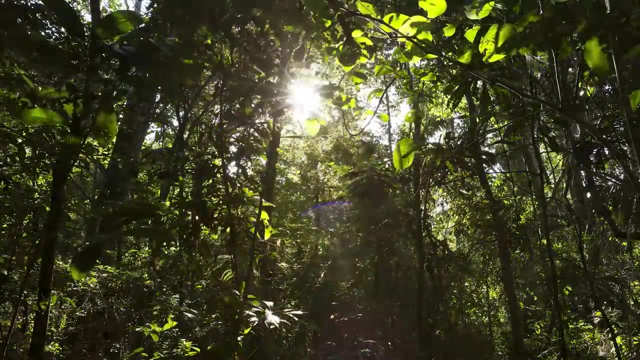 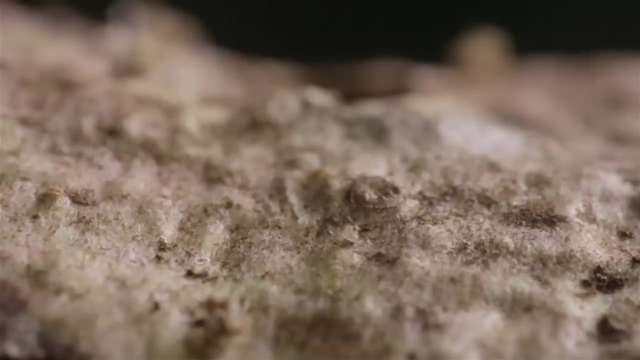 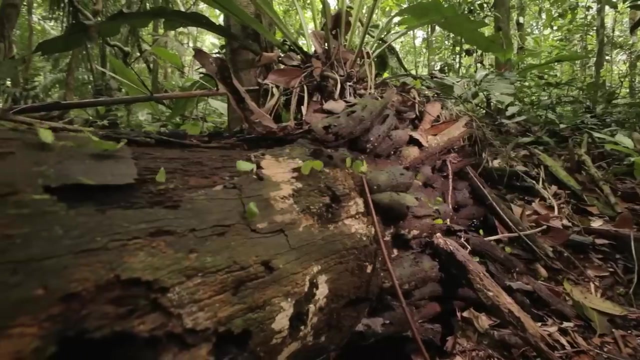 are on the lookout for an unguarded tree hopper and an easy meal. Music, Music, Music Music. Each day, billions of these tiny leafcutter ants embark on a journey, migrating through the forest along miniature highways. The daily commute is coordinated through a powerful 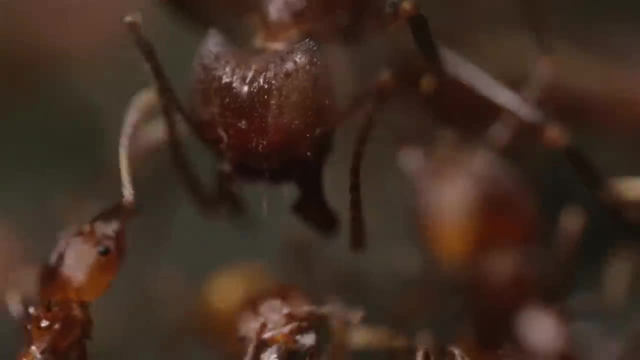 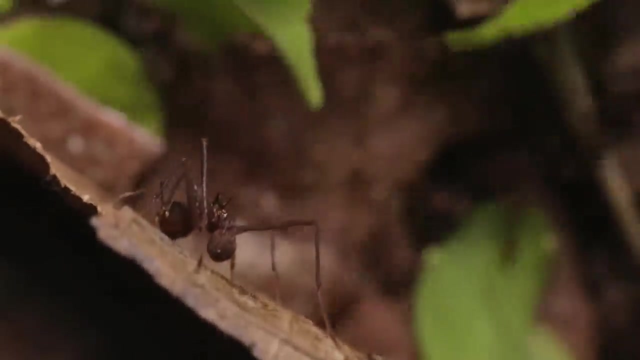 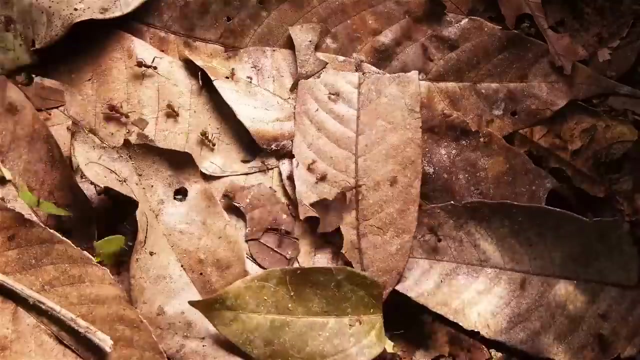 yet invisible chemical messaging system. However, the journey to work can be a hazardous one, and falling leaves often create traffic problems. But these ants are prepared for almost anything. Specialized workers are deployed to remove the blockades. It only takes a handful of ants a few hours to clear a full coating of leaves. 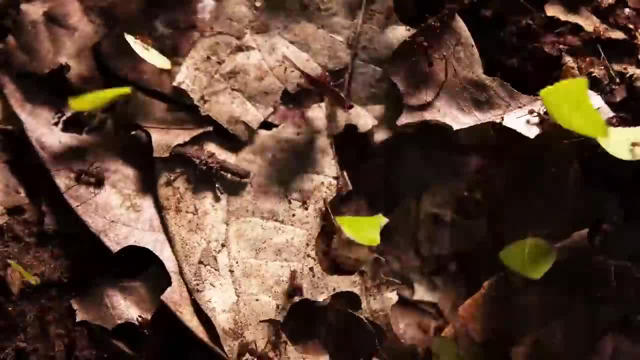 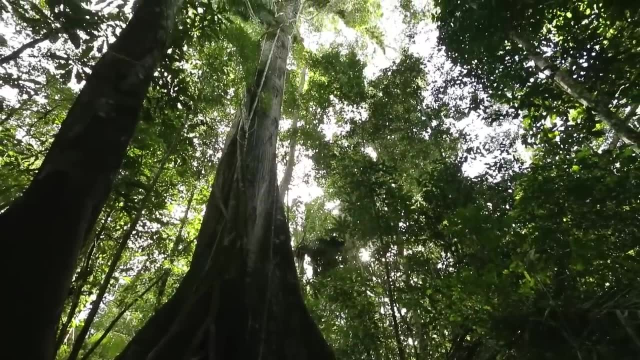 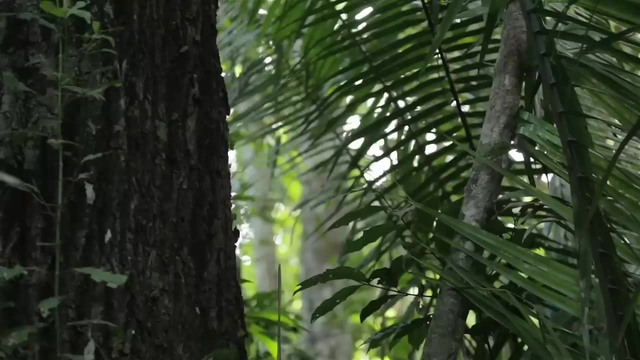 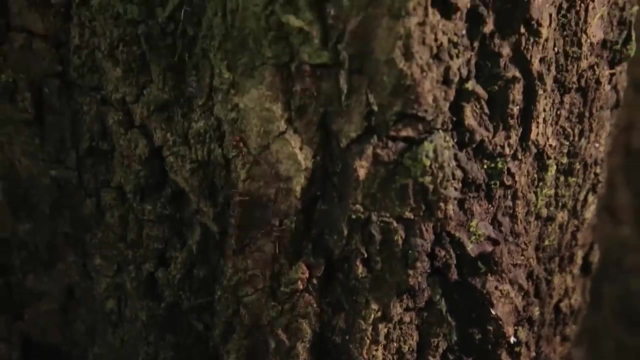 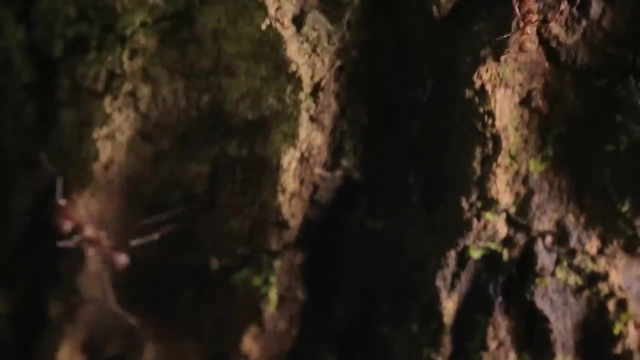 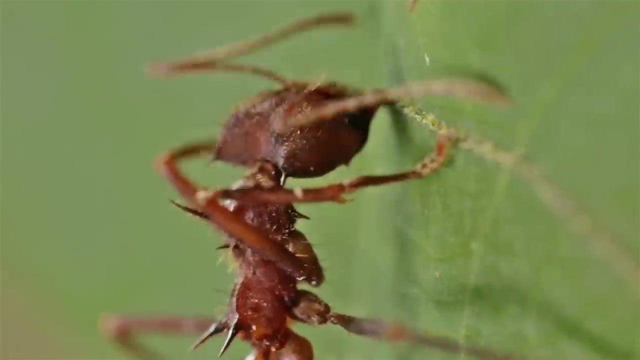 from the forest floor. Music, Music. The workers are all heading for a harvesting tree. They're after its leaves, but to get them they must scale a height comparable to a human scaling the highest mountain in North America. Music, Music. They begin to remove segments from the tree's leaves. 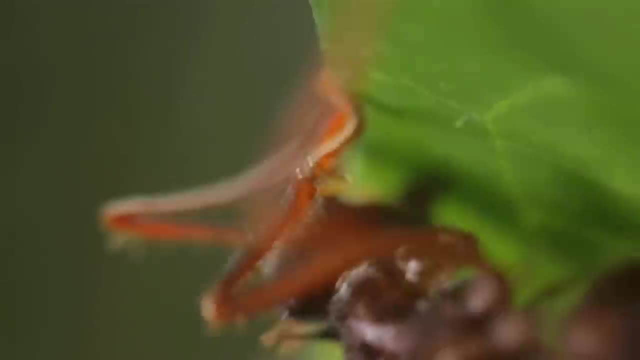 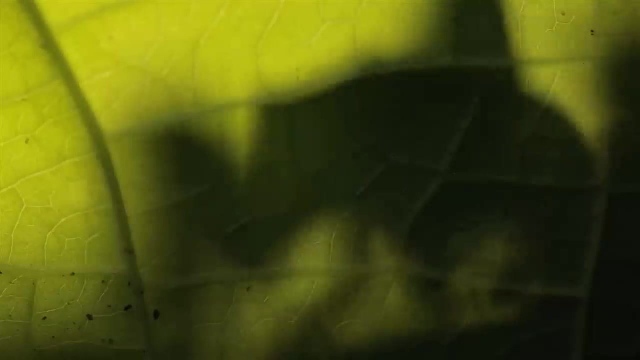 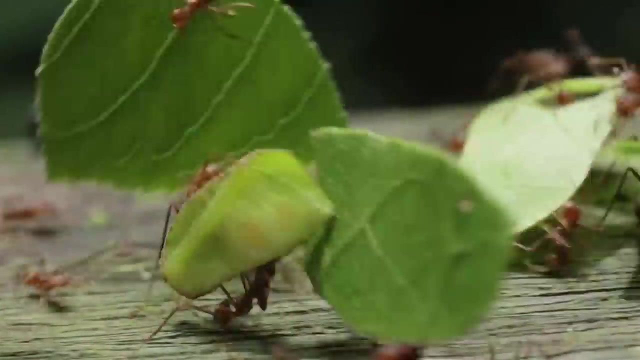 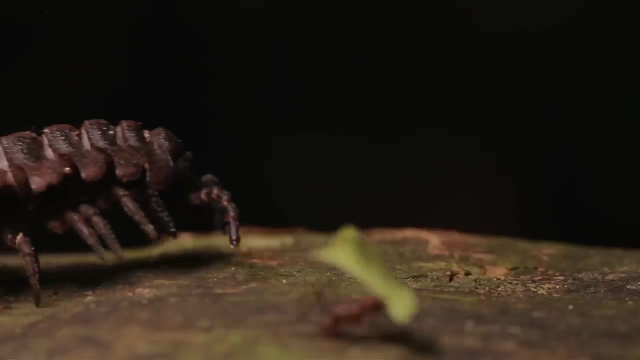 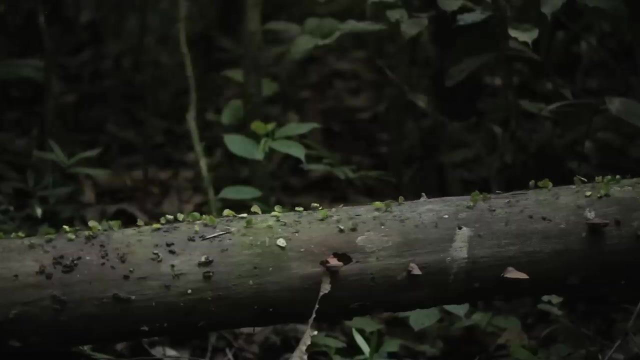 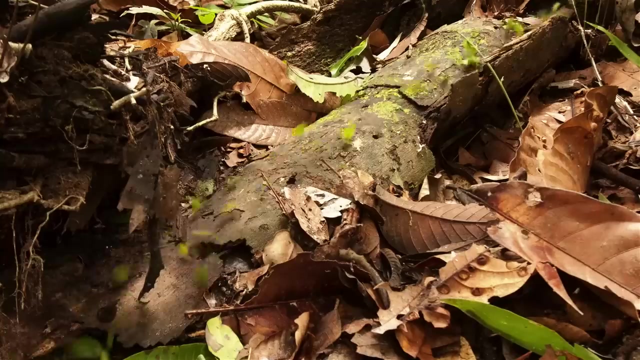 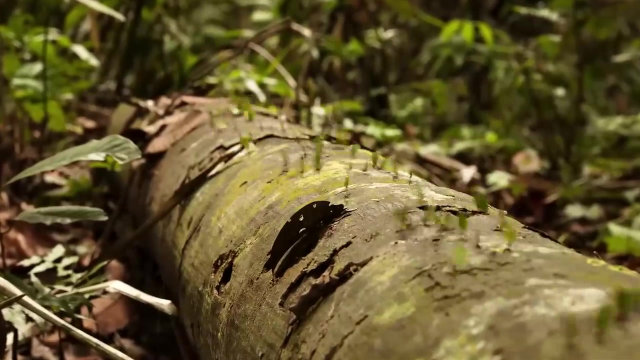 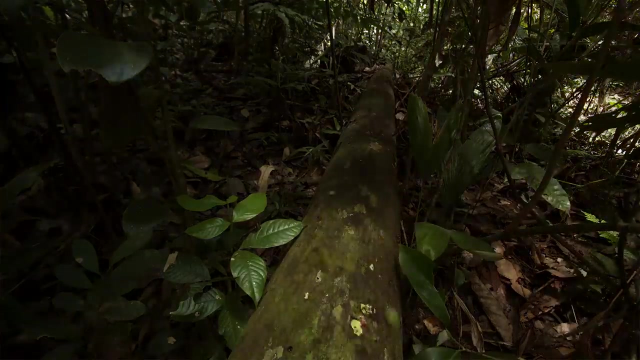 using jaws that vibrate thousands of times per second, Then they must embark on the 100-meter journey back to the nest. Despite the distance, the whole commute only takes each ant about an hour. Efficiency is key, And once the jaws of workers become blunted, 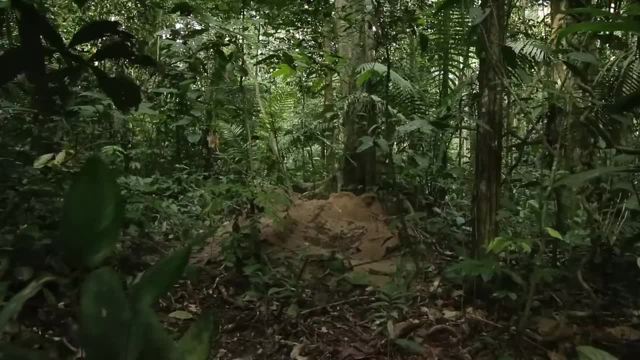 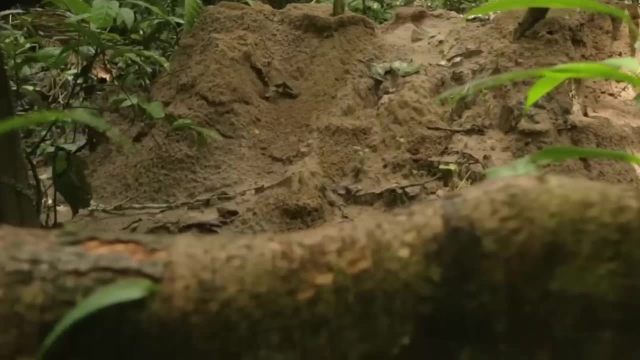 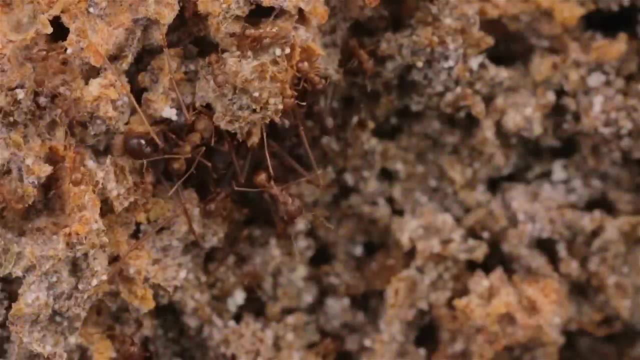 they'll carry the leaves cut by their little sisters instead. At the surface, their home doesn't look like much, But below lies an underground labyrinth of tunnels stretching eight meters beneath the forest floor, home to a colony with as many members as the city of London. 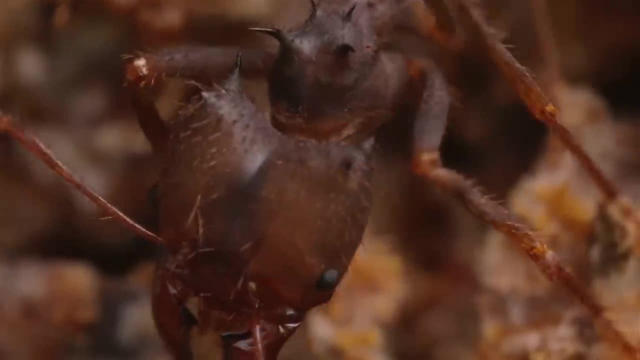 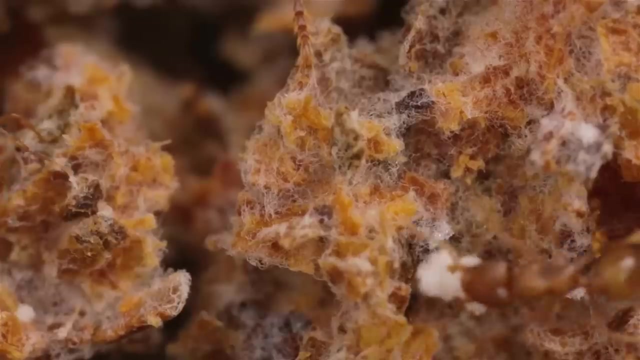 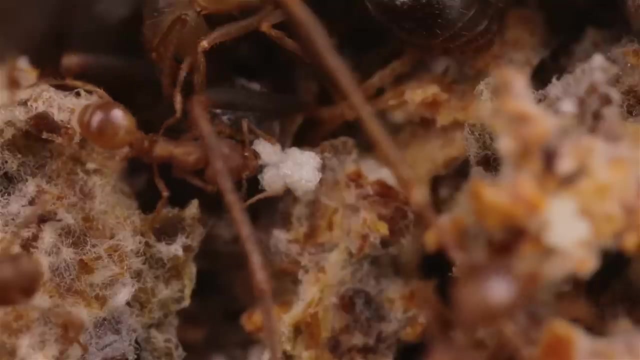 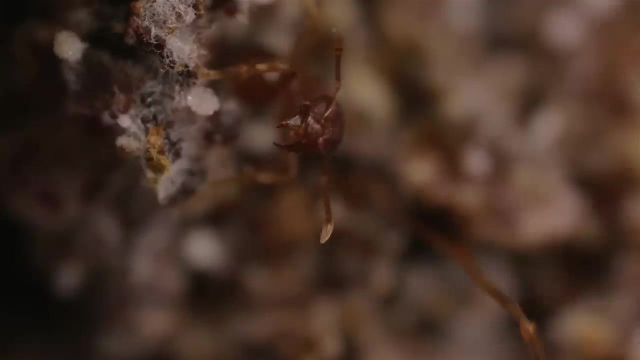 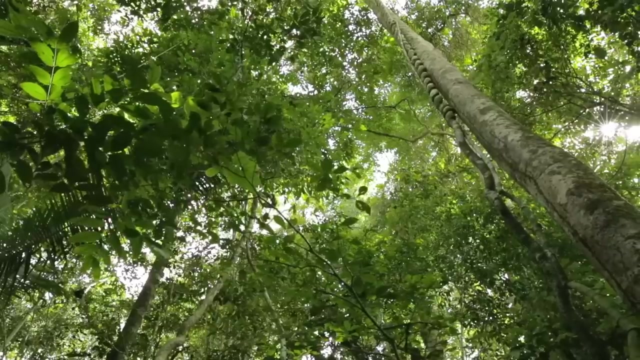 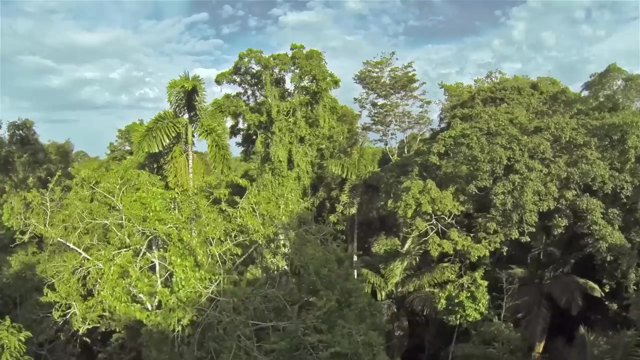 Here in the bowels of the earth, they store their precious leaves and meticulously tend to fungus gardens that sprout from the decomposing vegetation. The tiny white rounded fruiting bodies of the fungus are used to feed the entire colony, Far from the darkness of the forest floor. 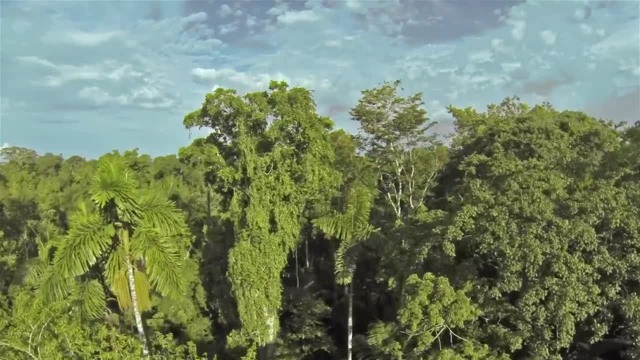 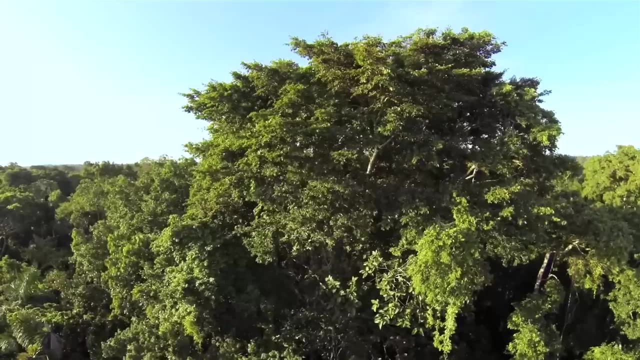 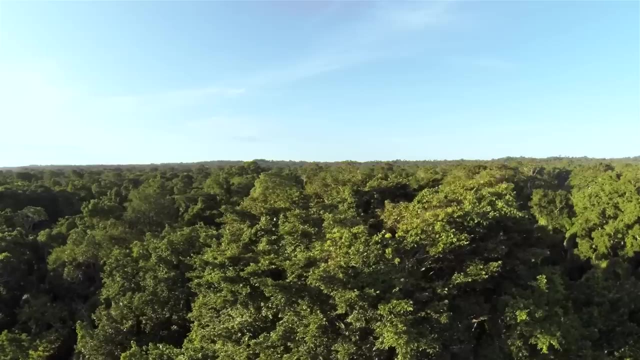 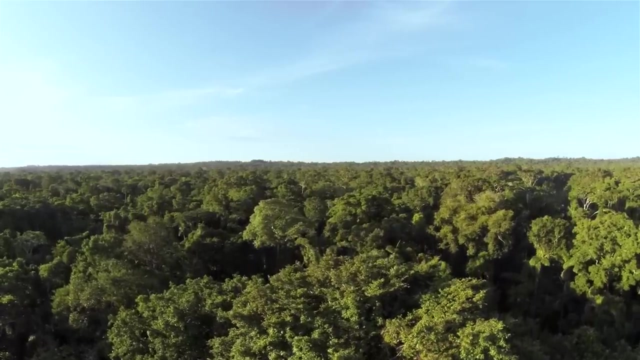 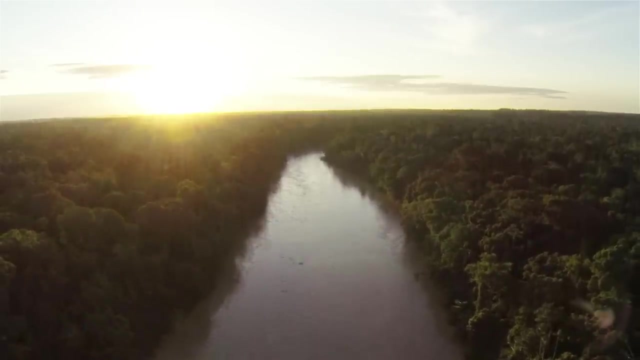 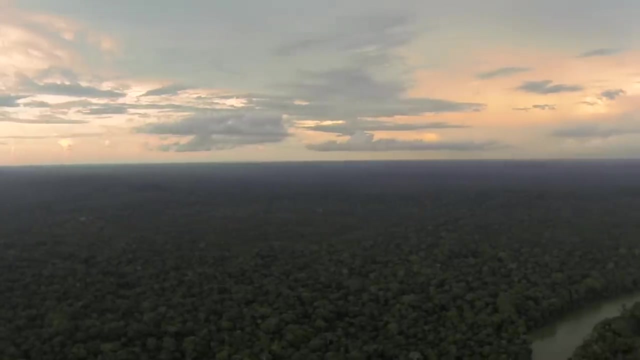 the rainforest canopy is bathed in intense tropical sun. This is the engine room of the jungle, where giant trees capture sunlight to fuel their growth. With a rain, it's the time for the wildflowers to come and play in the open. 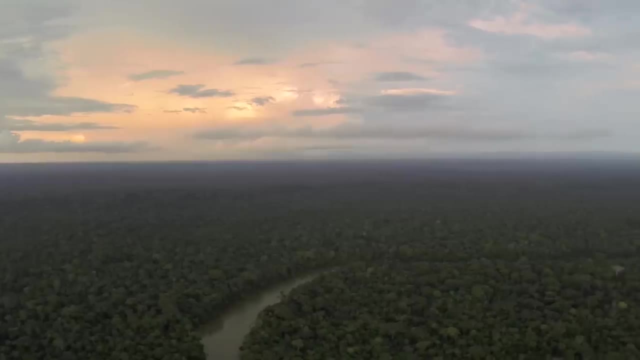 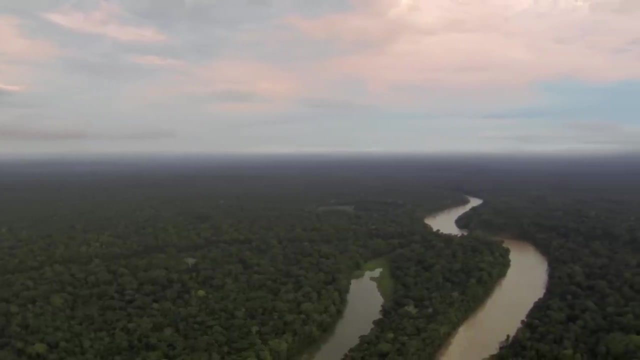 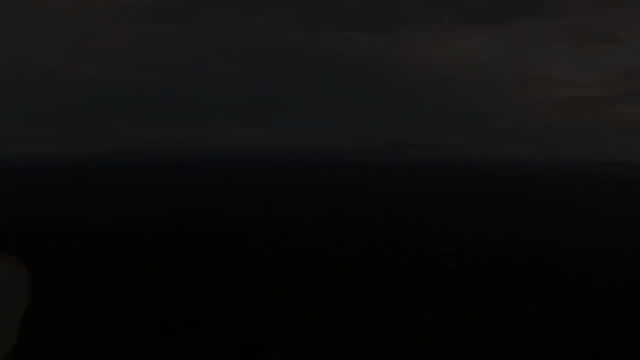 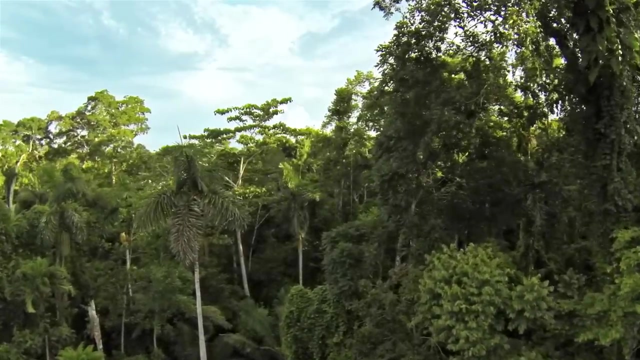 Except for the snaking waters of the Las Piedras River, these rainforest treetops stretch unbroken for hundreds of miles, And this will break the ice miles. Here, in this skyward realm, exists the greatest diversity of life: in the rainforest, and so 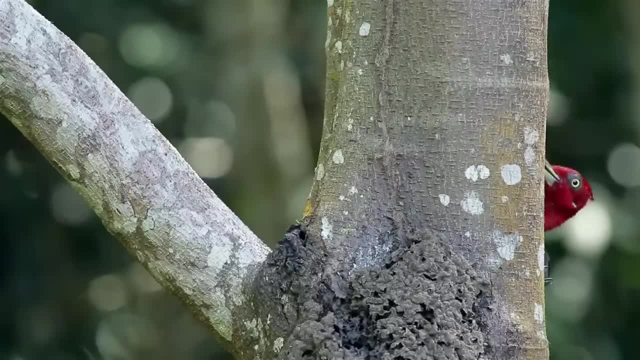 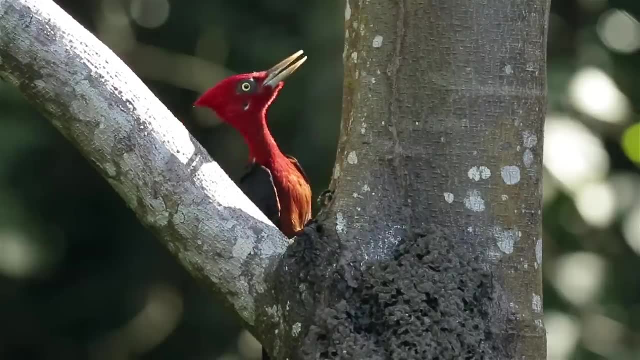 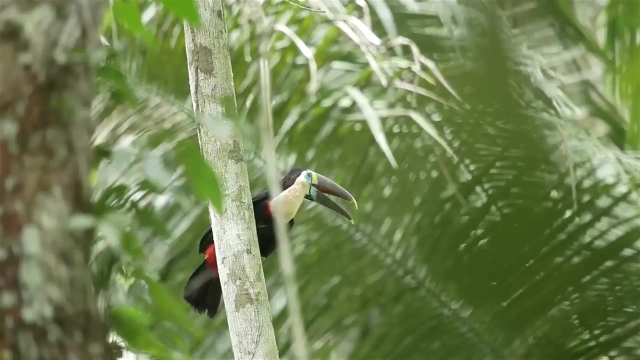 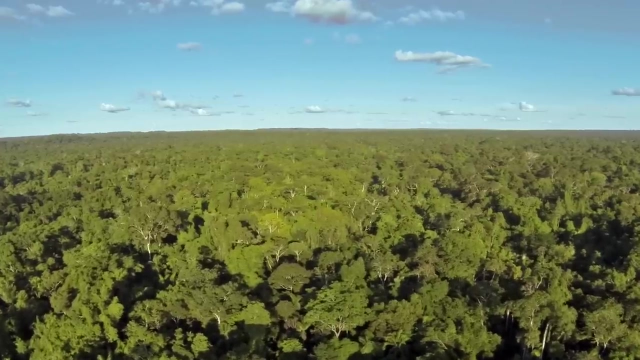 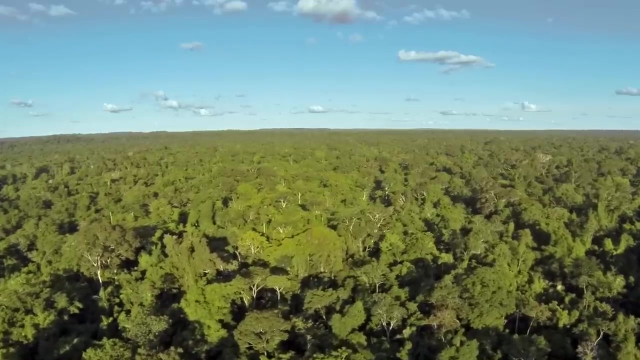 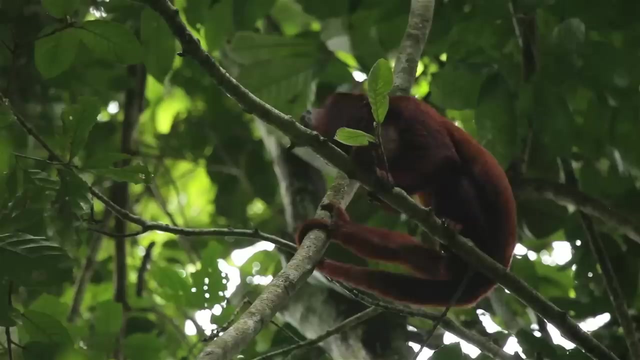 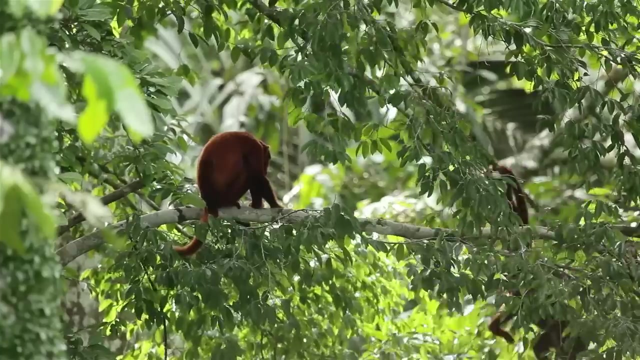 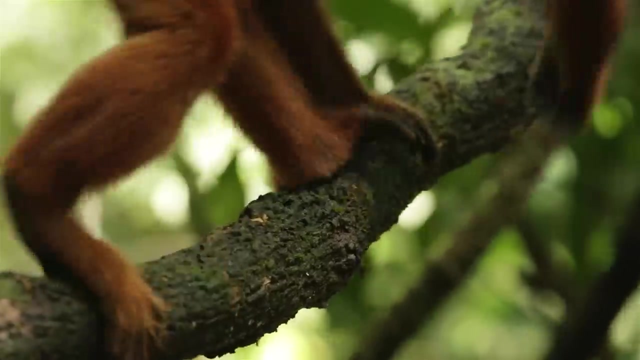 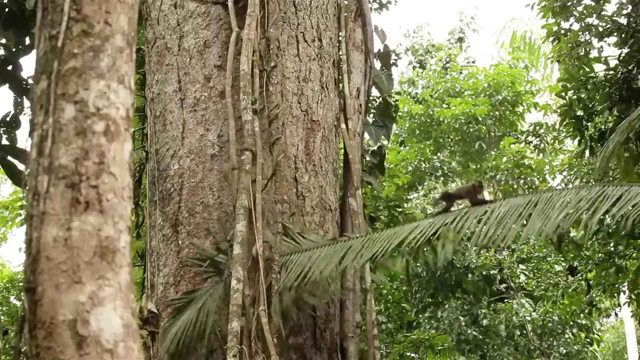 on Earth itself. The calls of red howler monkeys travel from miles across the treetops and stake a group's claim to a small patch of trees where they will socialize and feed on young leaves. Troops of brown capuchin monkeys will range far. 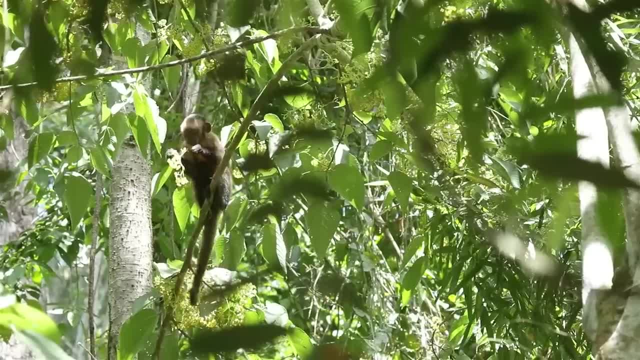 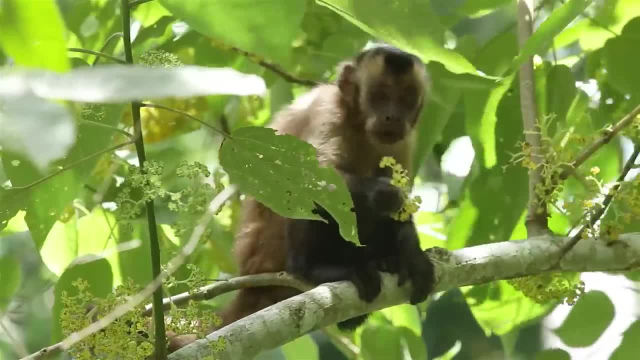 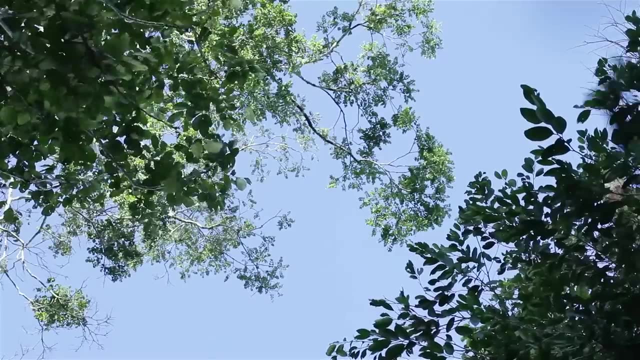 throughout the forest and will eat almost anything they can get their hands on, whether it's flowers, insects, fruit or even small mammals. The capuchins are often tailed by hundreds of smaller squirrel monkeys, who will pick up whatever they leave behind. 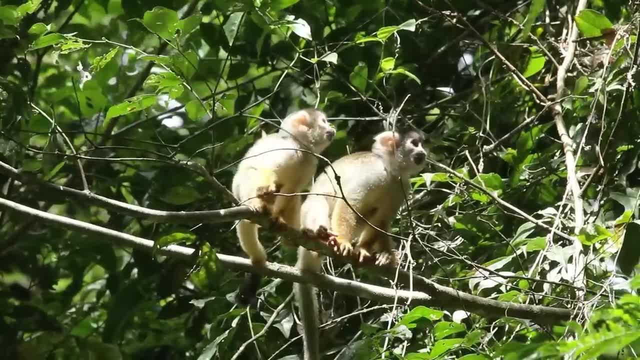 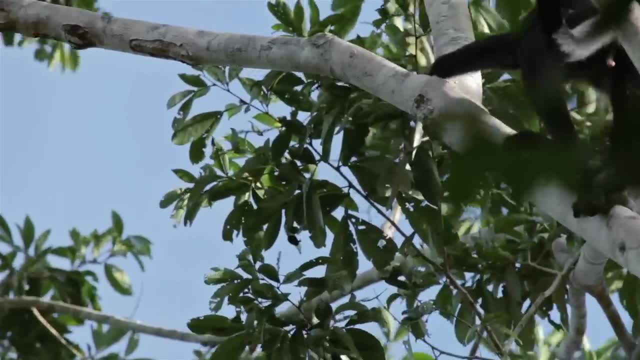 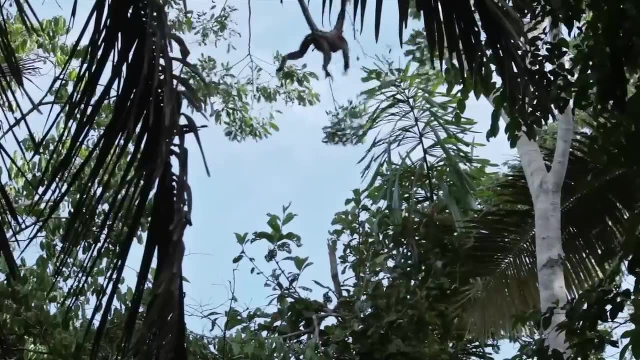 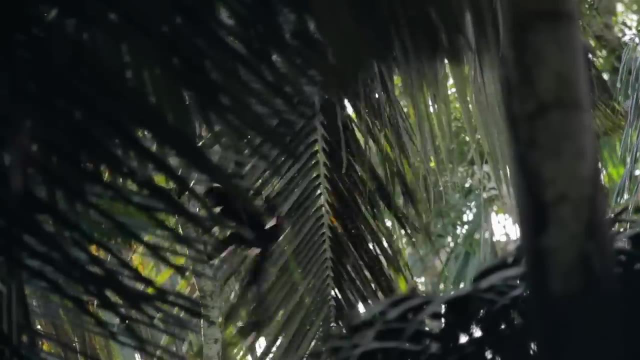 This unlikely alliance was forged to reduce the risk that a single individual will be picked off by an eagle. The largest of the monkeys here are the spider monkeys, and they are constantly on the move. They follow well-trodden routes that track the shortest distance between fruiting trees. 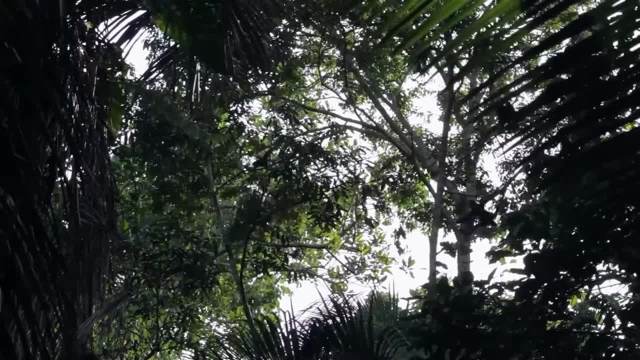 During times of plenty, as many as a hundred individuals can be found traveling together for a short time. The capuchin monkeys are the largest of the monkeys here and they are constantly on the move. When small groups meet, new friends are made and new groups are formed. 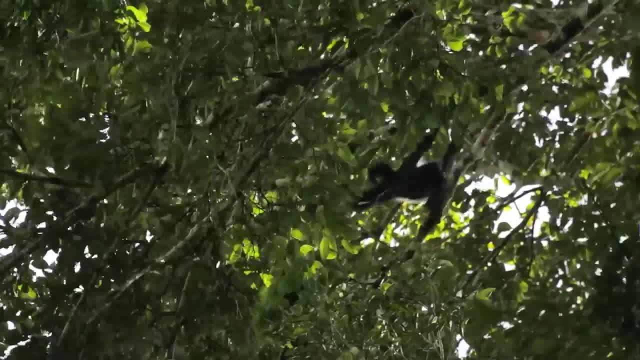 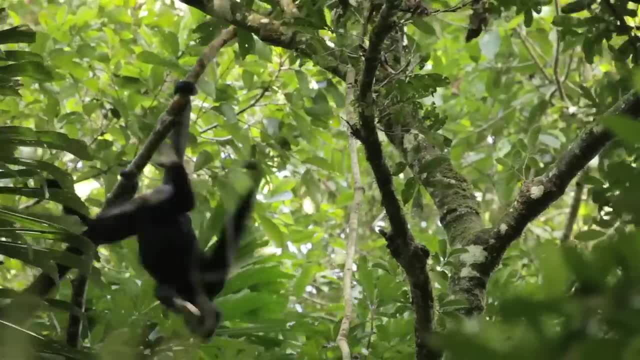 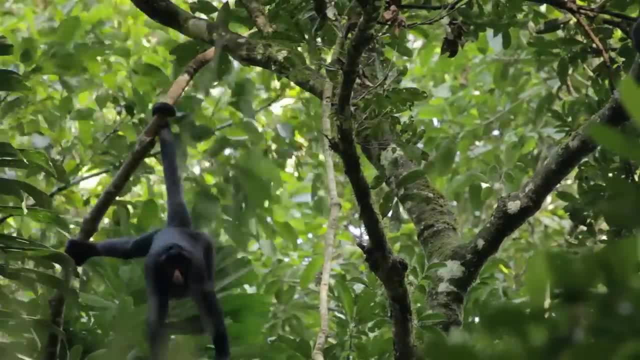 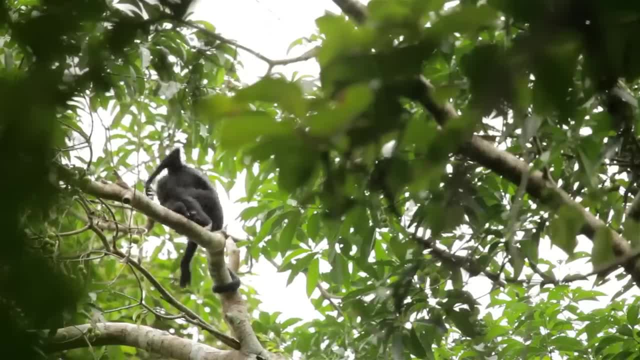 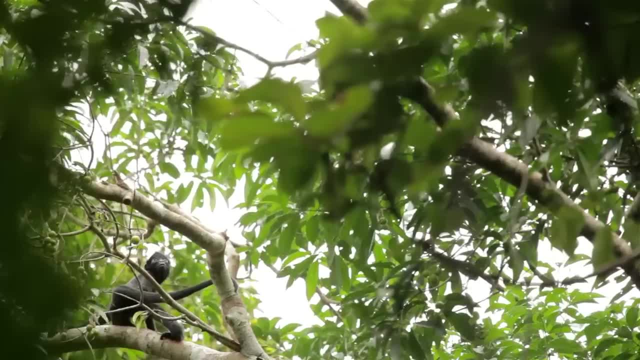 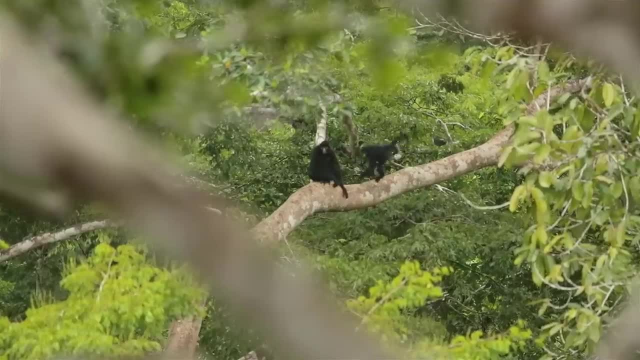 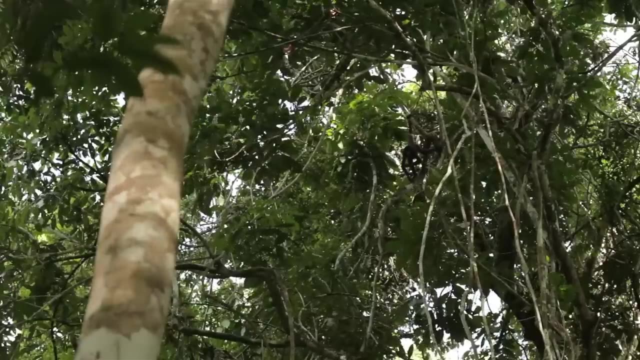 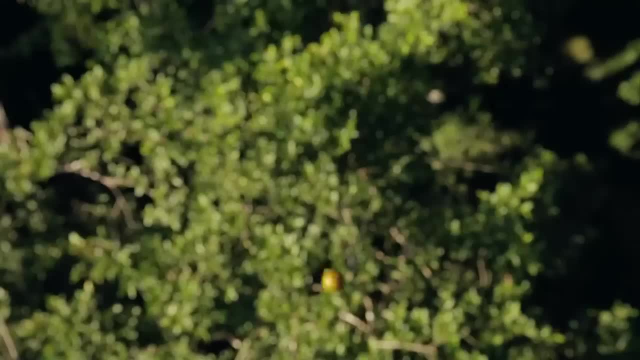 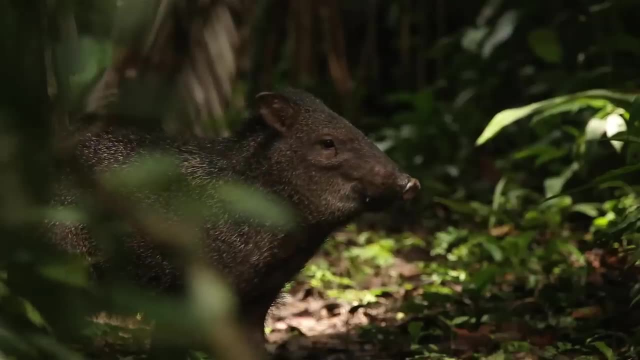 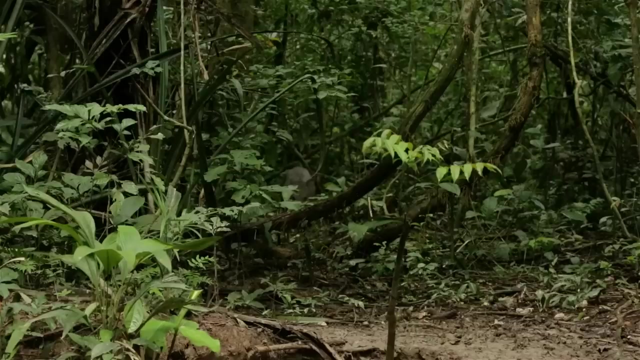 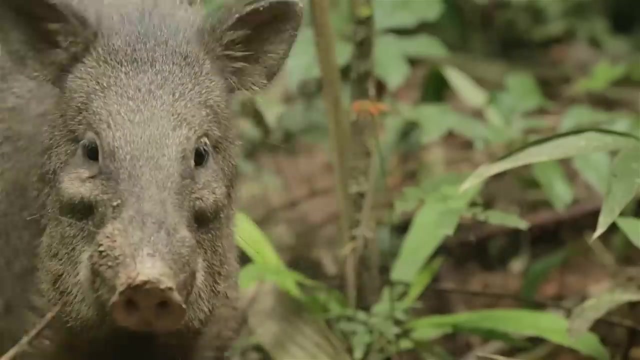 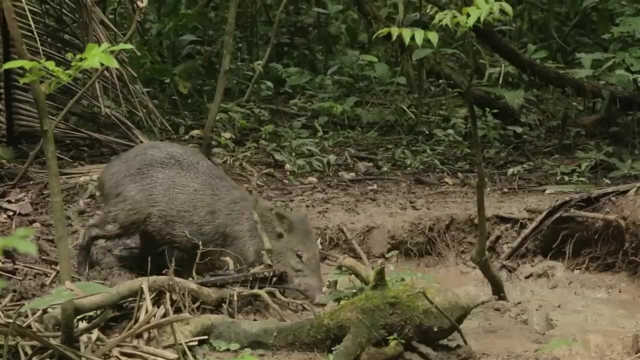 drop the rest, But it rarely goes to waste, as peccaries that roam the forest floor will consume much of what's been dropped To balance off their diet. collard peccaries seek out special places from which to feed. The thick mud in this hole contains unusually high concentrations of salt, a rare treat. 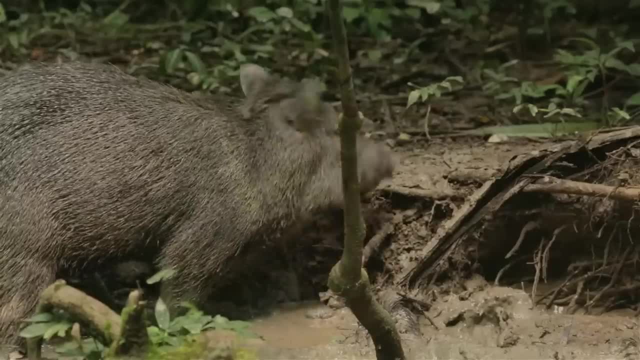 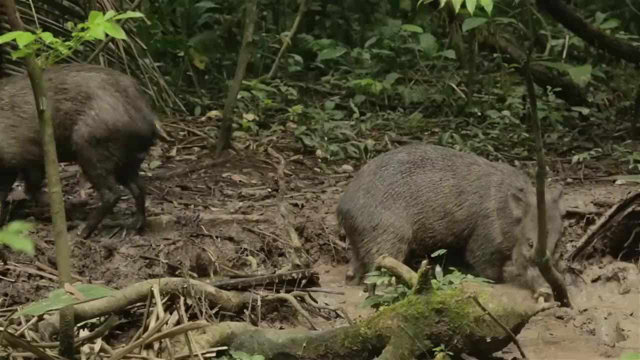 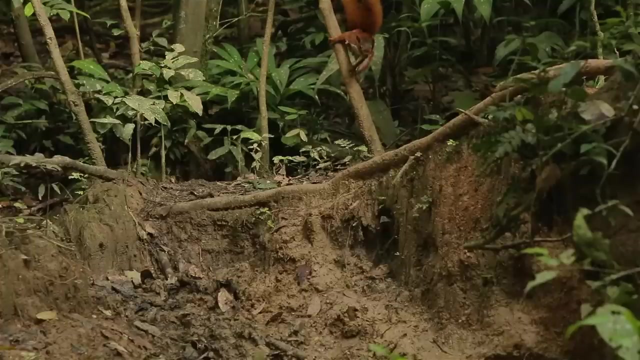 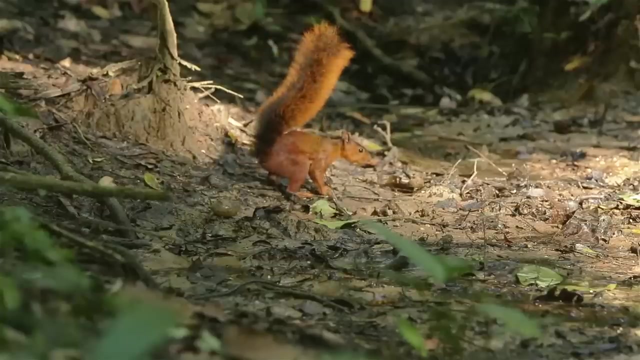 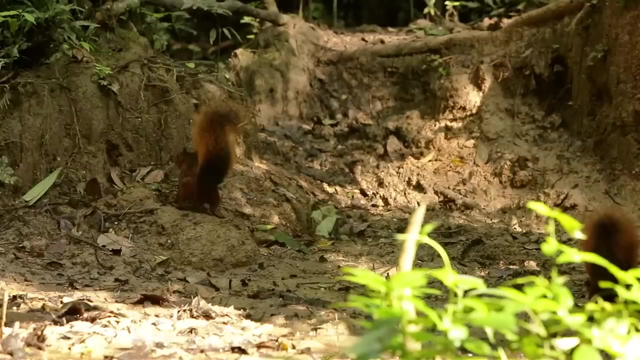 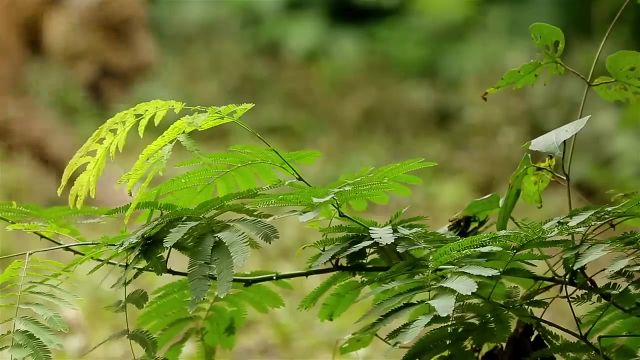 so far from the sea. Small mineral licks like this one are dotted throughout the forest, and for many animals they're like miniature oases in a nutrient-poor desert. Throughout the day, a variety of visitors come and go. Some, like this red brocket deer, are particularly wary as they know that jaguars hunt here. 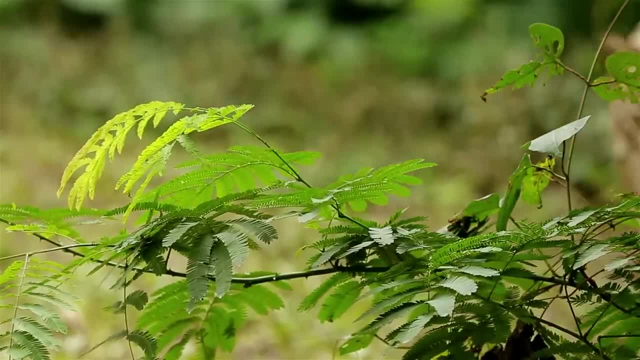 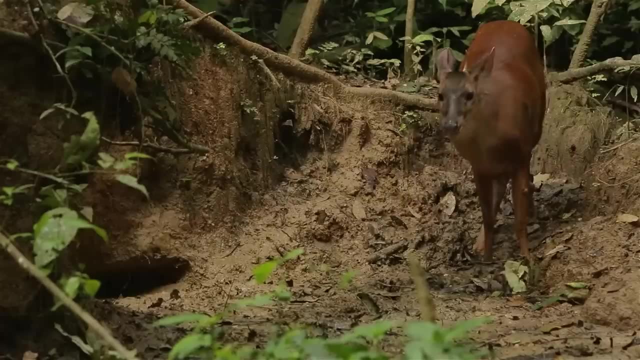 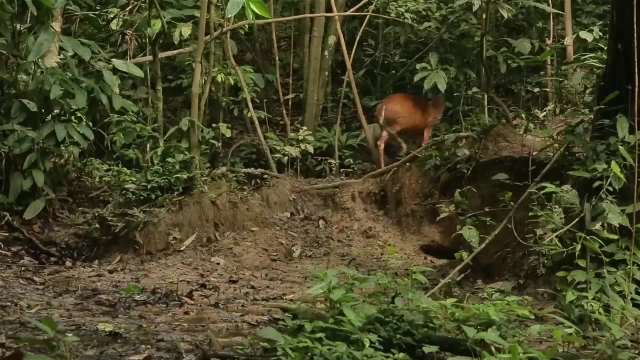 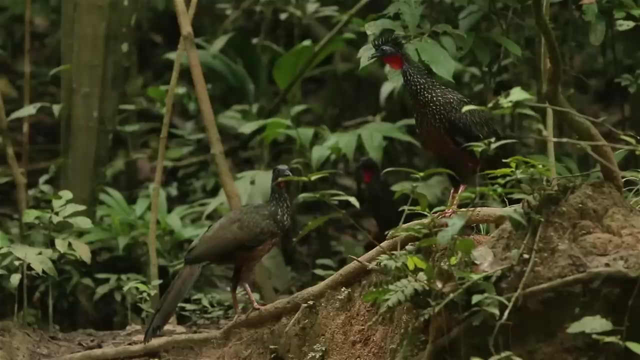 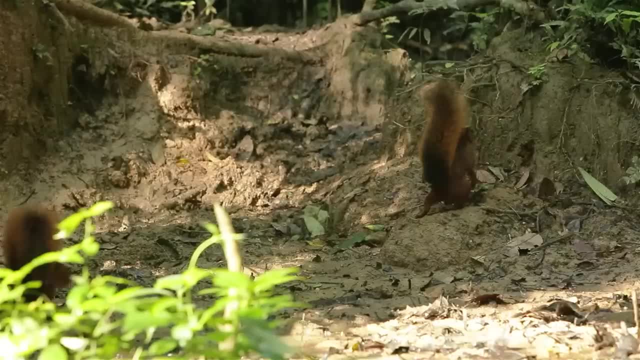 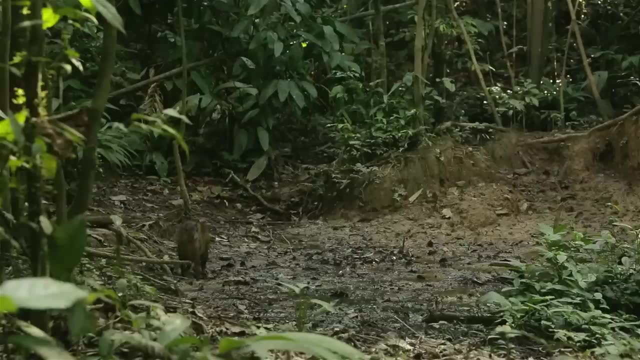 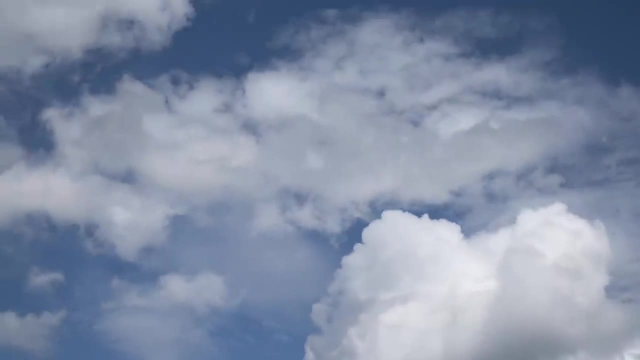 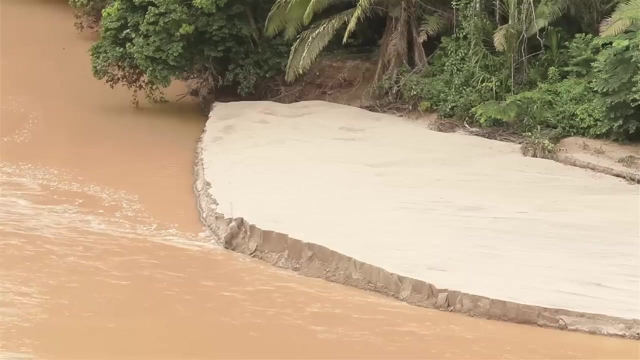 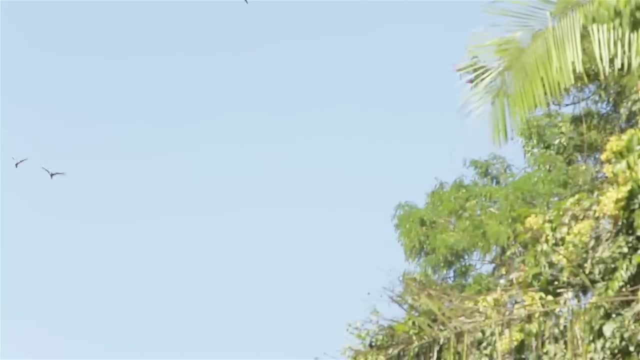 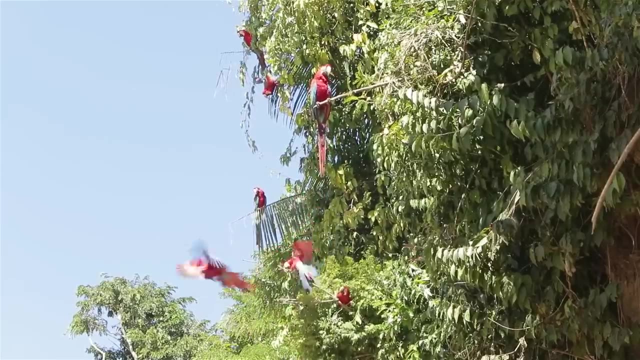 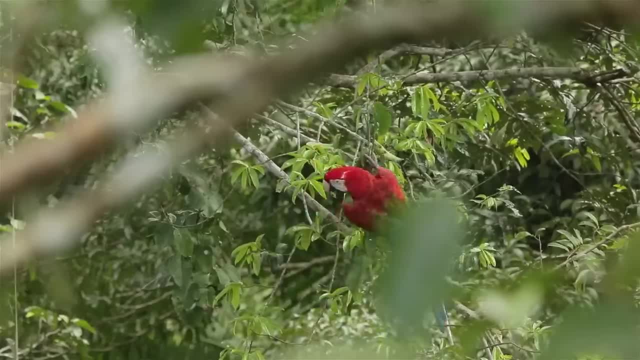 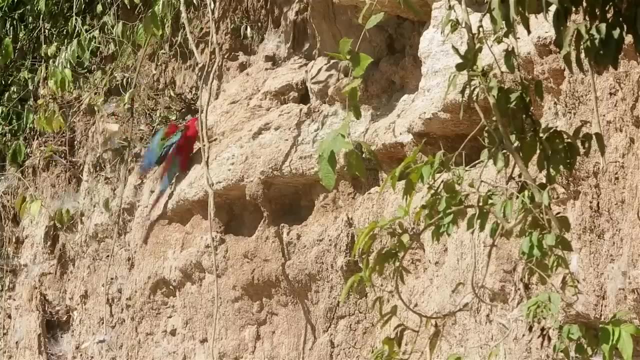 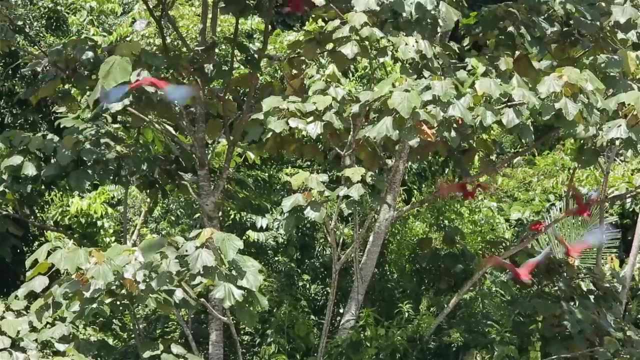 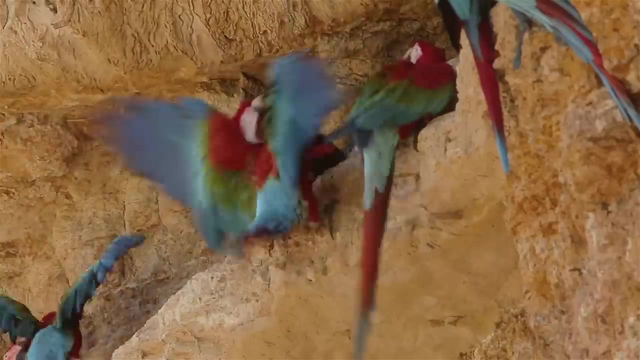 to fly down to the lick and reassure them that the area is free from predators. Once a few make it down safely, the rest decide to follow. Not only does eating the clay provide salt, but it also helps to neutralize the toxic chemicals found. 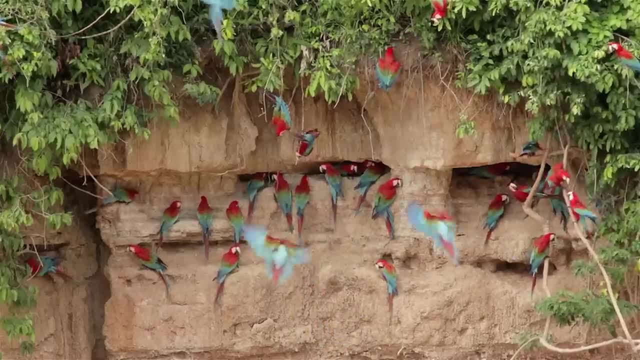 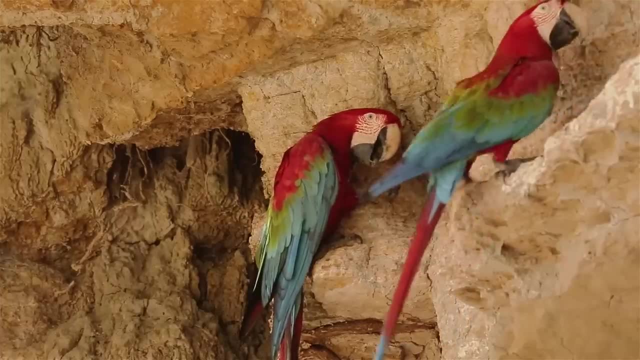 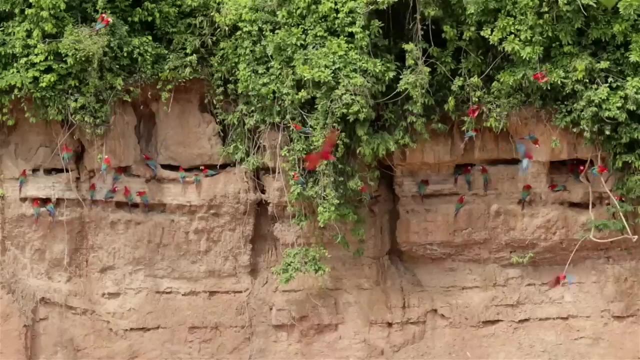 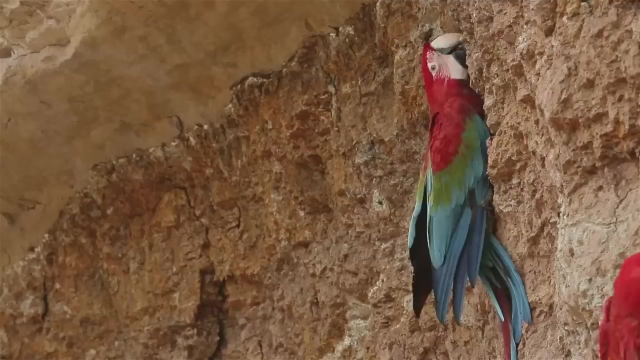 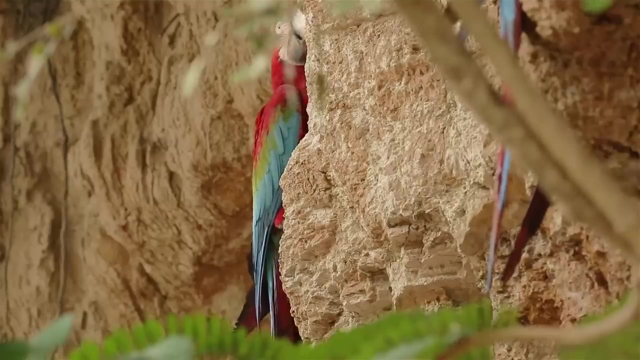 in many of the unripe fruits in the Macaw diet. For the Macaws, these visits to the local clay lick are more than just feeding opportunities. They're places where mates can be found and disputes can be settled- A couple who actually enjoy their time at the lake. 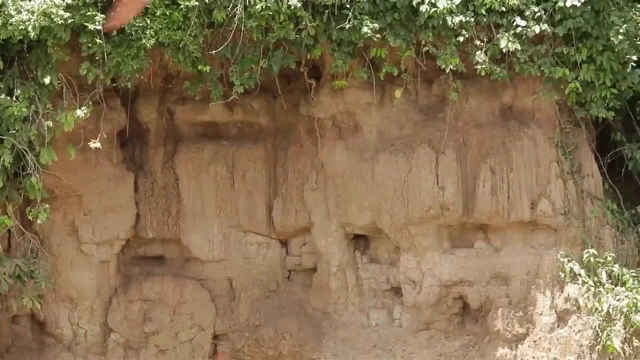 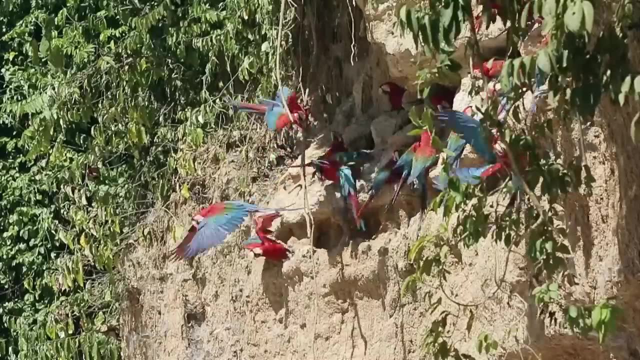 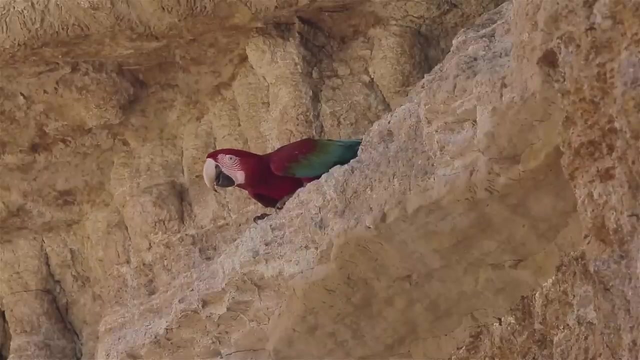 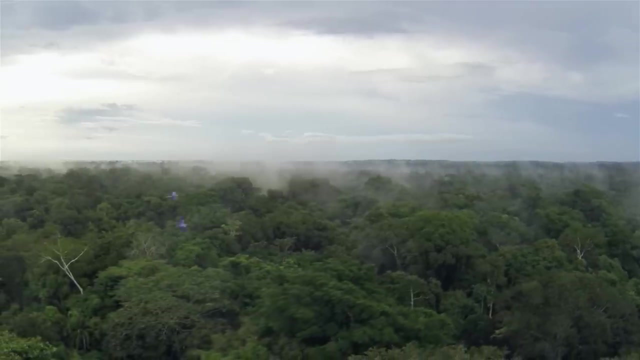 as they see the weather change. The Males have a strange habit of coming up close to the mates to see what's going on, And they like the experience. It's my best thing. I'm just going to have to go to sleep. 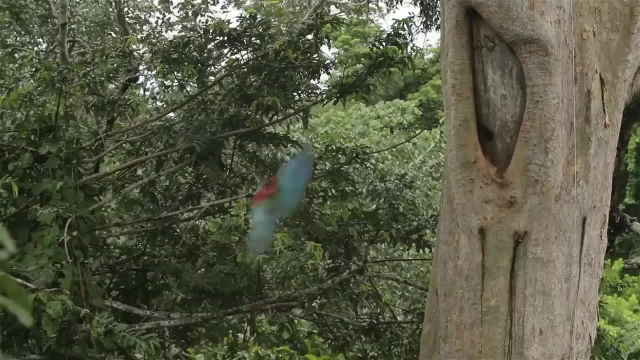 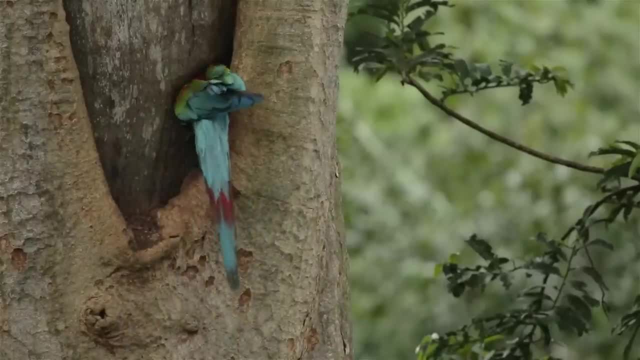 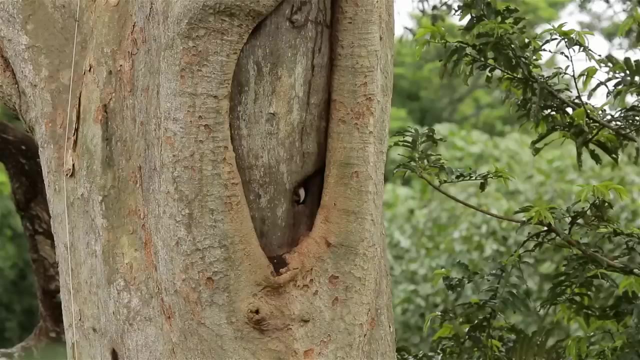 I think the Macaws are going to be interesting. I don't know what the fish are doing there. It's nesting season and high in the branches of a Chihuahua tree, two Macaw parents have enlarged a natural hollow. Inside is a hungry chick who now, after several months of confinement, is beginning to survey. 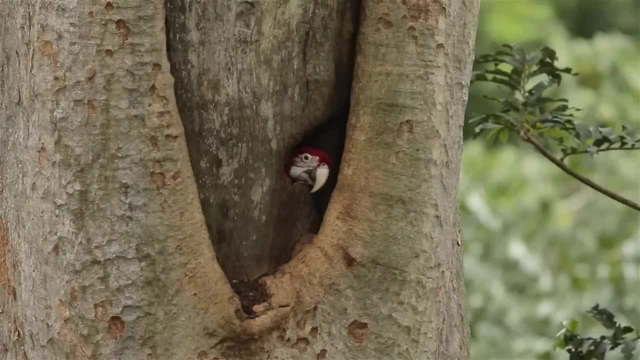 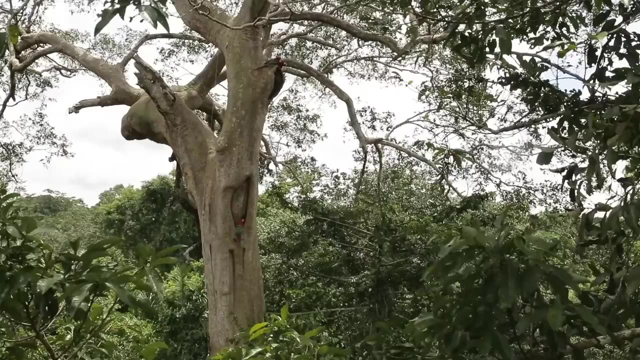 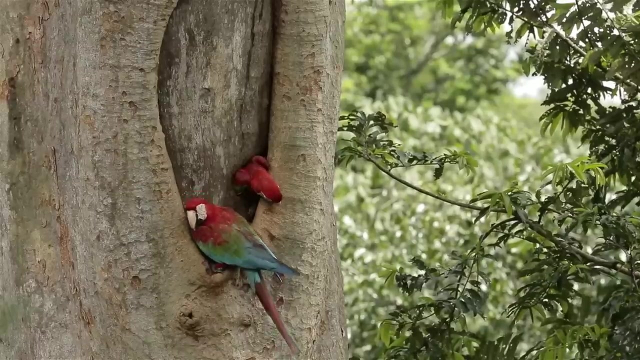 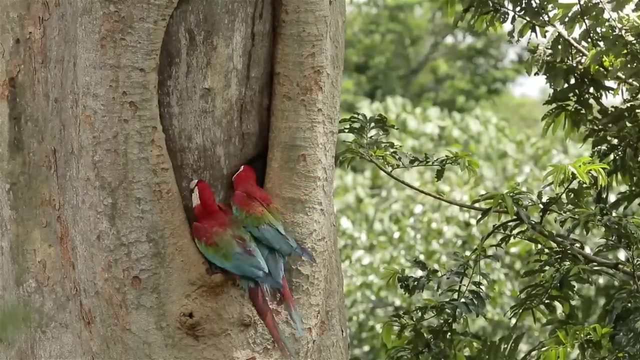 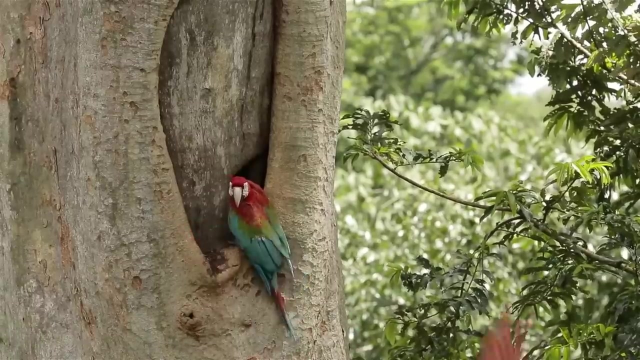 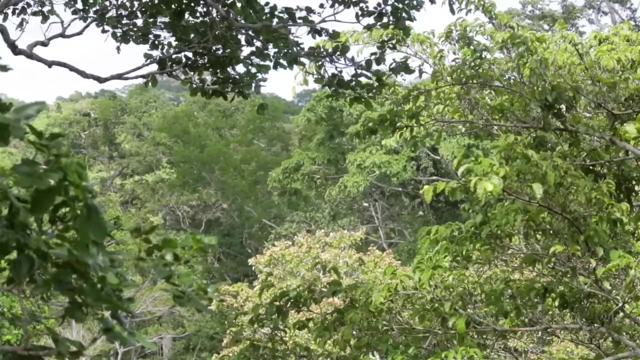 the world outside. For now, his mother and father must deliver his daily dose of clay, but in a few weeks time he'll be ready to fly the nest and follow his parents. For other animals, it simply isn't possible to carve salt from the earth. 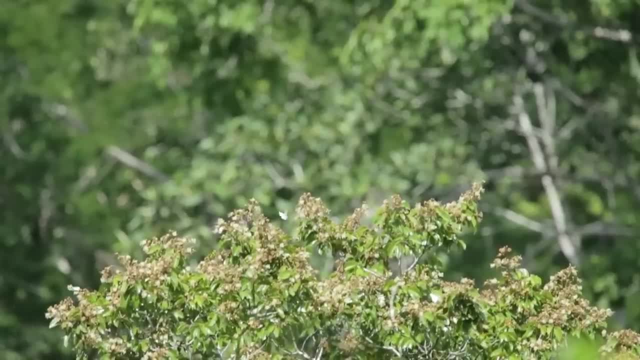 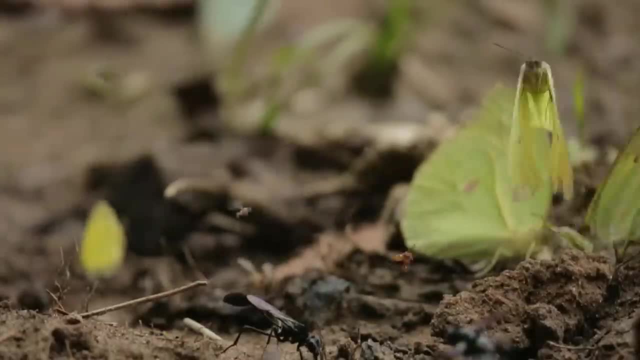 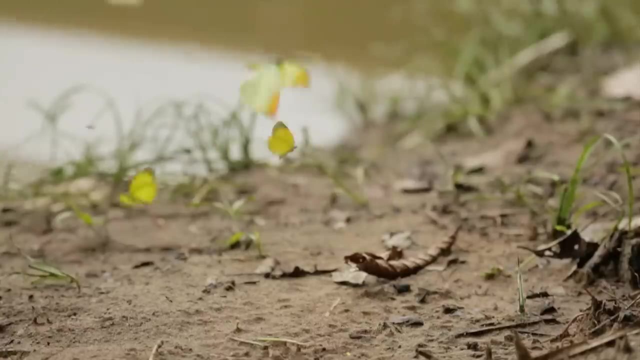 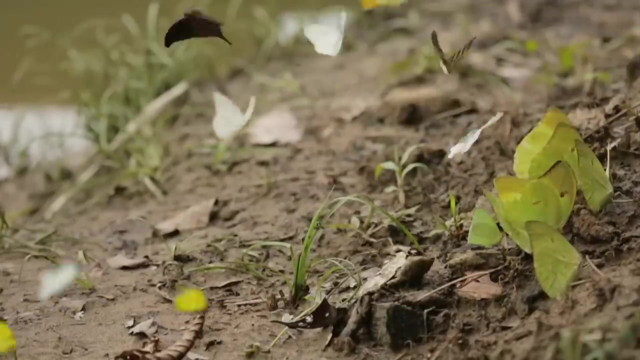 The butterflies congregate on damp earth at the banks of a lake where the waters have receded and deposited salts and other nutrients behind them. But they're cried out and the birds come back into the air to eliminated. But for butterflies, life in the rain forest can be hazardous at best. 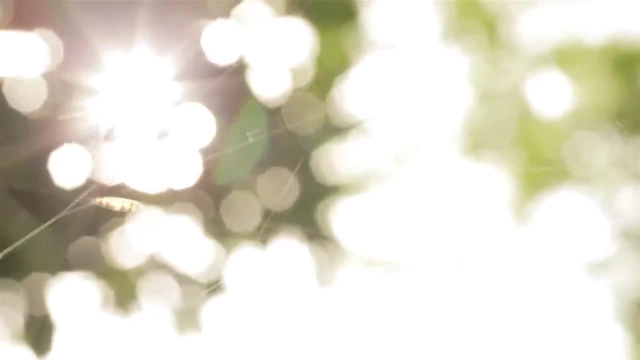 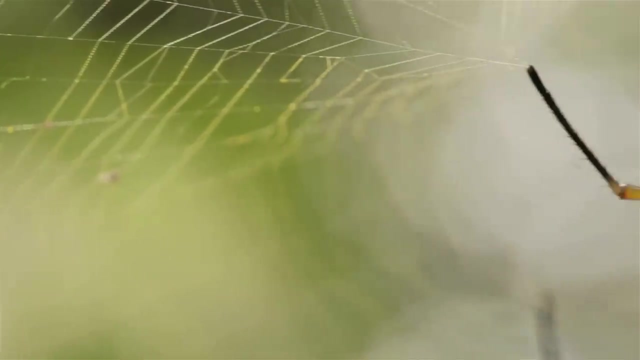 Golden orb spiders are Goliaths, but so too are blue mobile green spiders. There are more than one species of living species in the world, But only many of them are masa nicer than the other species. There's so much there it's impossible to say that's all. 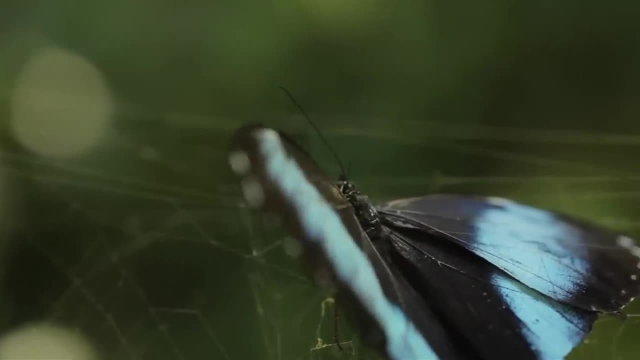 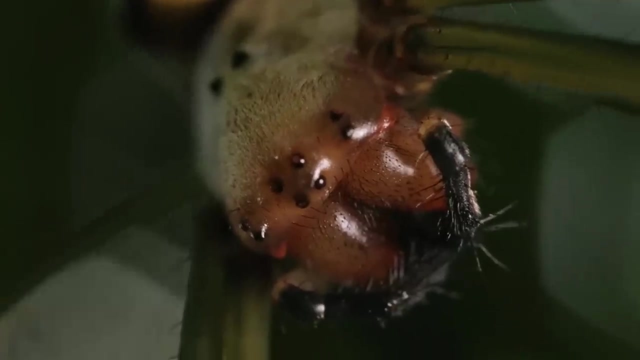 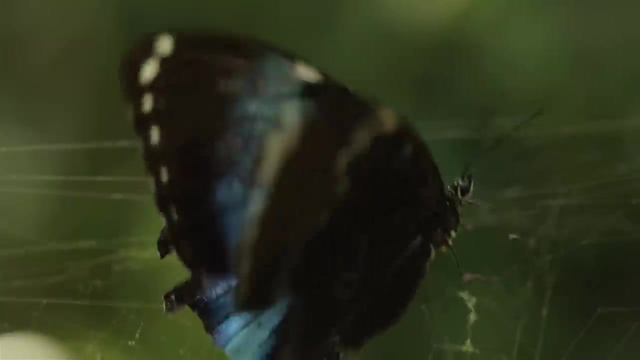 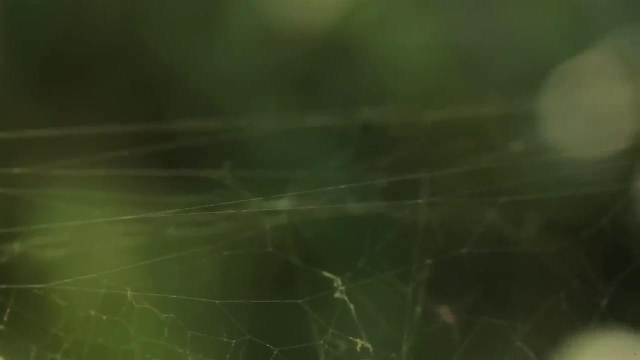 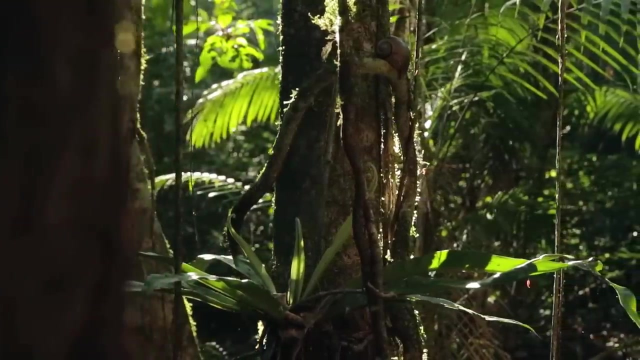 Golden orb spiders are Goliaths, but so too are blue, mobile, green spiders, morpho butterflies. The spider approaches with caution, wary of the butterfly's powerful wings. But butterflies this large don't stay stuck for long. While spiders may pose a nuisance to some, there's one animal here who's been 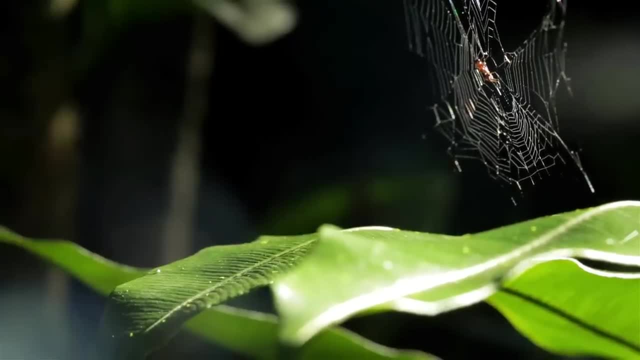 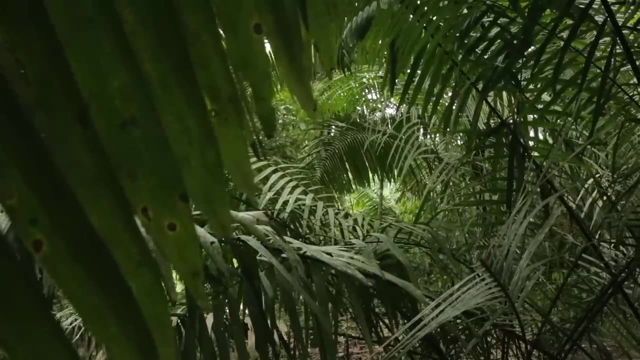 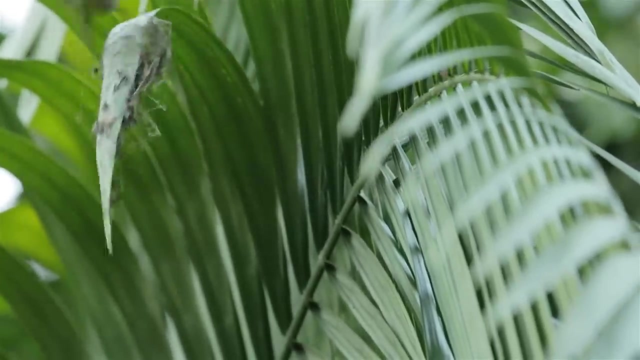 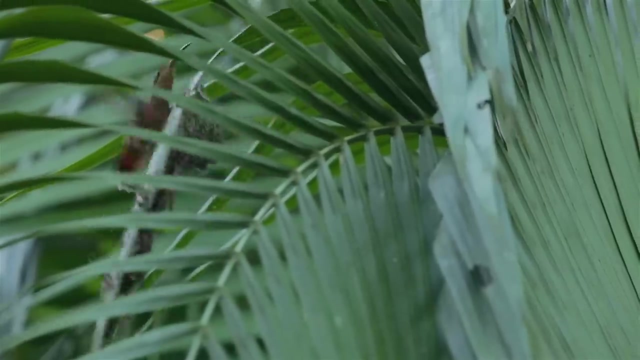 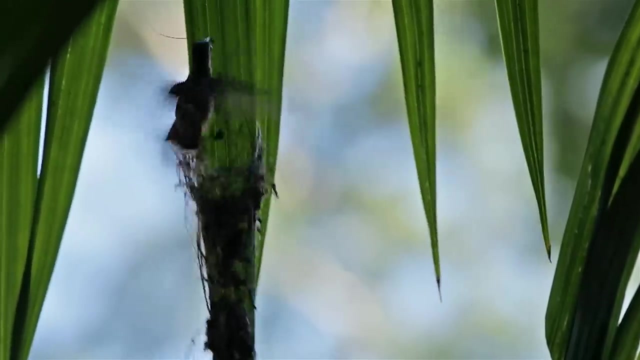 actively seeking them out. This hummingbird is making her first nest, strung together with spider silk and hung from the tip of a leaf. On each trip she can carry a single blade of grass or a tangled strand of spider silk. It takes her weeks to finish. 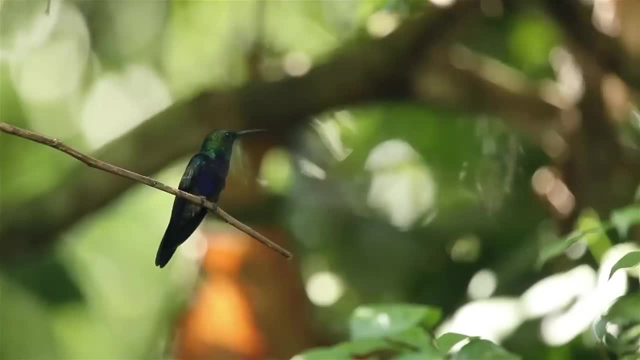 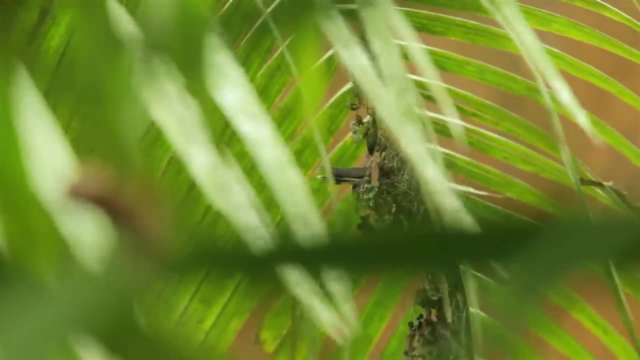 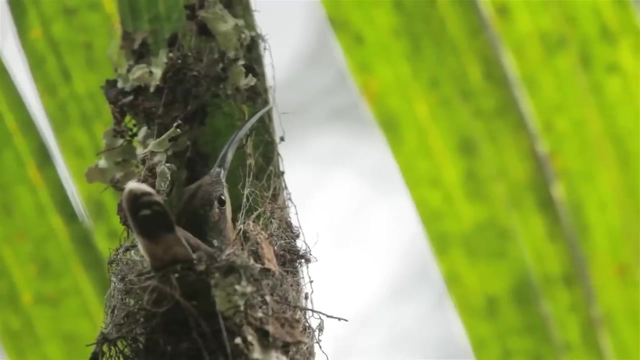 She must remain constantly vigilant as other hummingbirds may try to take an empty nest from the tree. But she must remain constantly vigilant as other hummingbirds may try to take an empty nest from the tree themselves. Once she is ready, she lays a single white egg smaller than a fingernail. 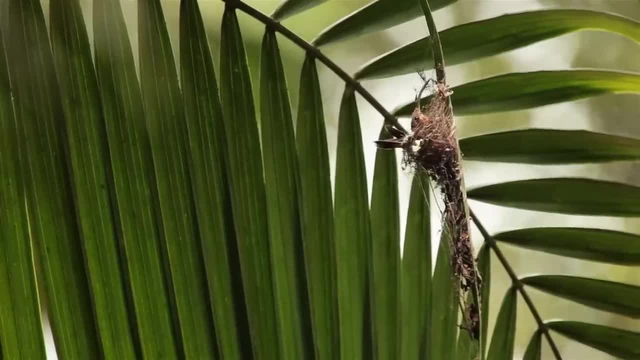 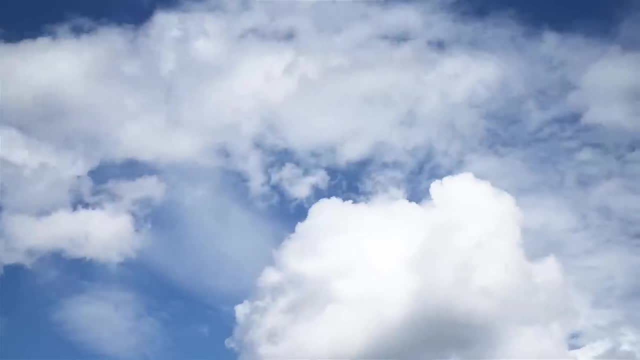 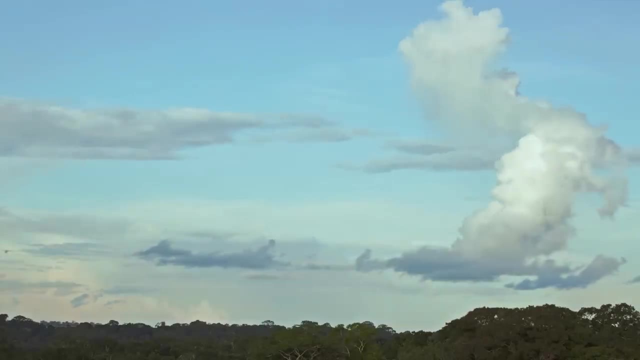 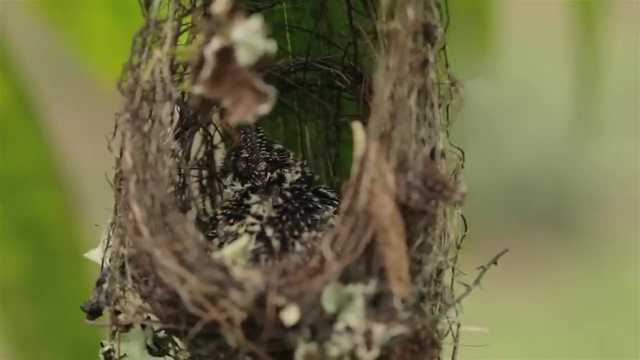 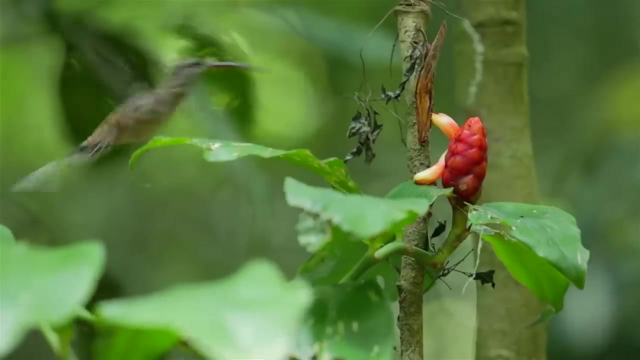 She may seem exposed, but her nest is positioned so far from the palm's stem that only the lightest predator could attack it without falling to the ground. A week later, a tiny hatchling has emerged. Now she must work twice as hard as she is feeding for two. 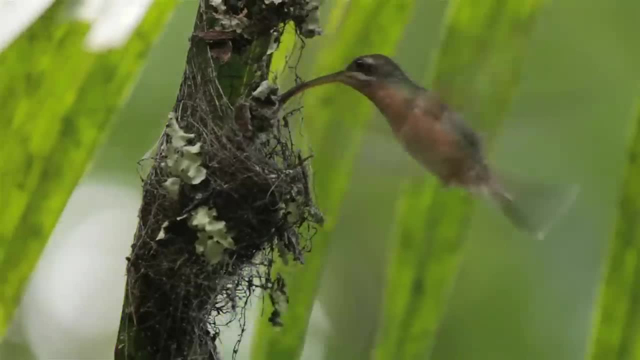 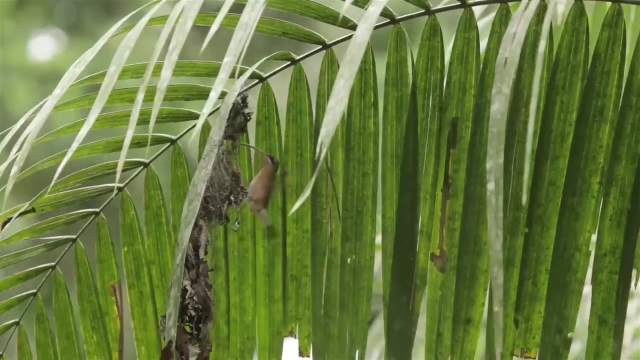 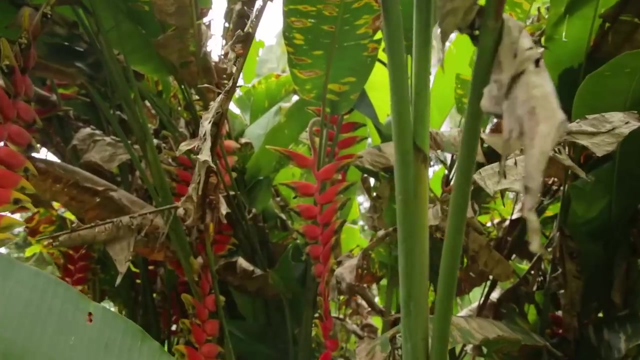 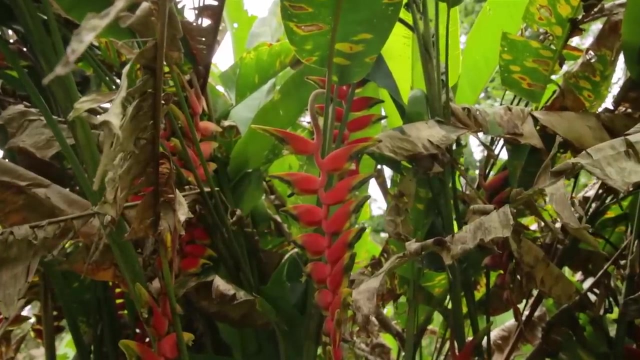 The male has been unable to make a sound at all during this week's work, which is typical of her. She may have lost her life if she had stayed in a primal place for too long. It's still too early, though. 🔊. 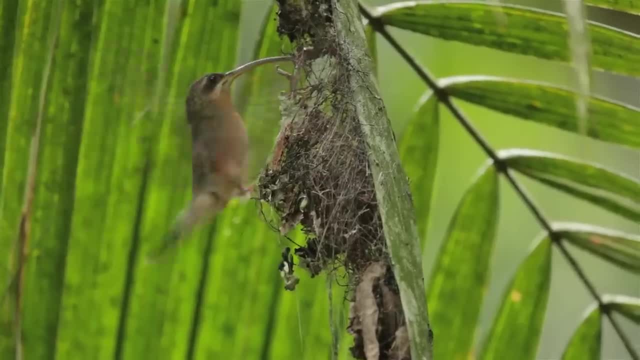 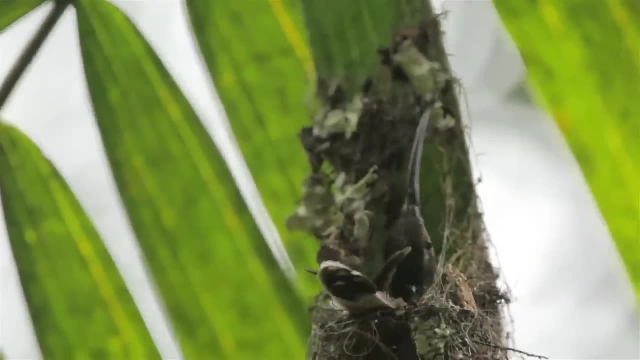 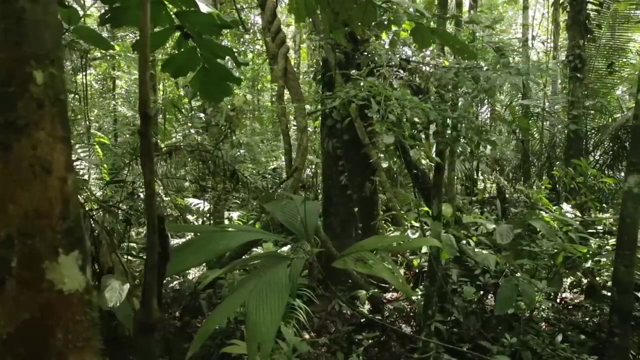 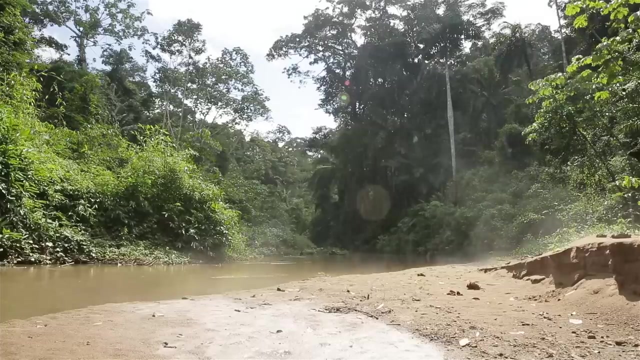 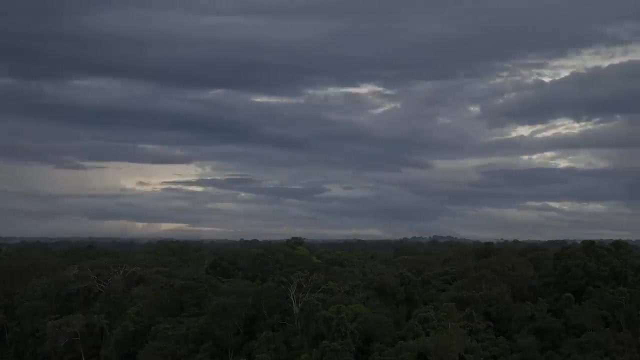 🔊, 🔊, 🔊, 🔊, 🔊, 🔊, 🔊. But the dry season is coming to an end. Her work will soon be put to the test, and her chick's life will depend on it. The temperature has been rising for days, and the air has become saturated with moisture. The creatures of the rainforest can feel it. The rainforest isn't called the rainforest for nothing. In the Amazon, storms hit with a fury like few other places on Earth. The nest is rocked by wind and hammered by rain. The chick must cling to the fibers that his mother so carefully arranged. 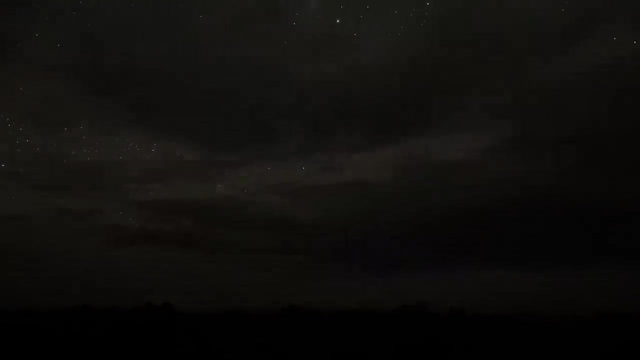 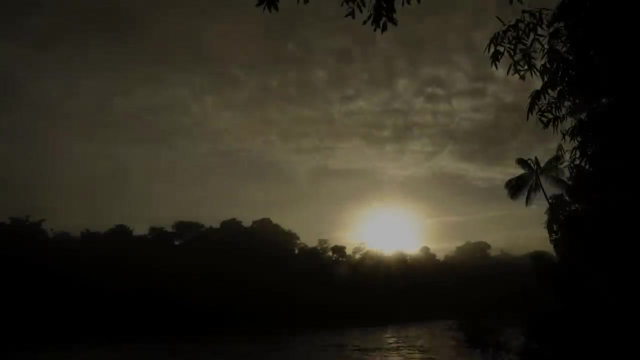 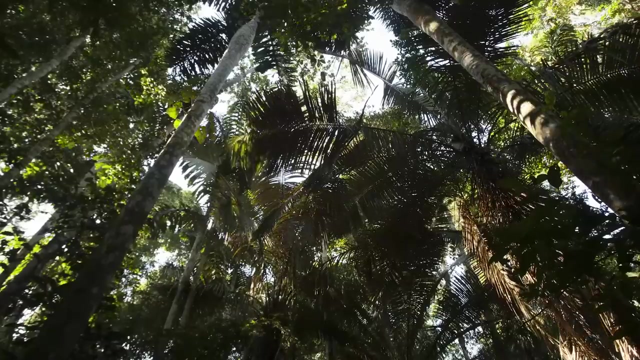 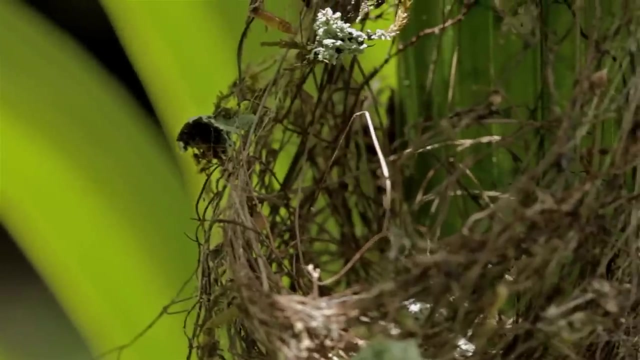 Dawn sees the end of the downpour, but the storm's effects can still be felt. The mother hummingbird returns to find her chick gone and the nest empty. In her distress, the mother hummingbird returns to find her chick gone and the nest empty. 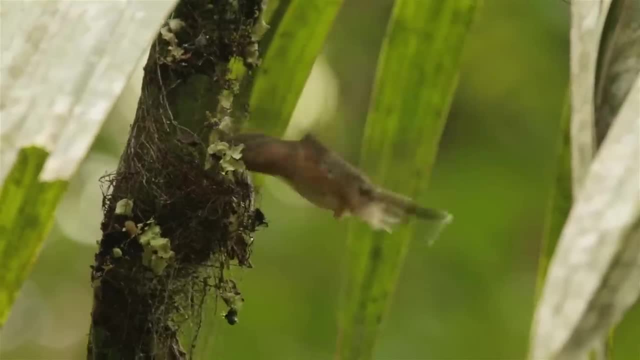 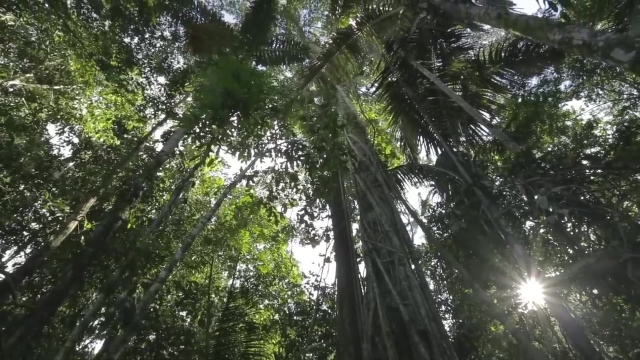 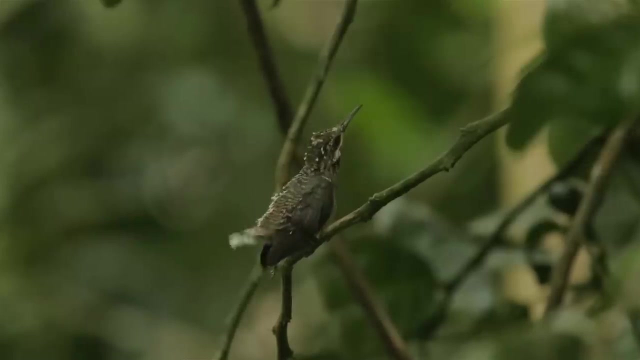 The mother hummingbird returns to find her chick gone and the nest empty. In her distress she checks for him over and over. He may have survived, but having been blown from the nest during the night, he's now alone in the rainforest. 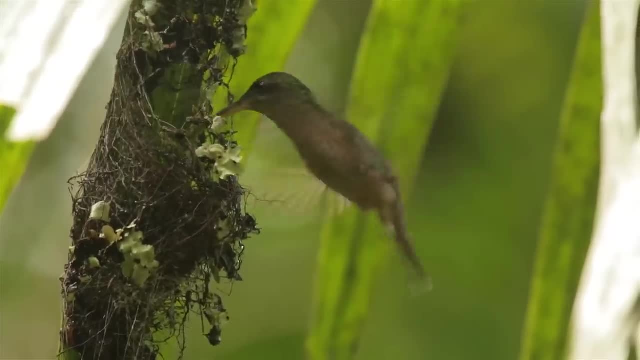 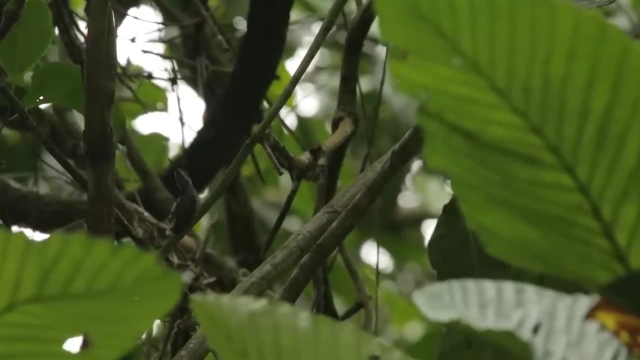 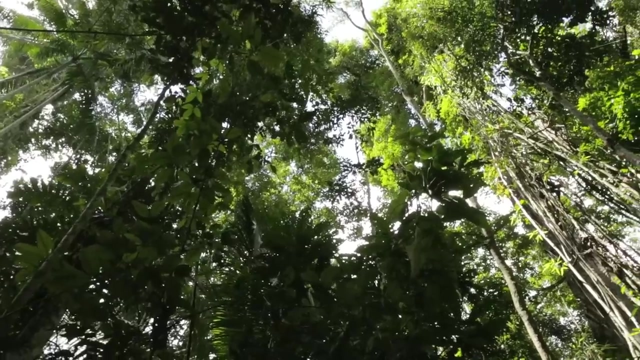 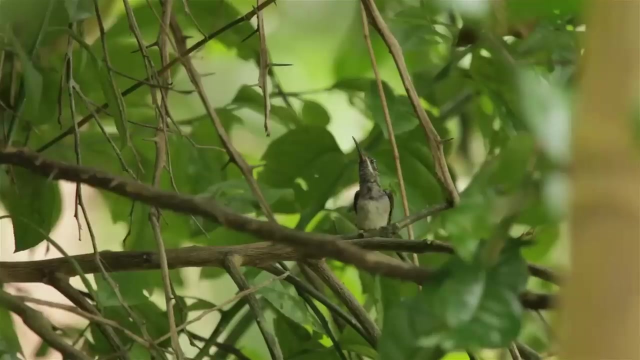 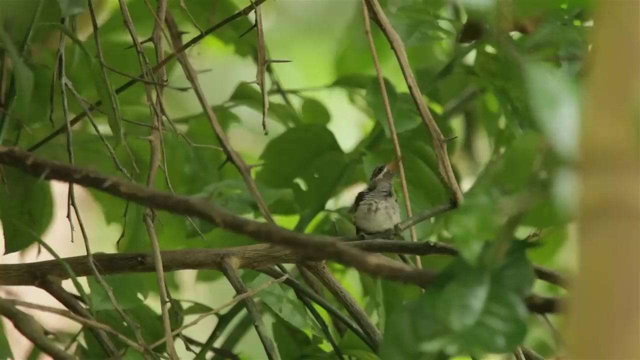 He doesn't yet know how to find food for himself, so she must find him quickly, or else he will starve And he'll need to wait for the nest to be destroyed. Their calls to each other sound out across the forest And the two are reunited once again. 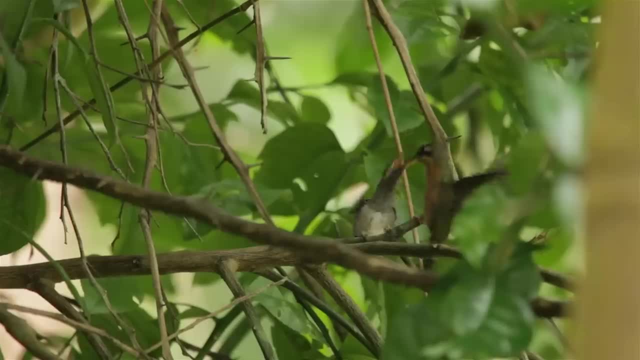 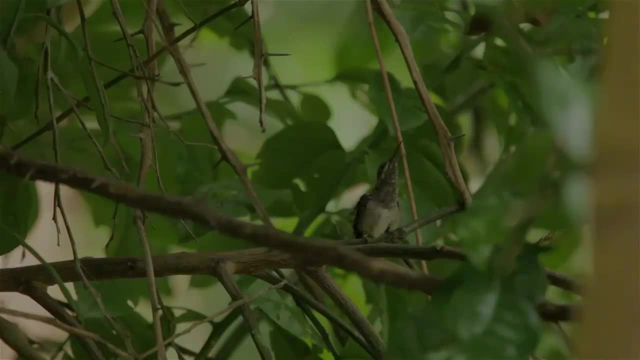 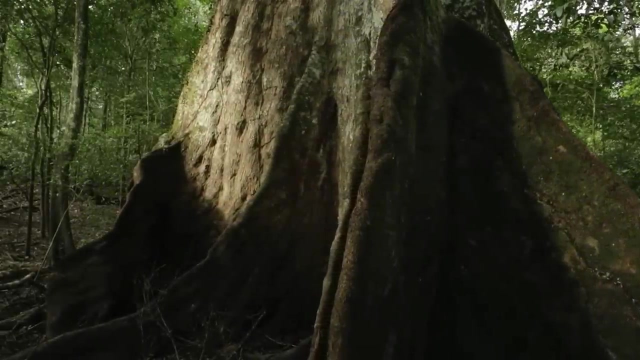 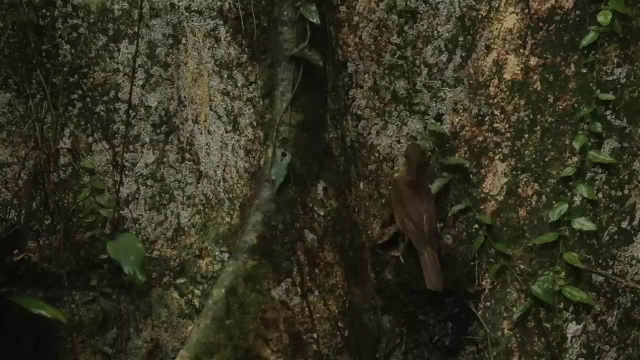 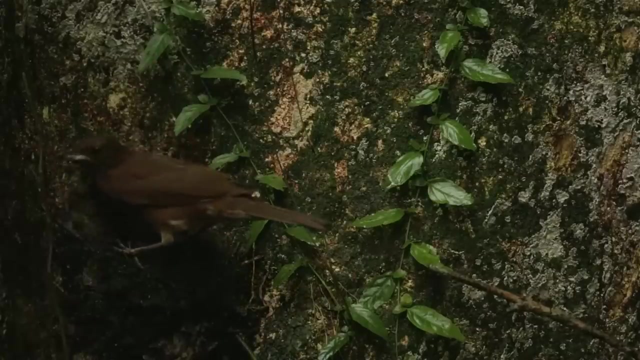 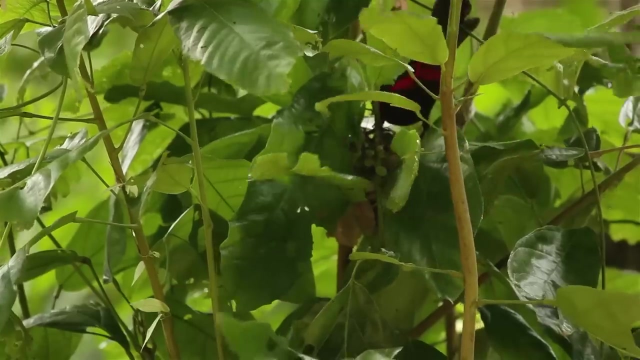 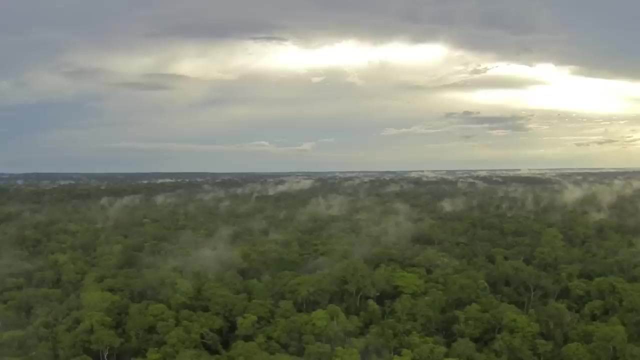 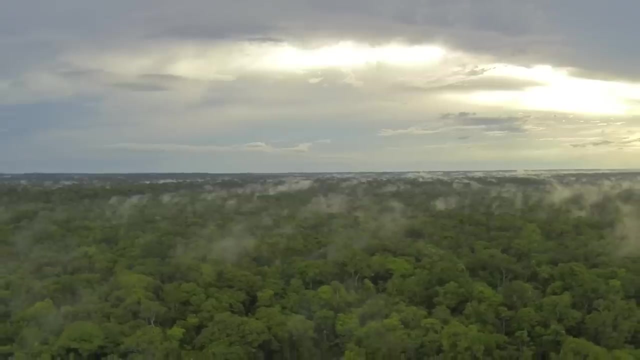 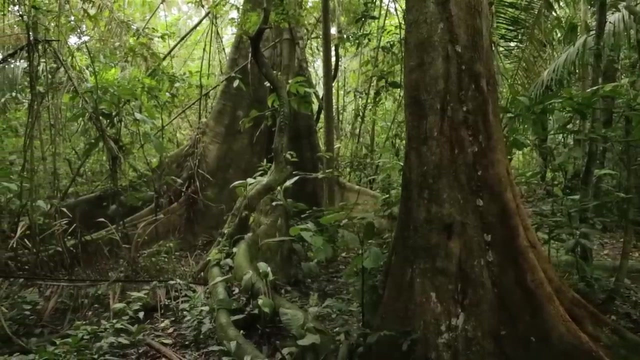 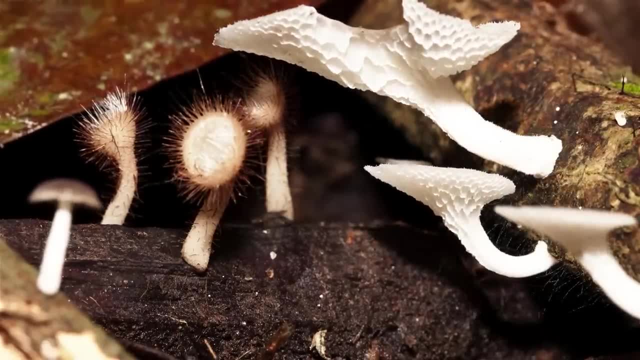 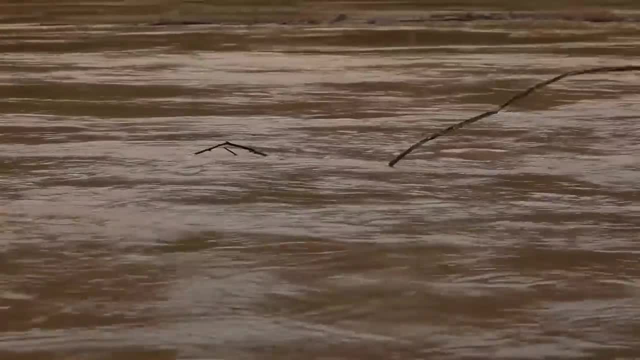 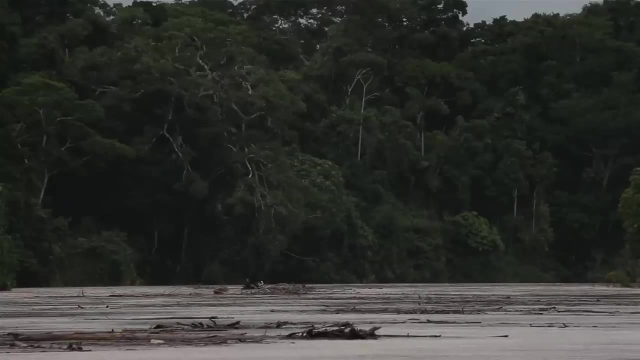 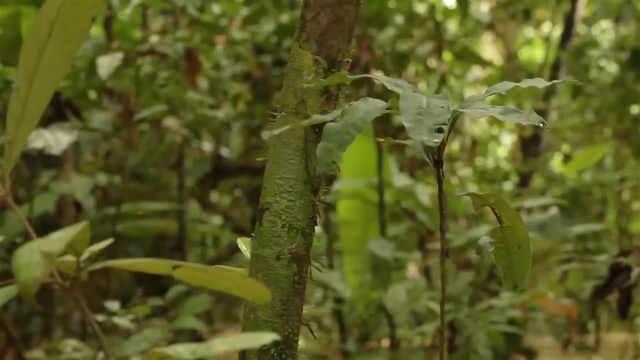 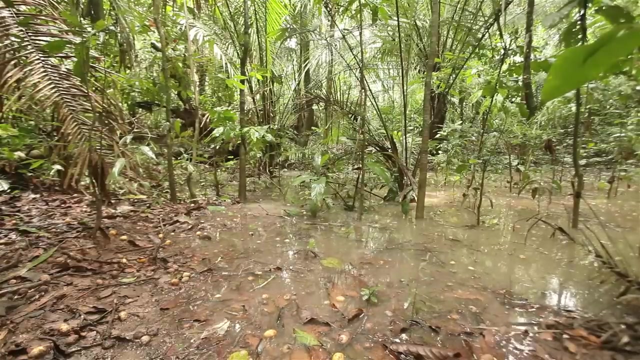 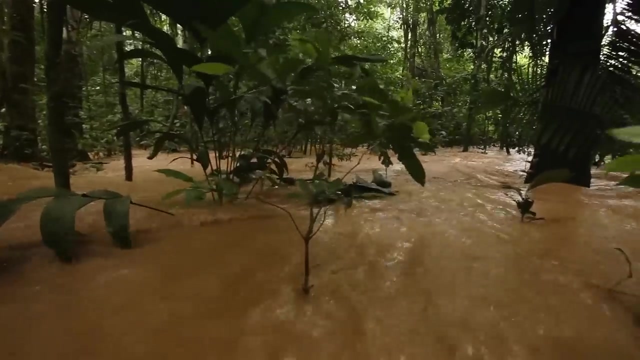 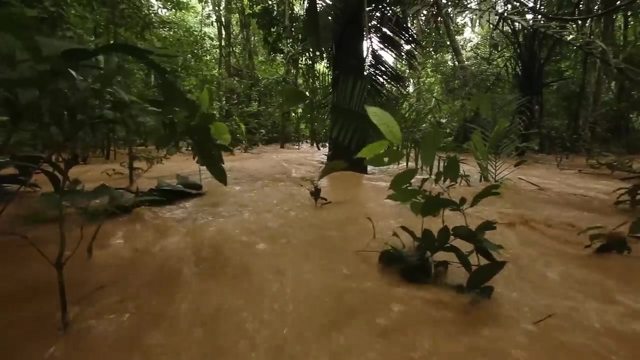 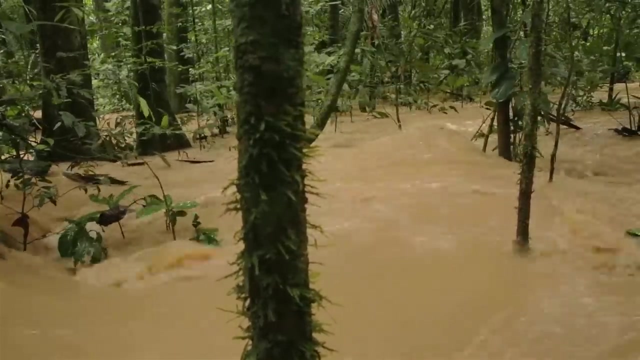 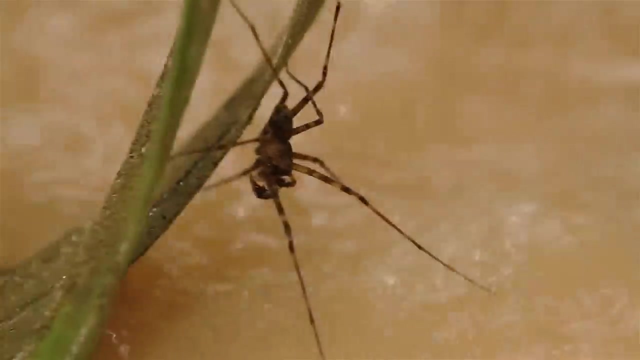 But they have also brought destruction. The Les Piedras River is bursting its banks. Entire trees are carried away with the current. The swelling river surges through the forest. For those too small to outpace the flood, the only way is upwards. 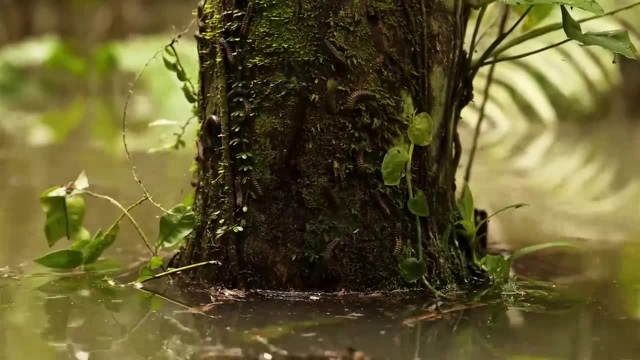 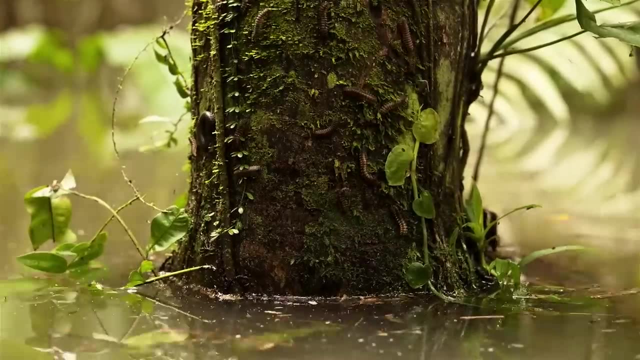 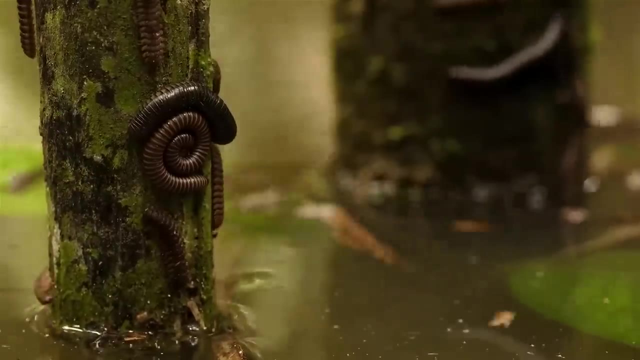 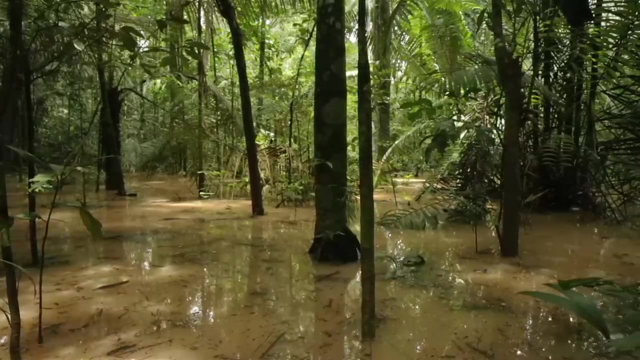 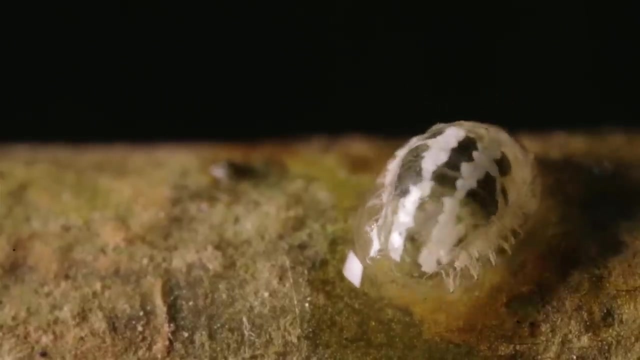 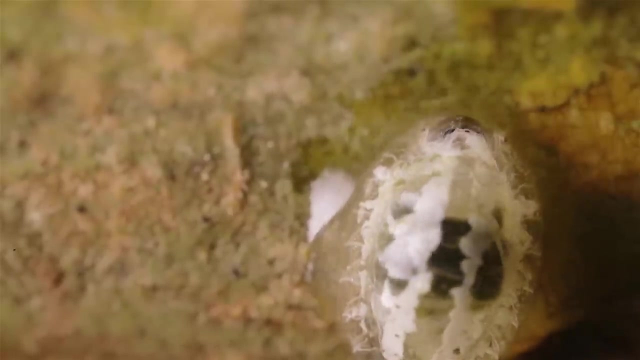 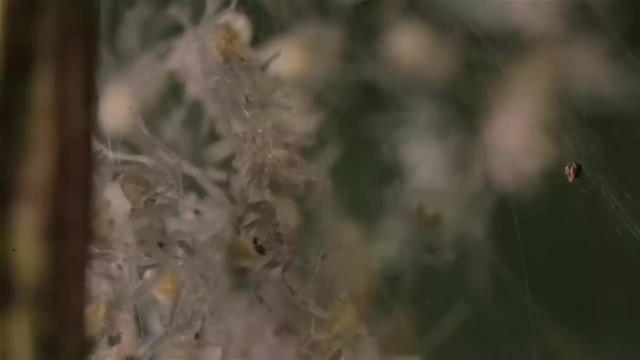 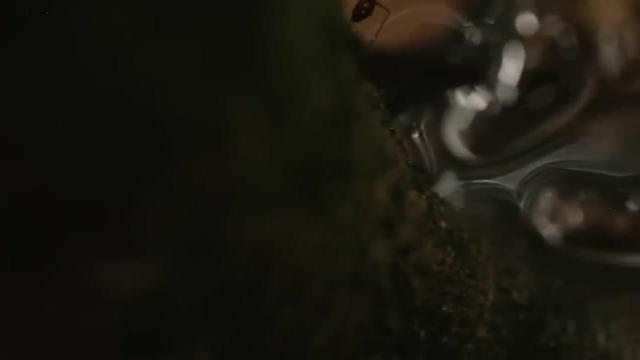 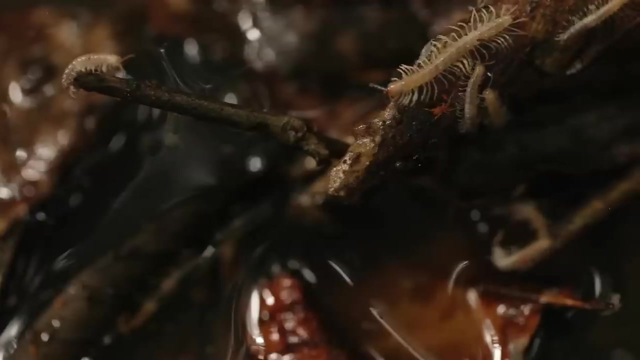 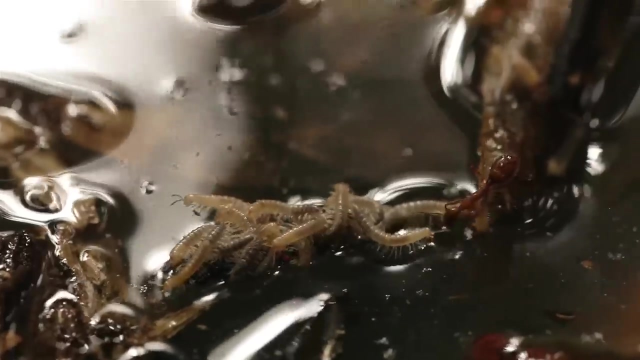 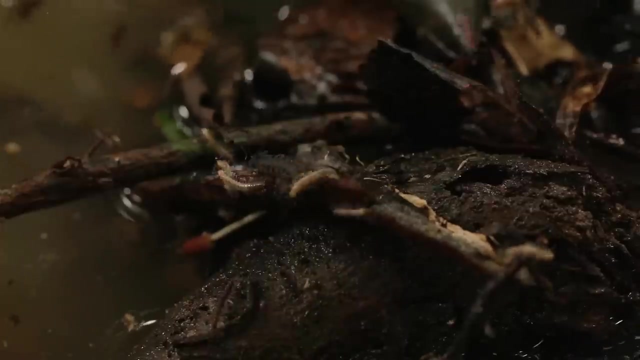 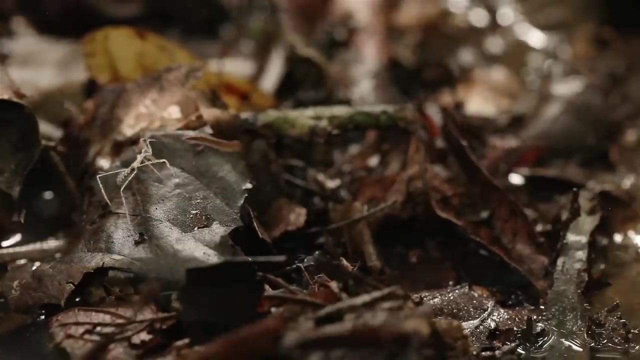 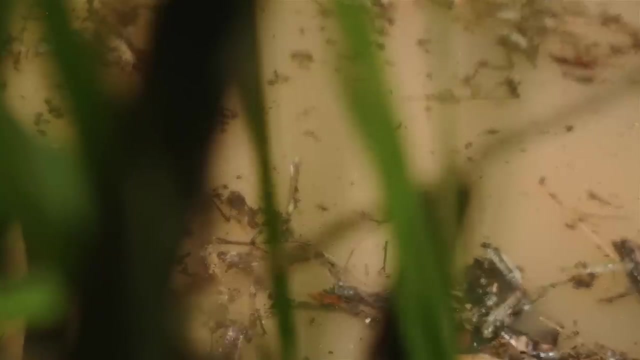 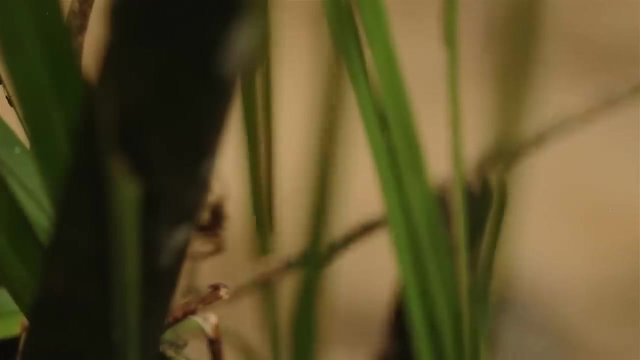 Every available inch becomes saturated with life. Strange forms are forced from the darkness. curtain dwells. For many, high ground is nothing more than a few floating leaves. curtain dies. The search for escape is constant. In such crowded conditions, predators are spoiled for choice. 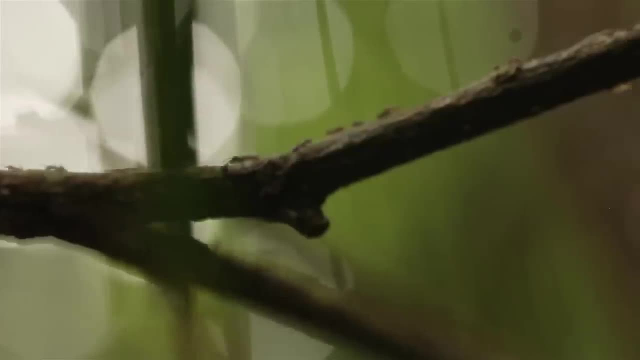 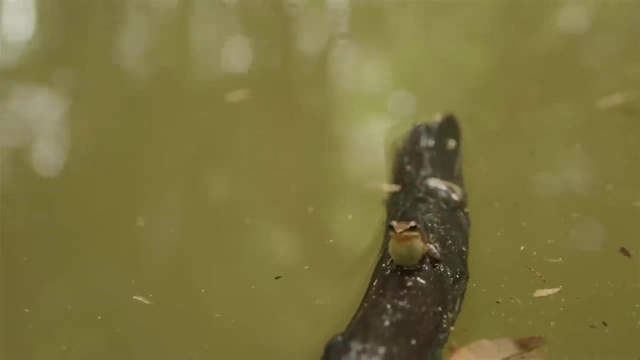 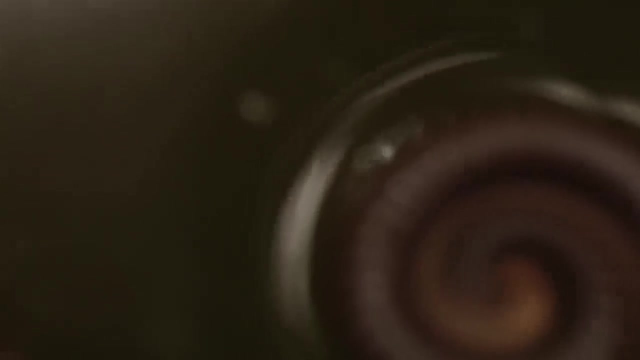 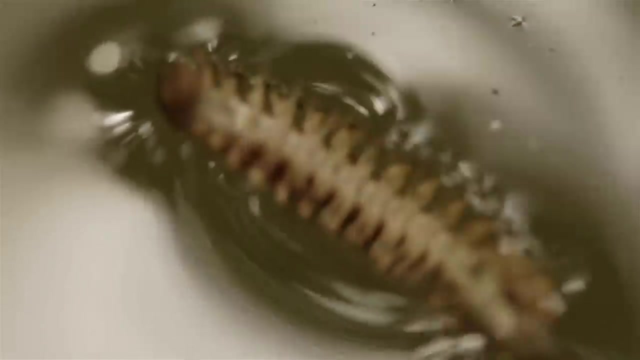 Isolated on their treetop arcs. it could be weeks before the river recedes and the creatures of the forest touch solid ground once again. Many were too slow to escape the rising water. Surface tension will keep millipedes afloat for a short time, but if they begin to struggle, 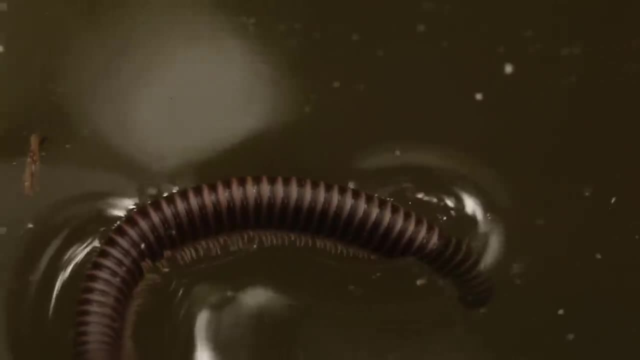 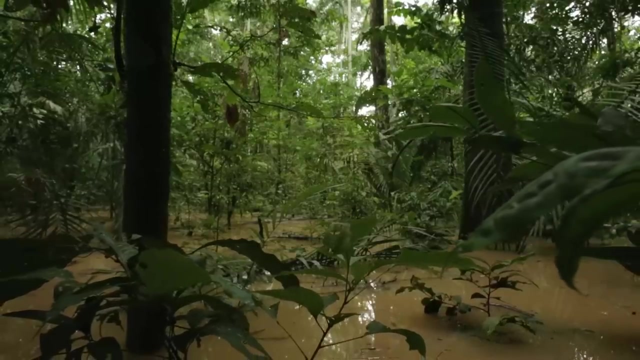 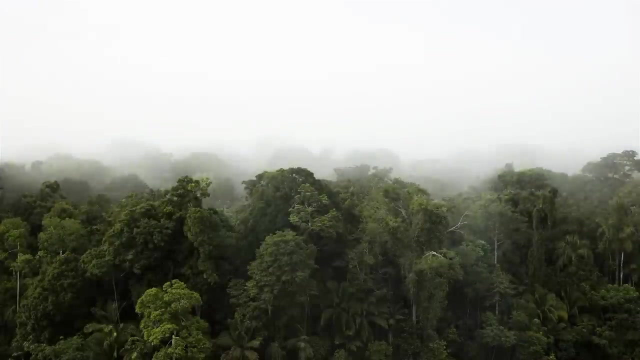 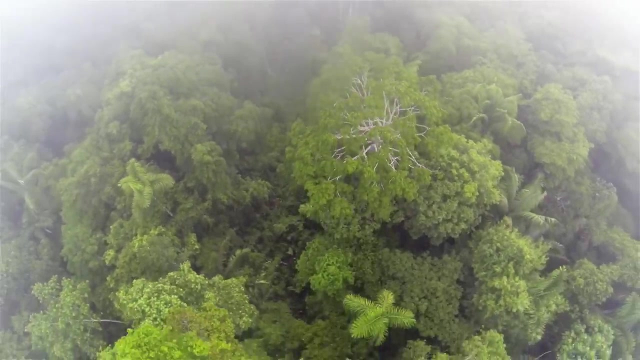 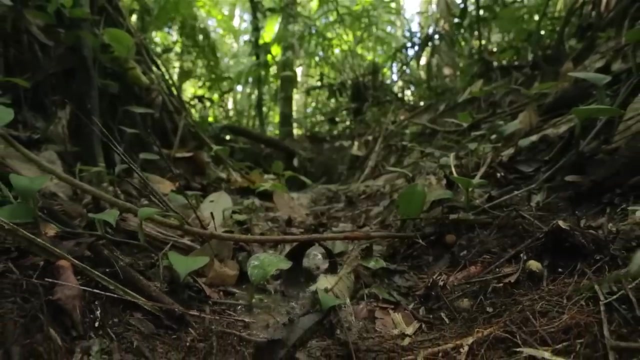 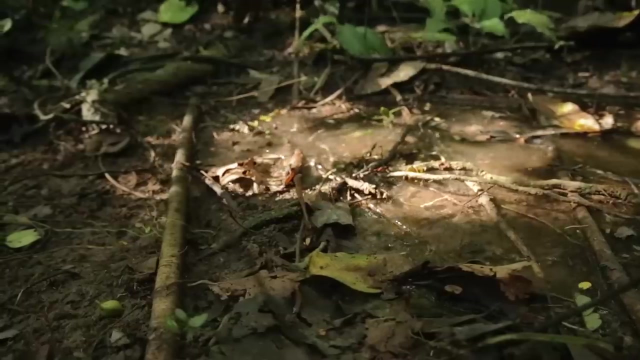 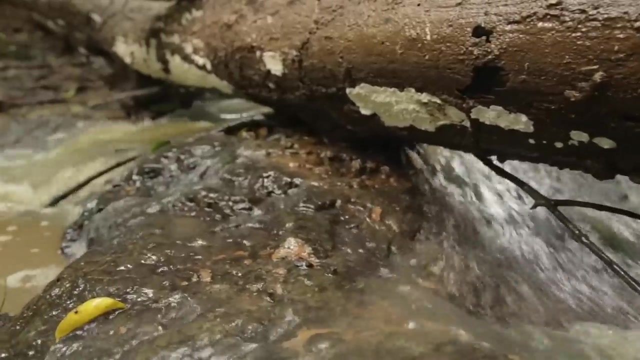 their legs break through. Attempts at escape only serve to seal their doom. The arteries of the jungle are now springing back to life. As the waters continue to rise, many creatures once isolated in pools and lakes are now free to move on. As the waters continue to rise, many creatures once isolated in pools and lakes are now free. 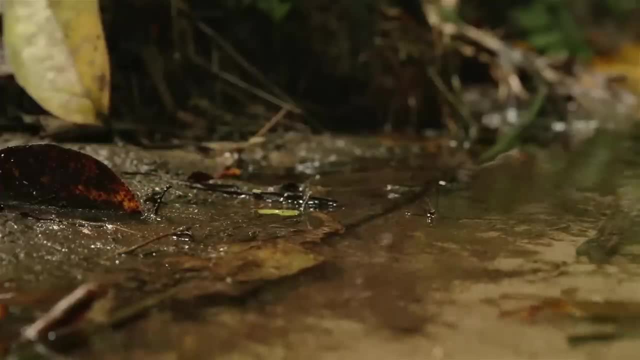 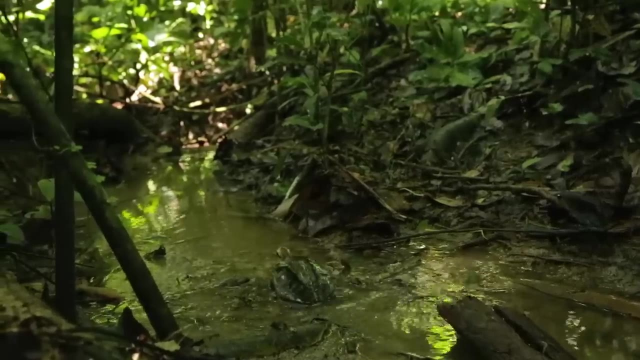 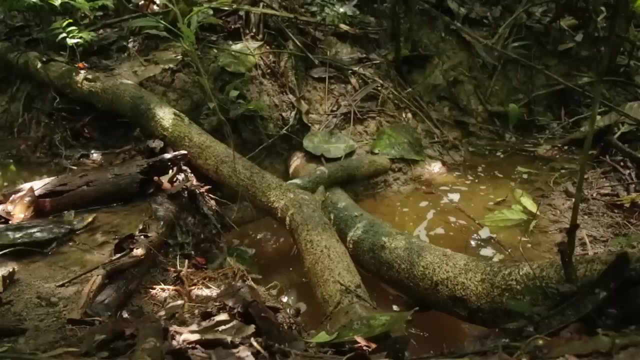 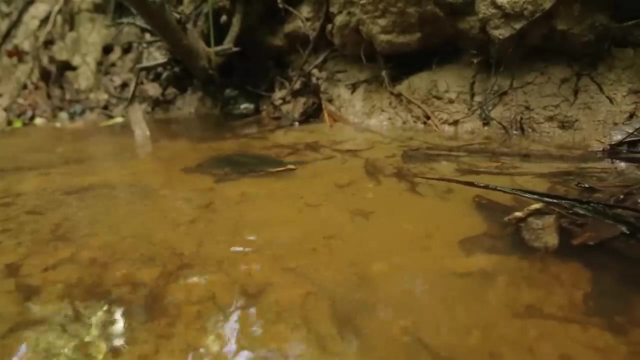 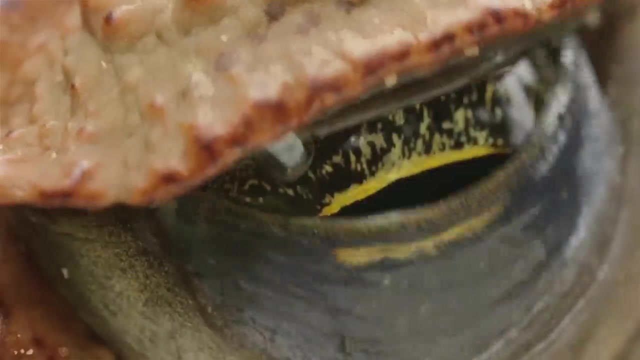 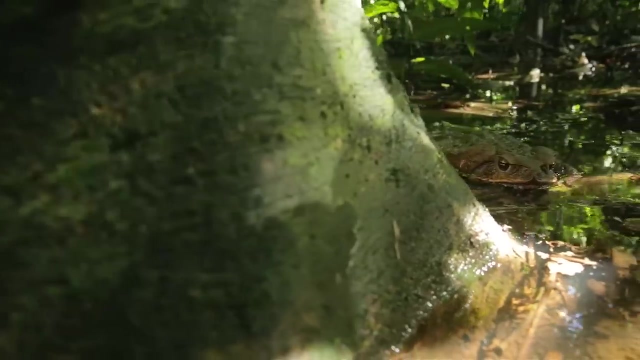 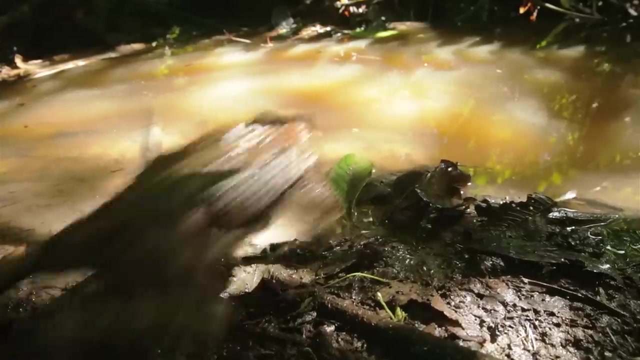 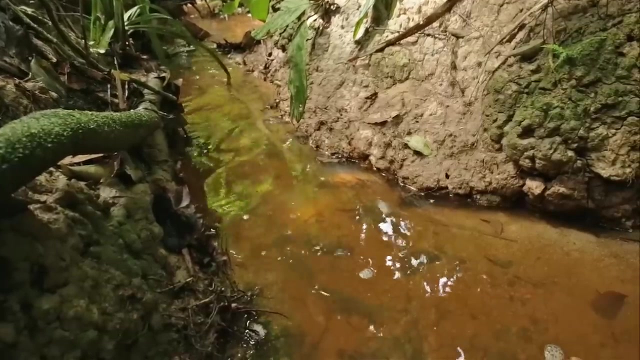 to move on Pursuing the use of the jungle. Gronin has found his second true goal. Whoa, A bird is an amazing equalizer. Fish are searching for a safe place to lay their eggs and predators are ready to cut them off. 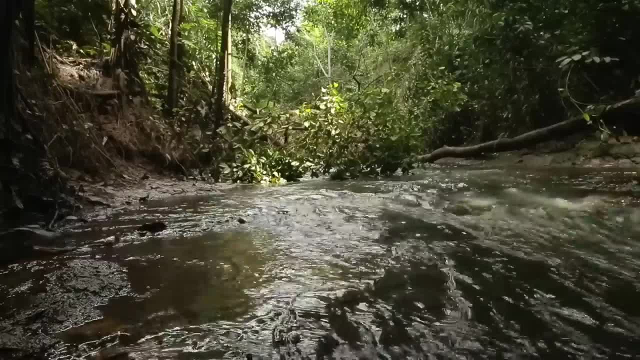 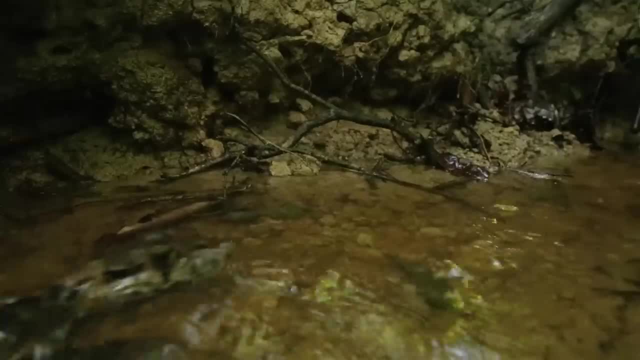 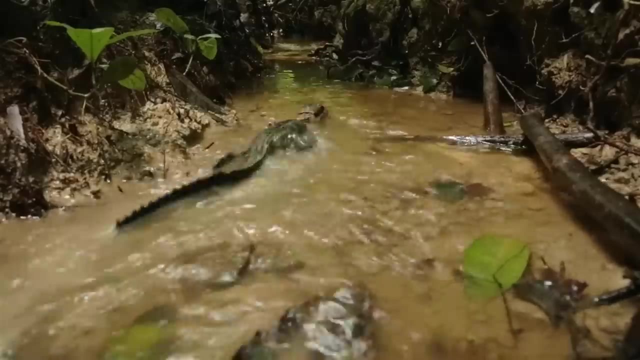 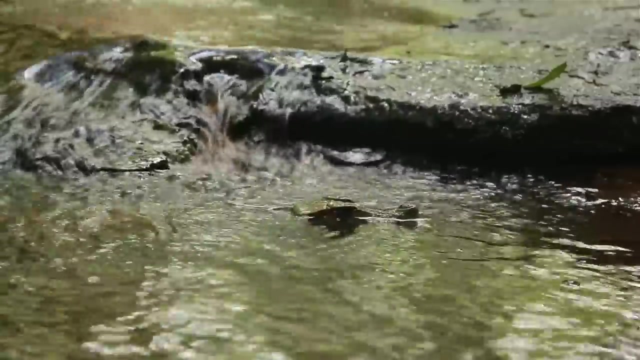 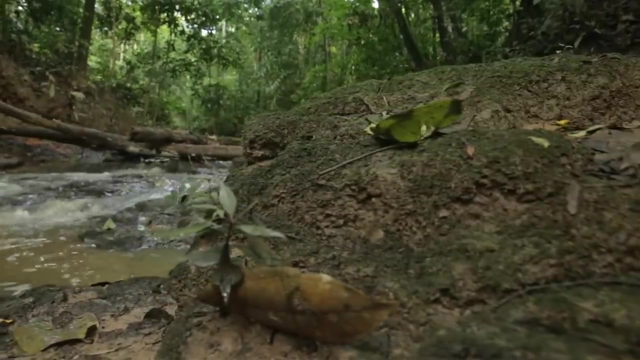 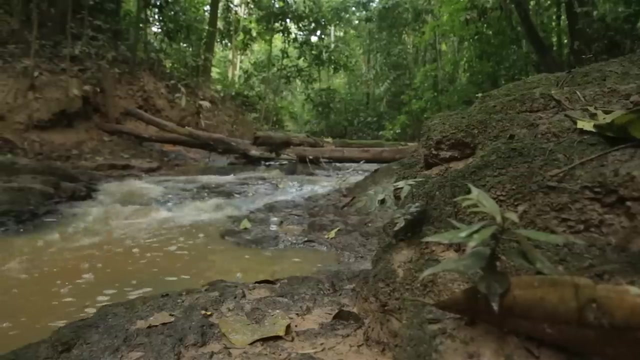 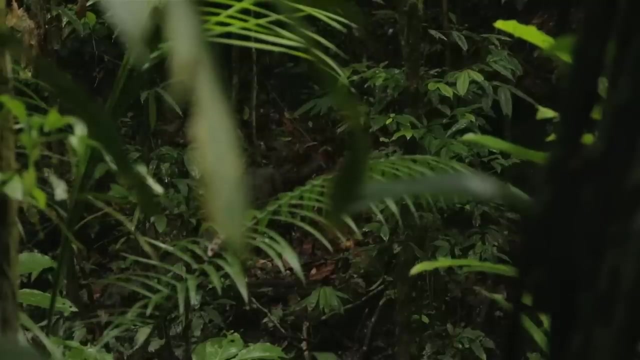 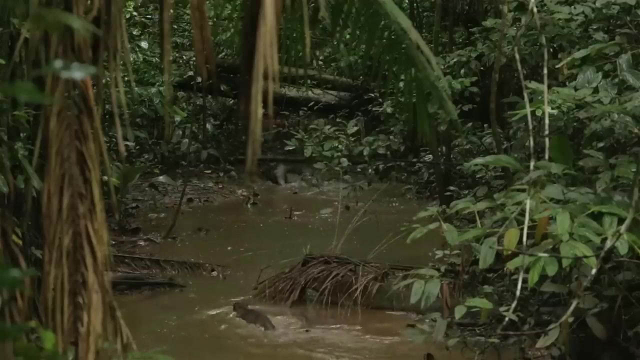 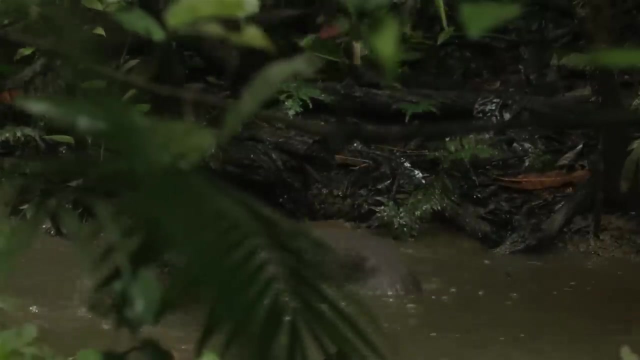 They're ready to lay their eggs. A new chorus is sounding through the depths: A family of giant river otters, seven strong, are also here to take advantage of the fish to be found in the swelling streams. And just as well, because this family 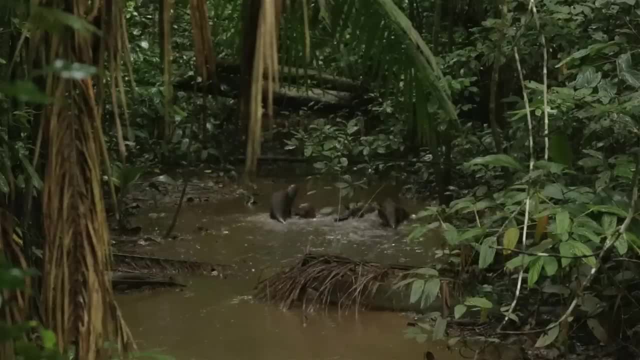 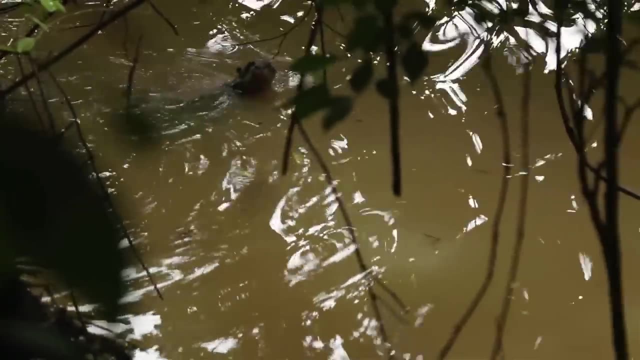 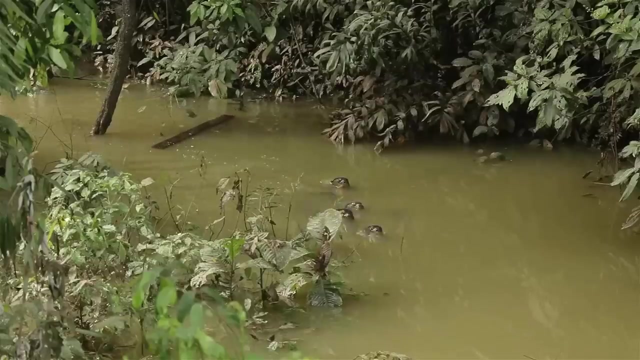 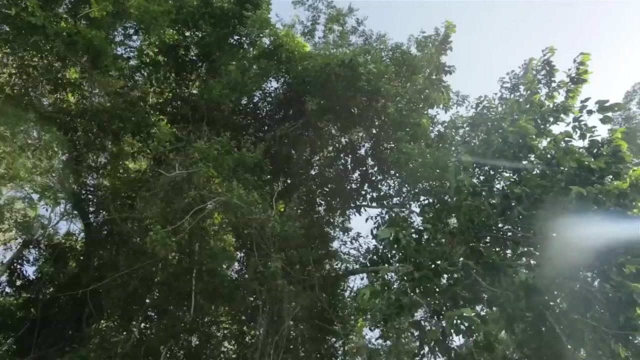 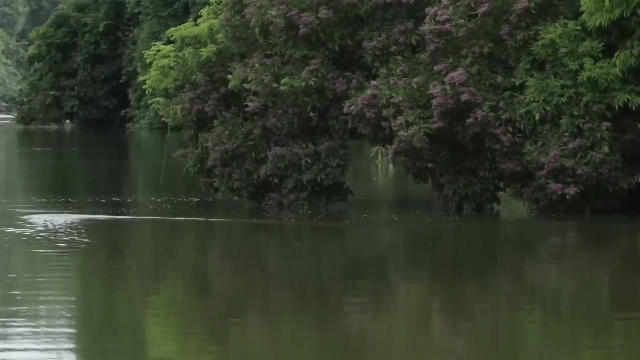 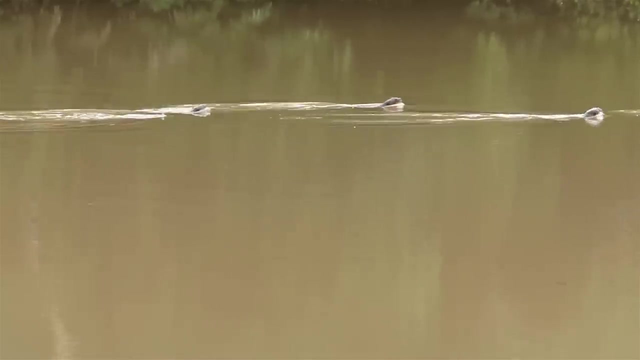 has three hungry cubs to provide for. But with so many mouths to feed, the otters can't stay in the streams forever and must move on to places of greater abundance. They spend most of their time in vast lakes hidden deep in the forest. 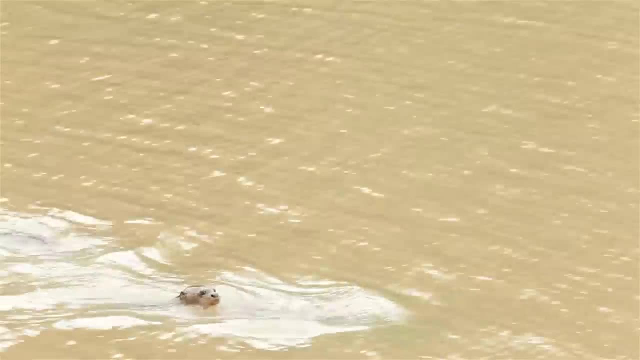 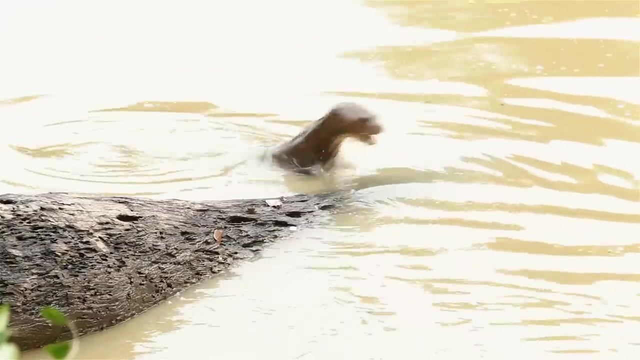 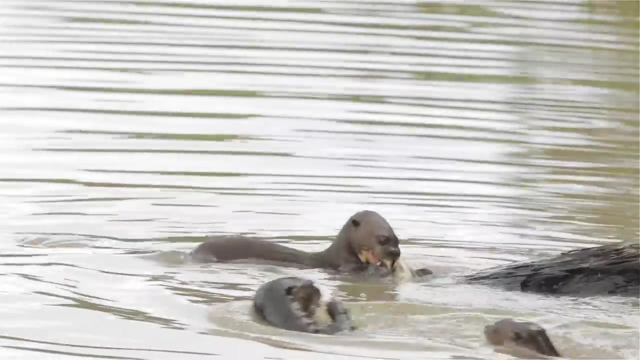 Half of giant otter cubs don't make it through their first year, but these are the lucky ones. They have made it past the crucial stage in their lives when they are most vulnerable to predators. They have found their way through the water. 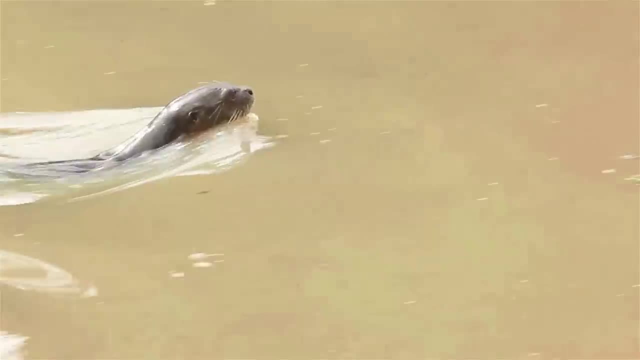 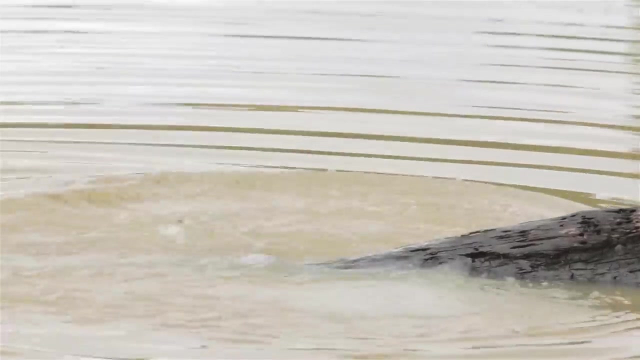 and have found a safe place to lay their eggs and have found a place to live. They've found their way into this new life, and the only thing they're left with is a safe place to live. Nevertheless, they're still young enough to get away with stealing a fish from mom. 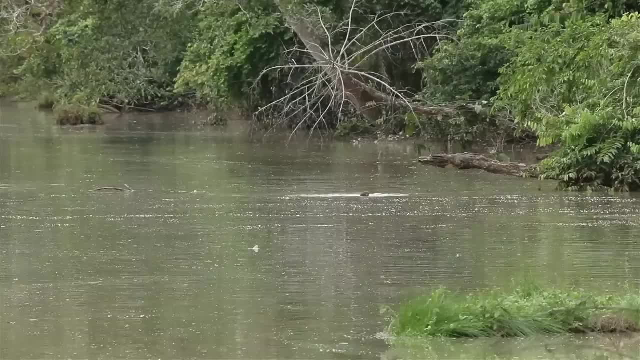 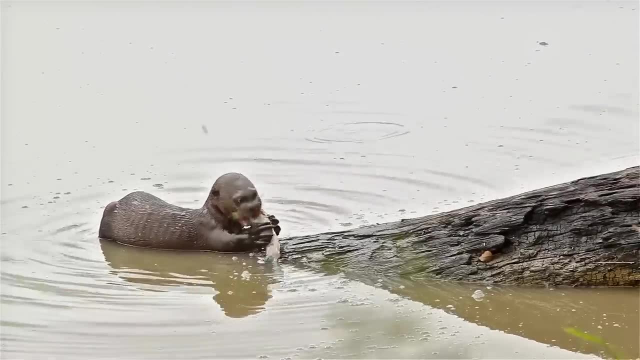 rather than hunting it for themselves. The cubs' jaws still aren't strong enough to dispatch a fish quickly, so they have to keep a careful grip Sometimes. a live fish is not always the best bait. They need a good fish to keep their mouth shut. 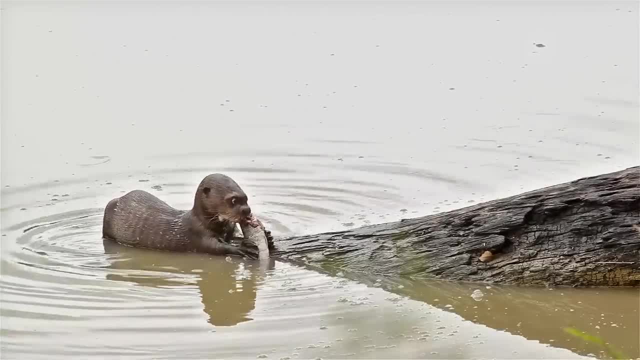 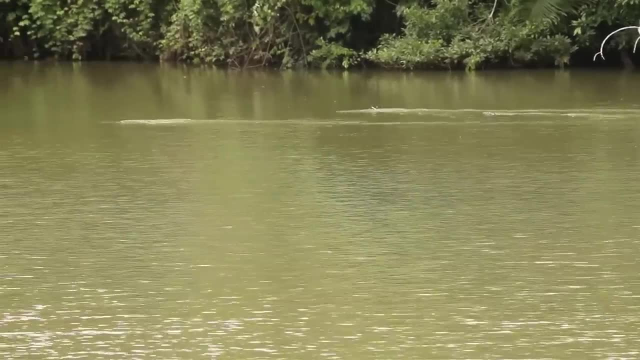 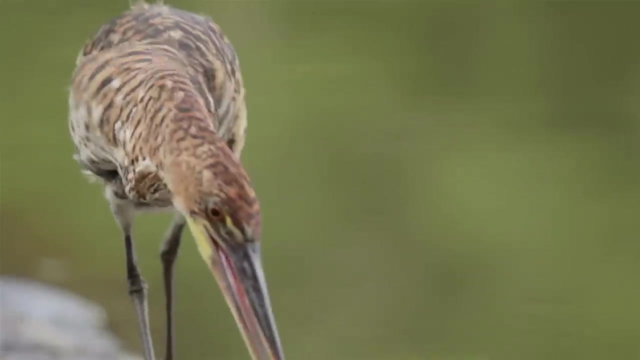 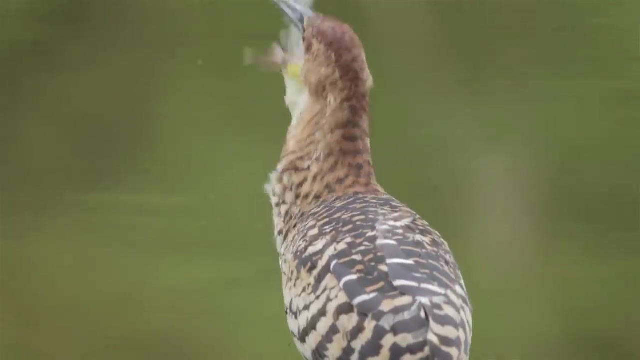 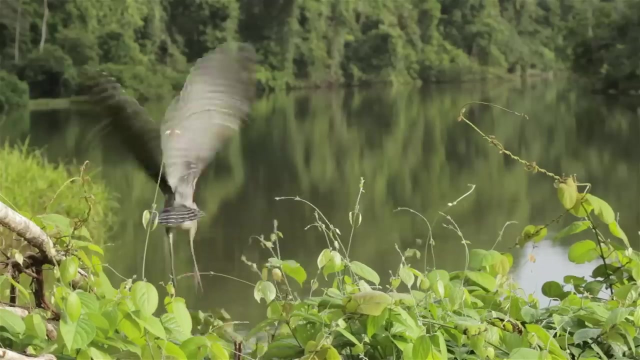 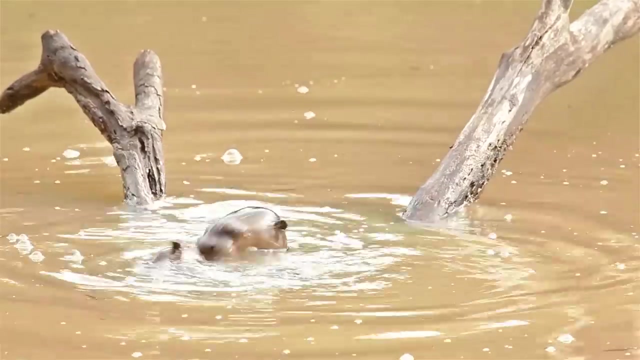 Sometimes a live fish is better than a dead fish. A live one can be a little startling. Other animals stay close behind the otters and pick up their scraps, But they aren't welcome everywhere With full bellies. there's plenty of time for play. 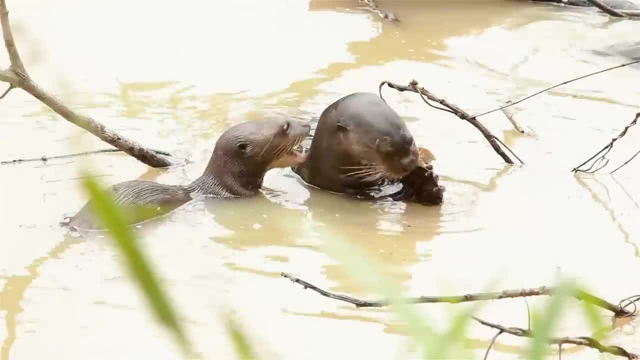 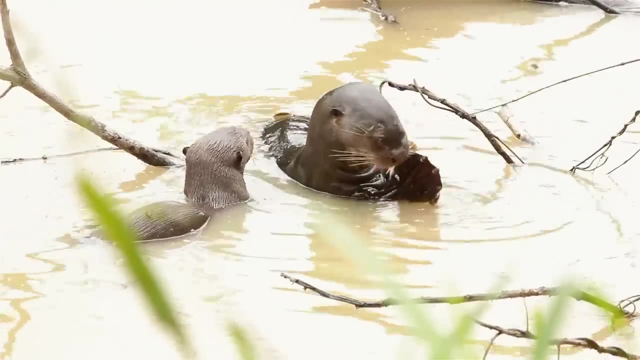 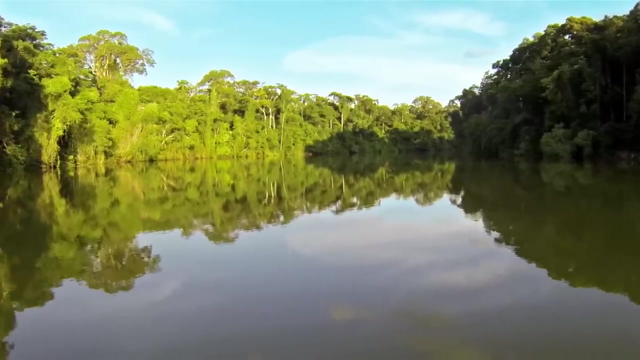 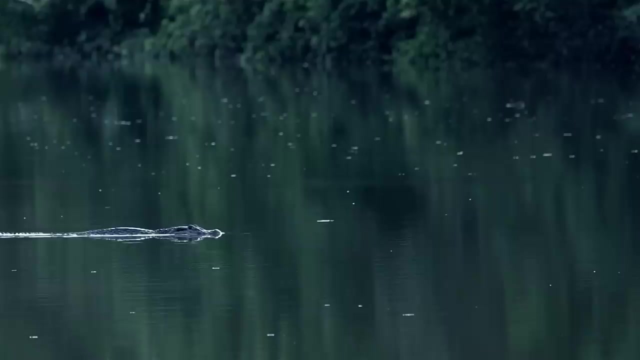 In a few months, the cubs will reach their adult size at two meters long, But for now they must still be careful not to stray too far from their parents, For these waters are home to another top predator. Male black caiman are highly territorial, and this five meter long individual is a new arrival at the lake. 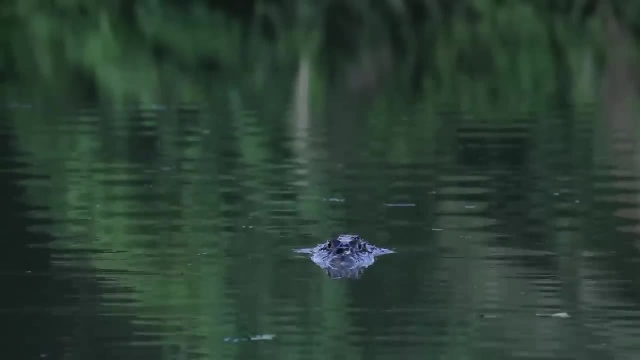 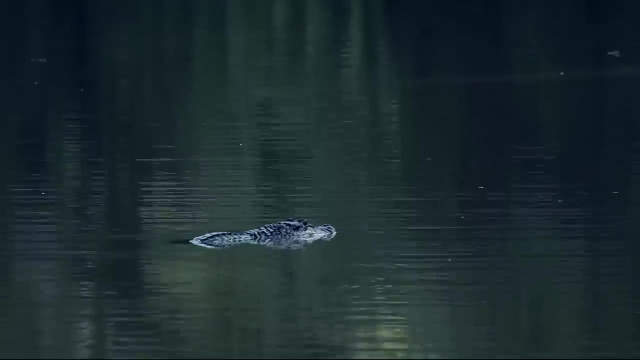 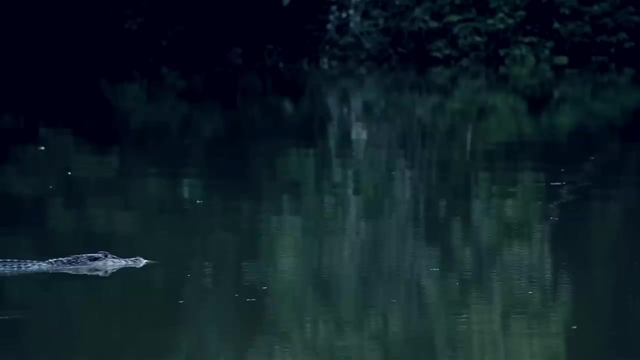 The current resident, a smaller male, is well aware and arches his back as a signal of his claim. The new, much bigger male responds in kind, showing that he won't back off so easily. As the caiman move in, they size each other up. 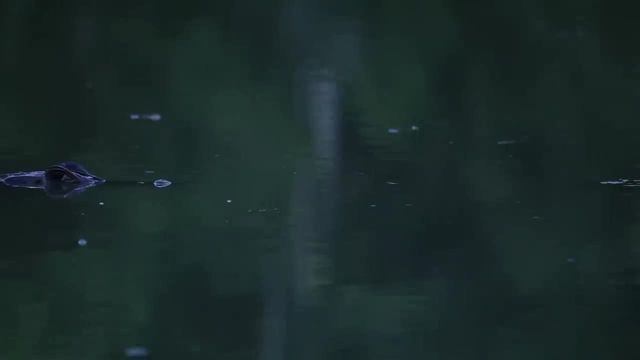 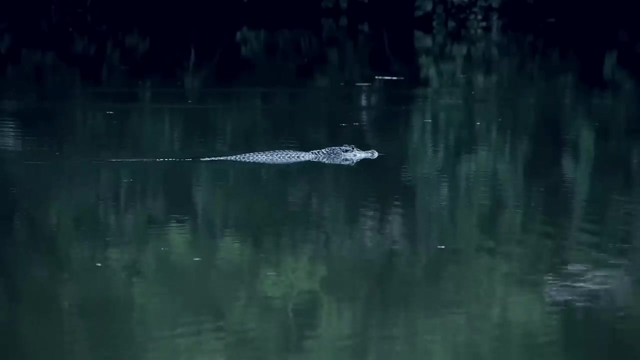 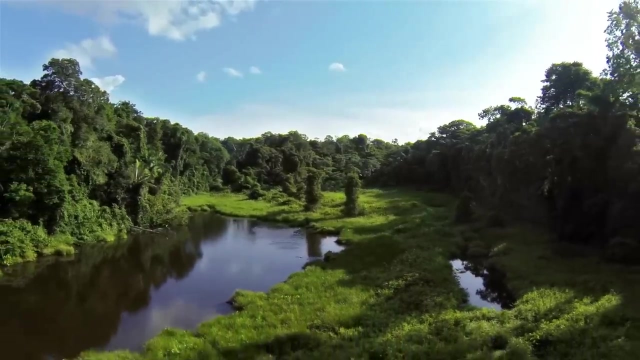 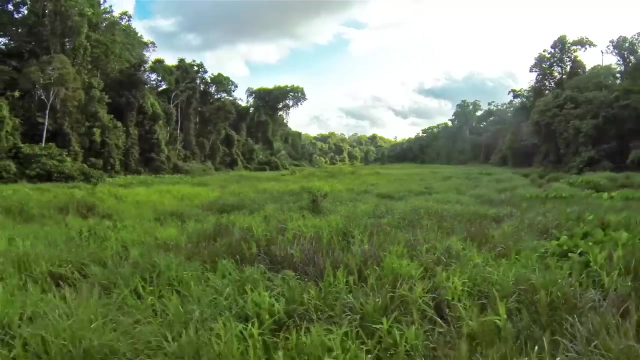 But the smaller resident male wisely backs off and the intruder succeeds in claiming these hunting grounds for himself. Some of these rainforest lakes are many hundreds of years old, But gradually vast mats of floating vegetation begin to choke the surface. The lake bottom grows shallower as it's filled with dead leaves and the forest moves in to reclaim the land. 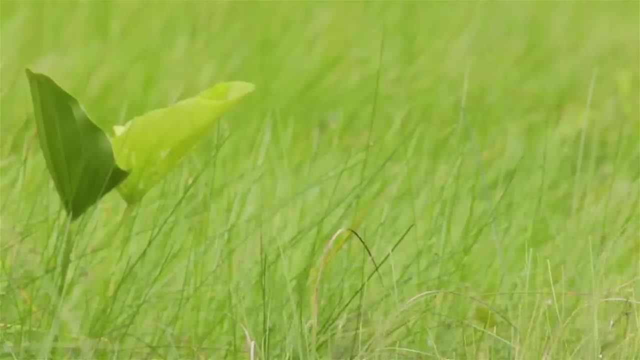 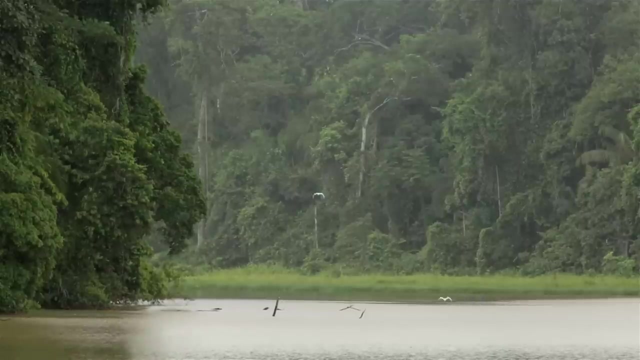 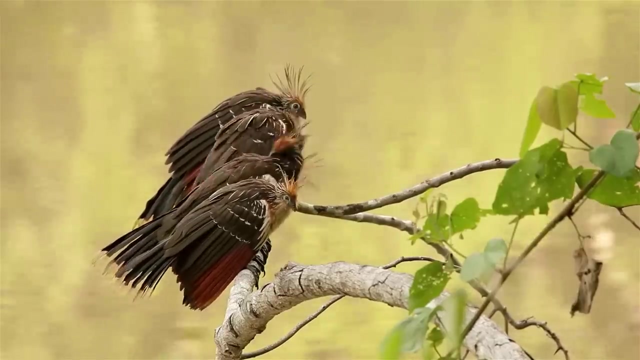 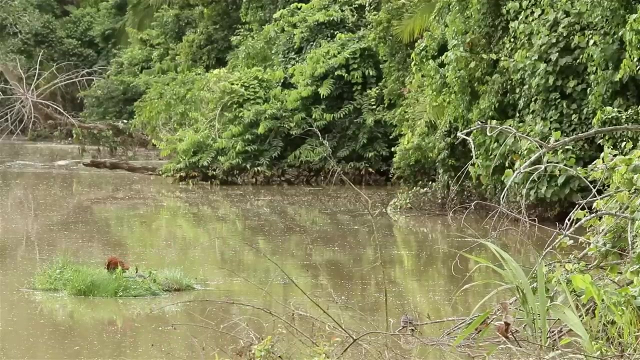 For now, this lake is a haven for wildlife of all kinds. These prehistoric-looking hoatzins find safety on the perches at the edge of the lake, where the predators of the forest floor struggle to reach them. This is the first time I've seen a caiman in this condition. 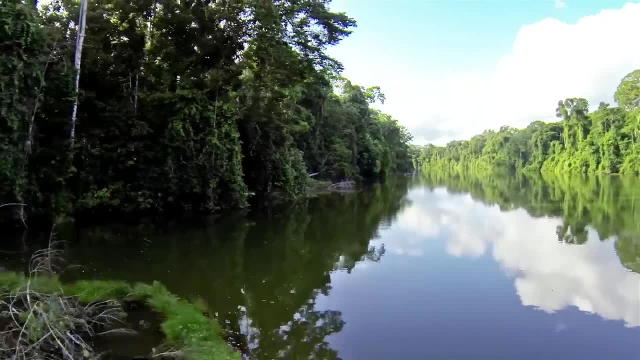 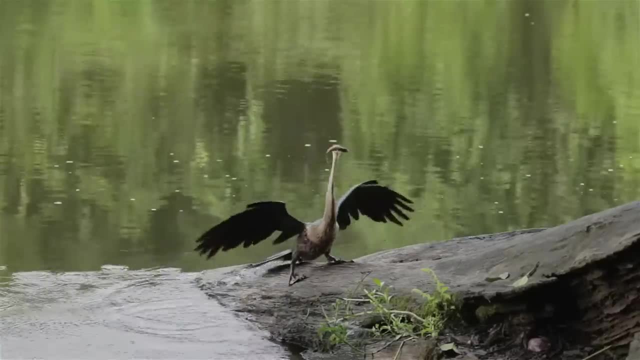 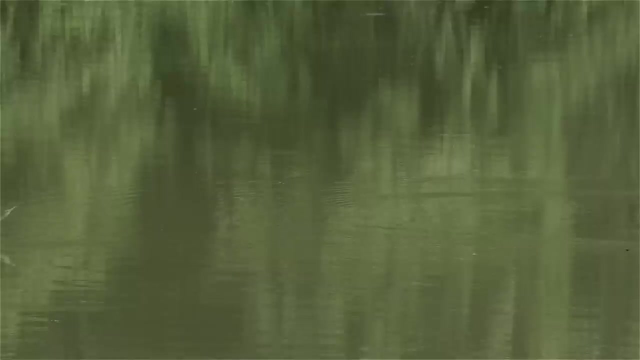 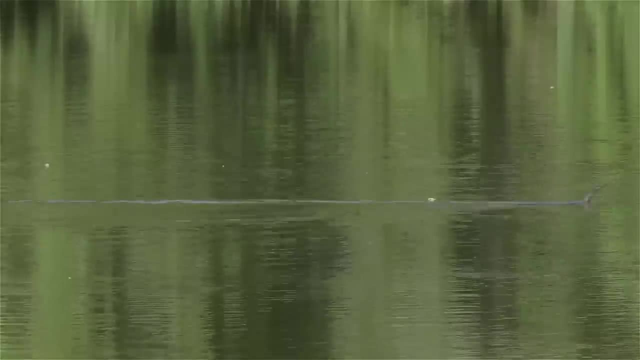 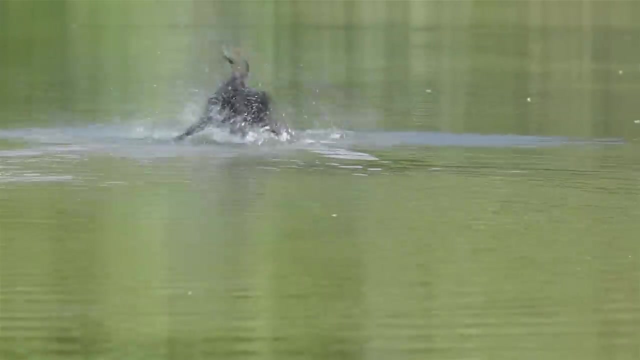 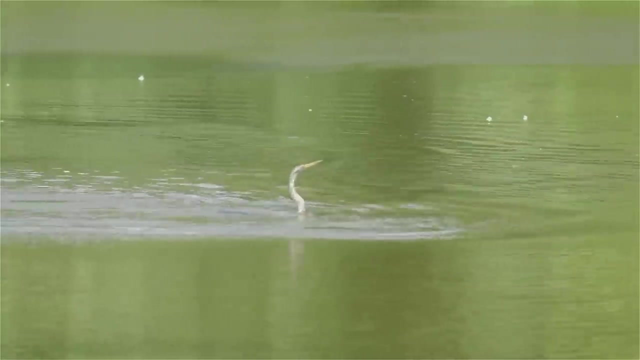 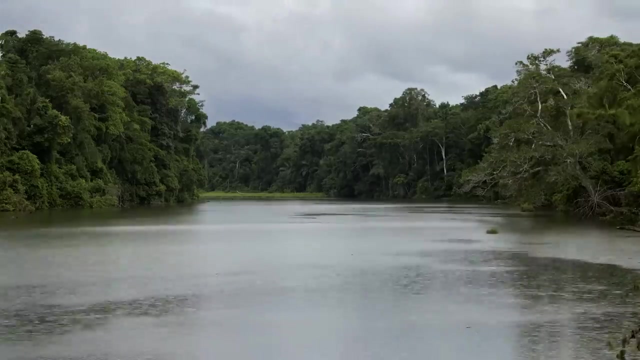 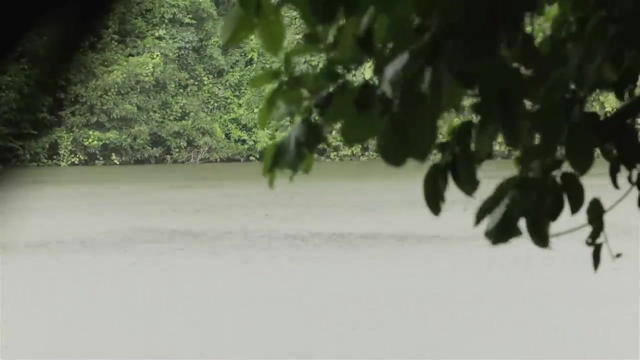 While a low buoyancy submerges their body while swimming at the surface, it also enables them to dive down and spearfish underwater more easily. Prime feeding grounds are often fiercely contested. For many animals, the daily downpours of the rainy season, 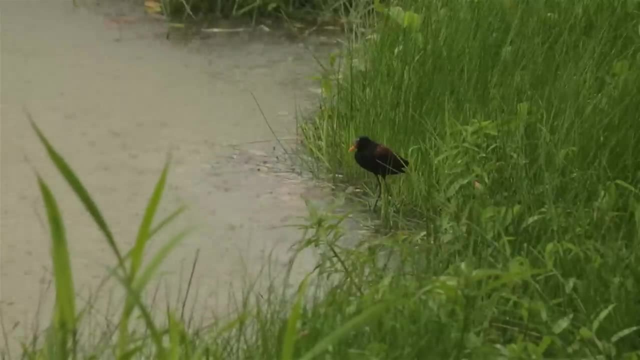 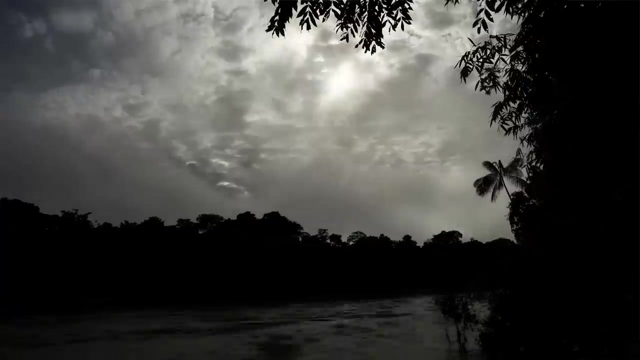 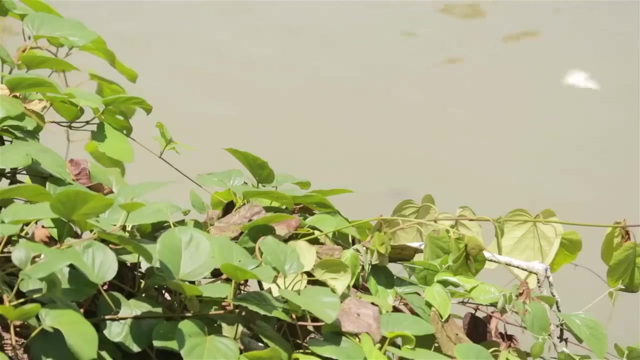 provide a welcome break from the stifling heat of the dry months, But for some they pose peculiar problems. The water has risen and the butterflies that once fed on the mud banks at the lake's edge must now look elsewhere for a meal. 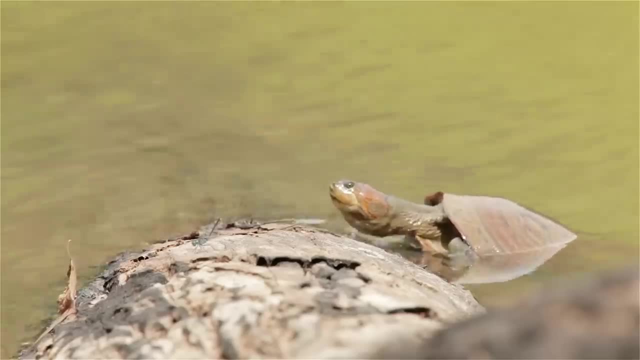 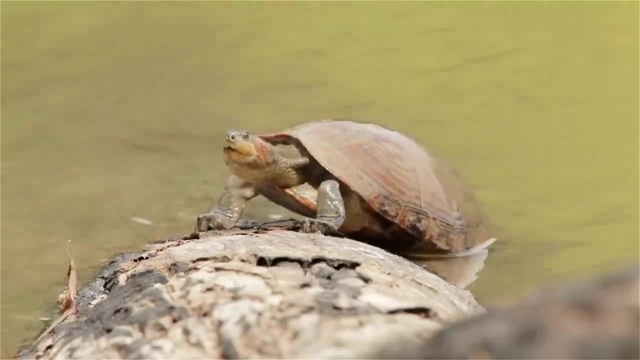 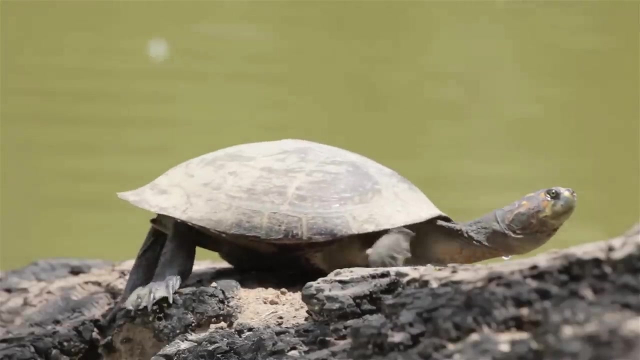 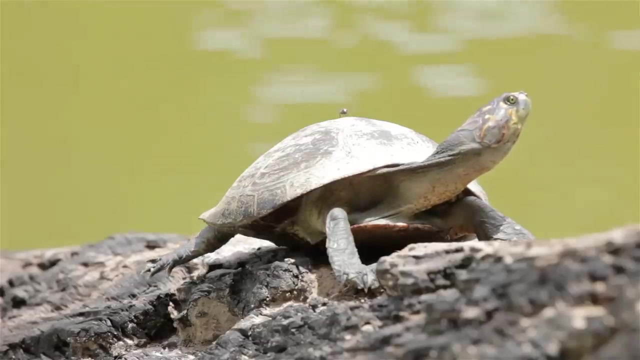 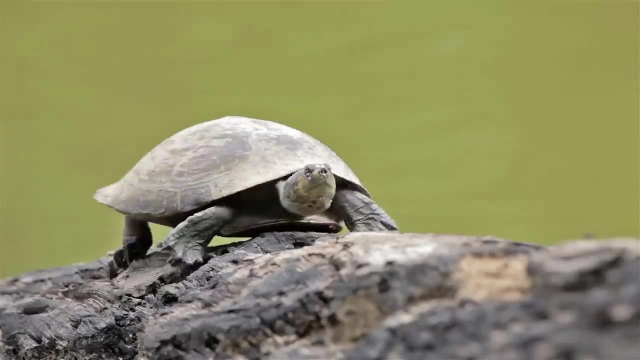 They may have to wait, but they know just the place to get it: Side-necked turtles who currently have entirely different agendas. There is nothing quite like a good scratch, Or, better yet, a good stretch In the rainy season. young turtles must make the most of the brief spells of sun. 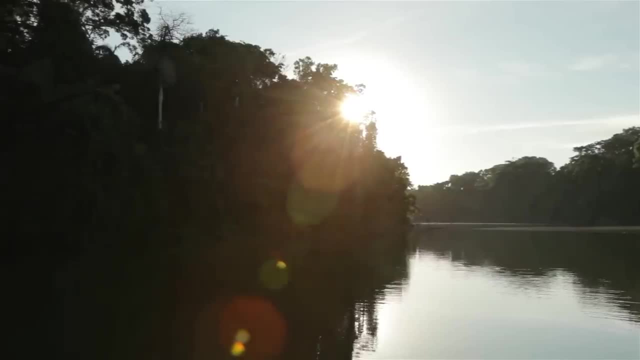 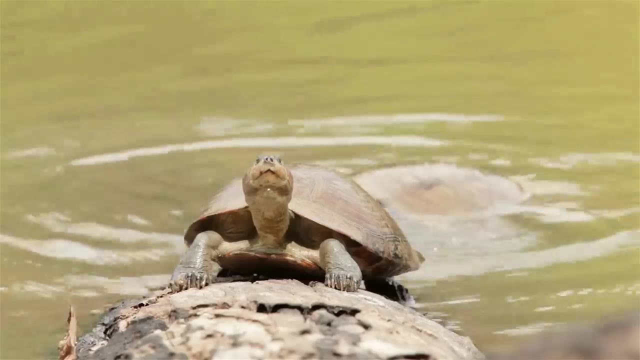 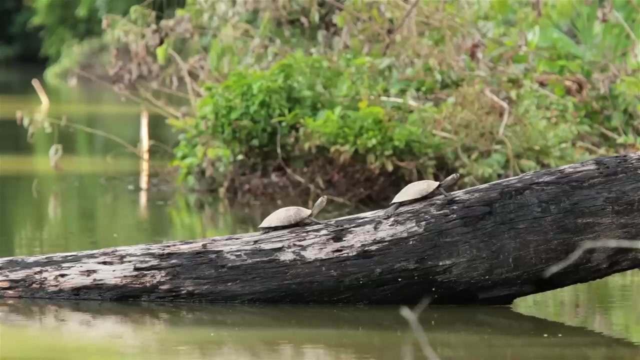 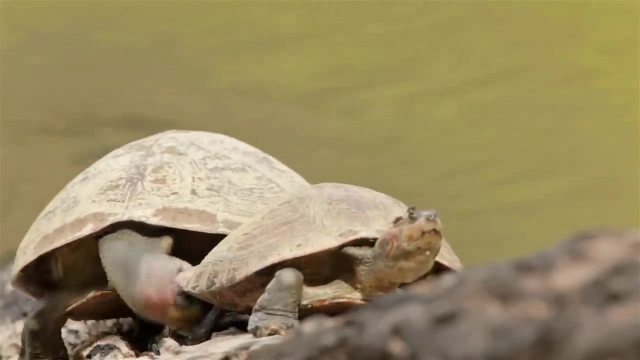 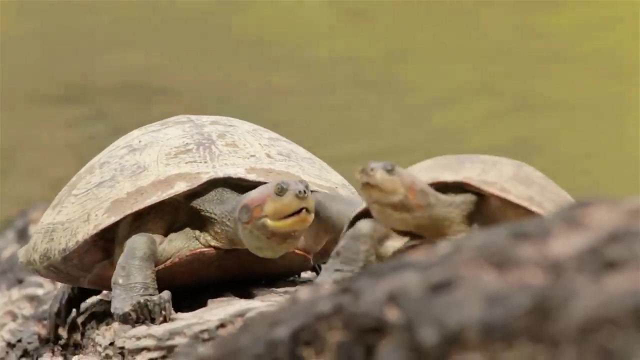 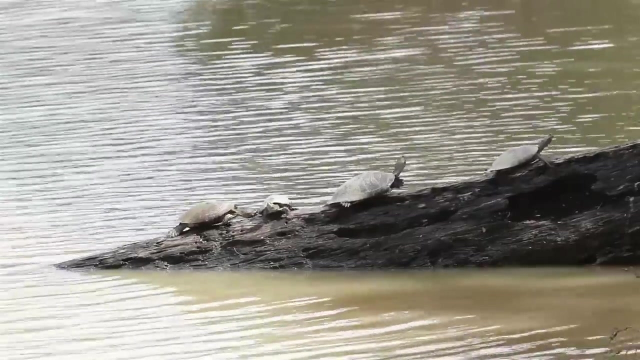 A good sunbathing log is hard to come by, so they rarely get it to themselves for long, Despite there being ample room for many turtles on the log, a big male won't tolerate his view being obstructed by a smaller one. In turtle society, size is everything. 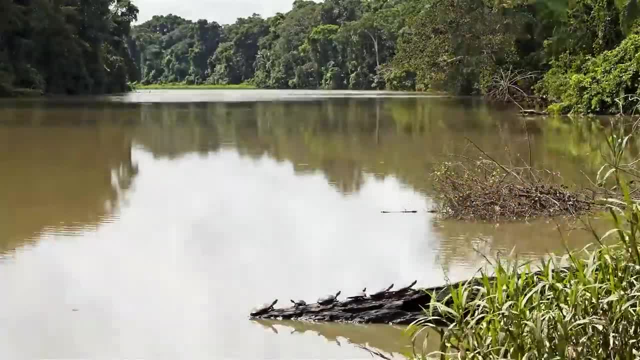 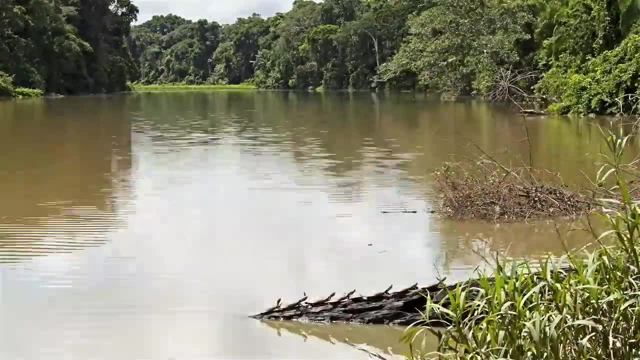 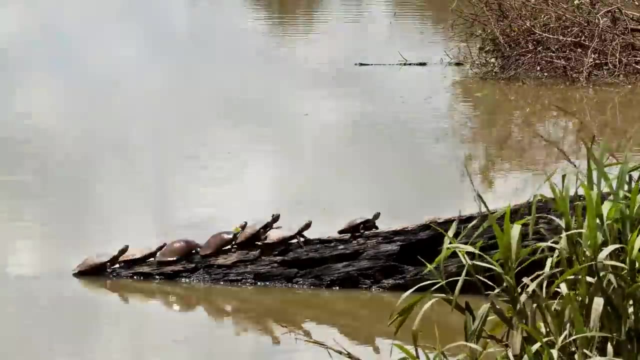 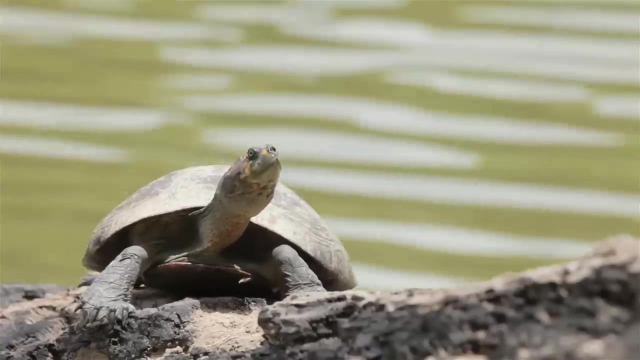 When the turtles are more evenly matched, log relations are more respectful, But as a consequence, they often tend to pile up. Life on the log is a process of constant nudging and shuffling. Once the turtles have settled, the butterflies can move in. 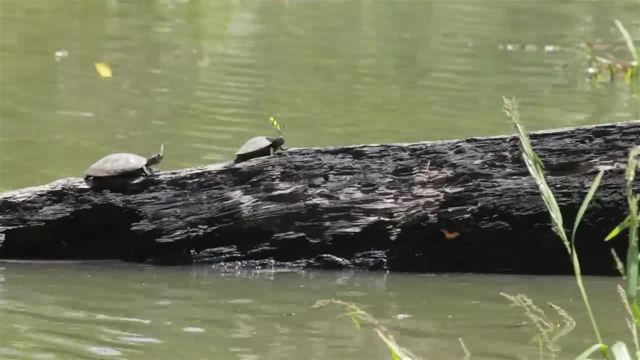 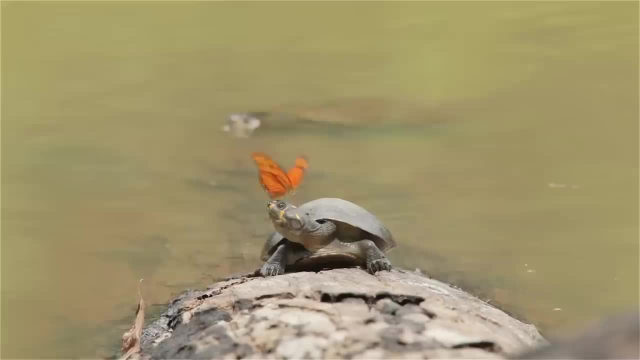 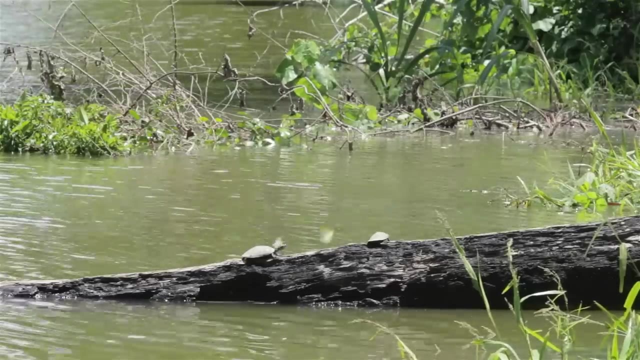 The butterflies lap up the salty turtle tears. But the turtles aren't sad. The tears clean their eyes after a dip in the water. The butterflies don't actually consume the tears, they collect, They save them. These butterflies are all males and they will pass the tiny bundles of turtle tear salt. 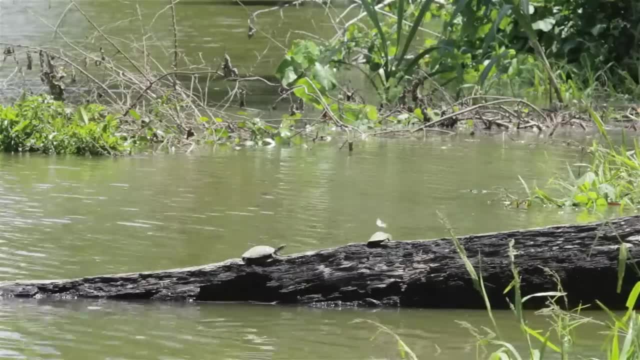 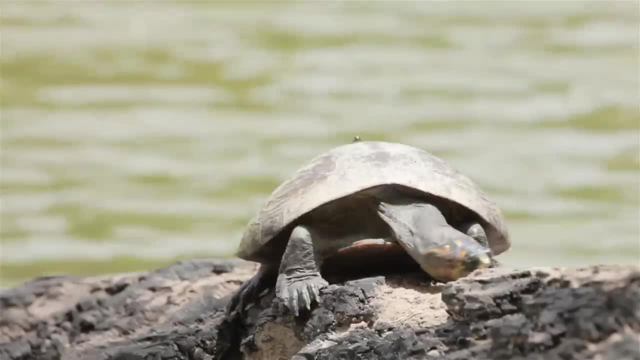 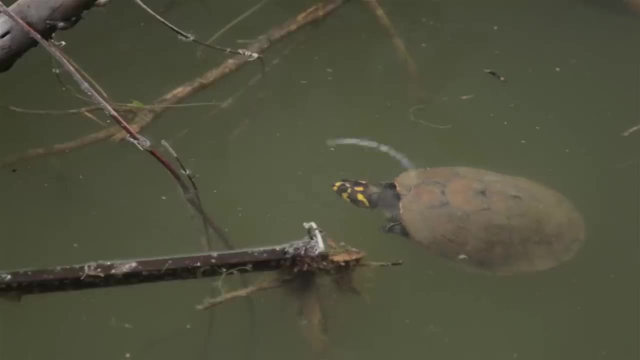 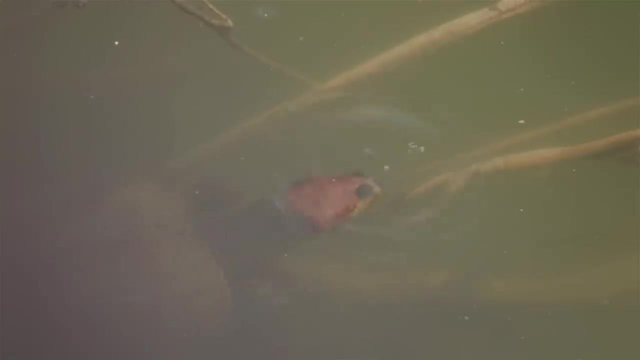 to the females during mating. For the turtles, butterflies are just about bearable, but bees aren't tolerated too well, So they have to slaughter them after mating. They're sure to be able to eat them, But if the butterflies have a little confidence, 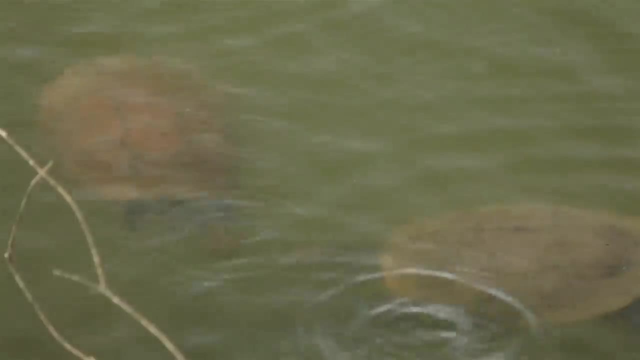 and take in the water, the turtles will still be able to do it. It seems that turtle relations in the water are not so different from those on the log. The bird that is born is different from those on the log: The bird that is born. 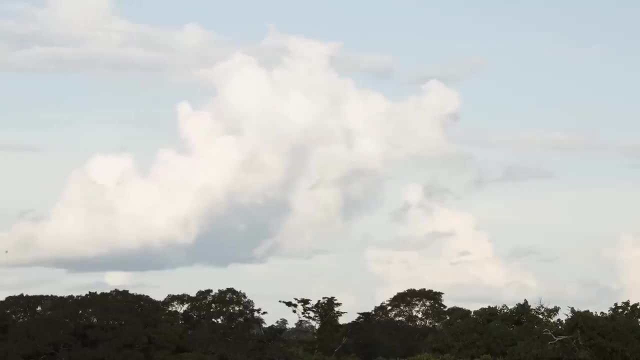 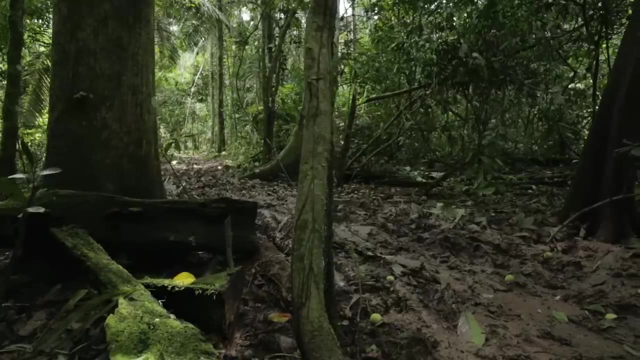 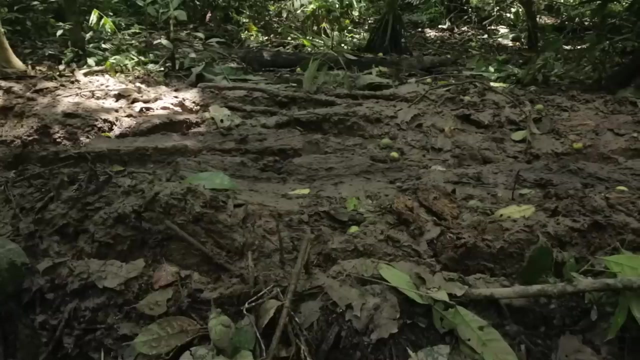 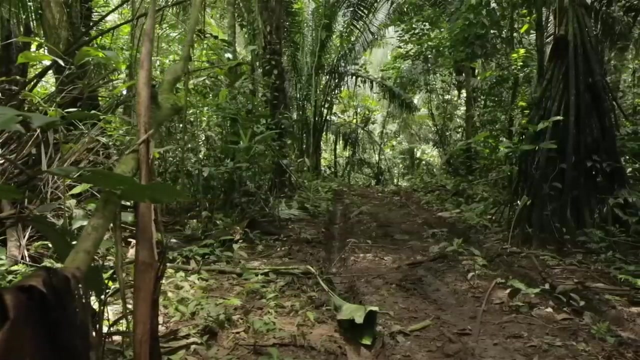 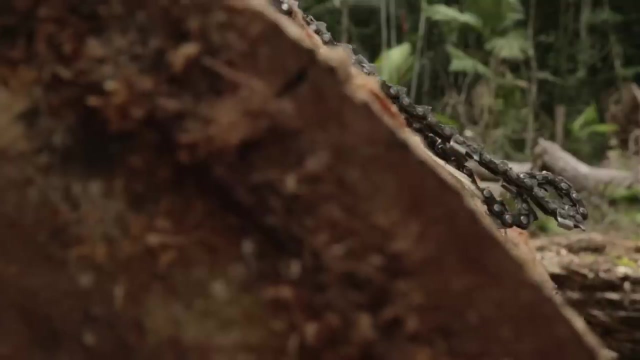 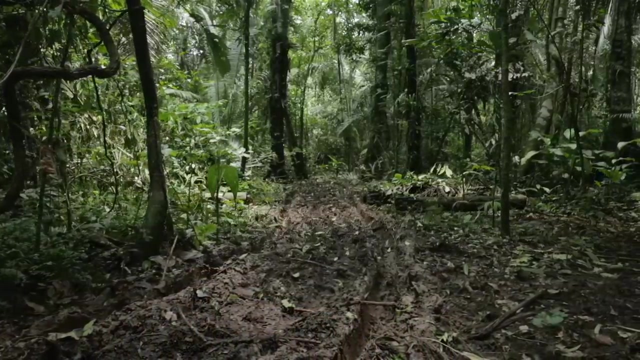 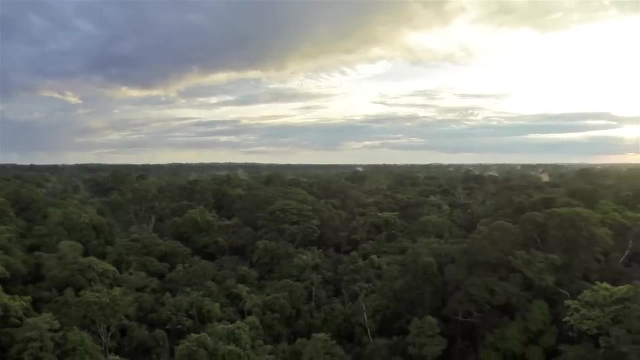 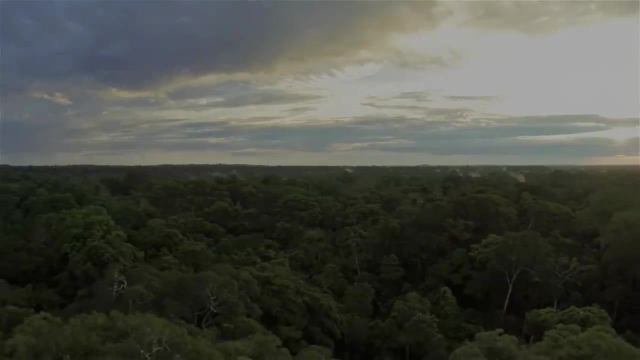 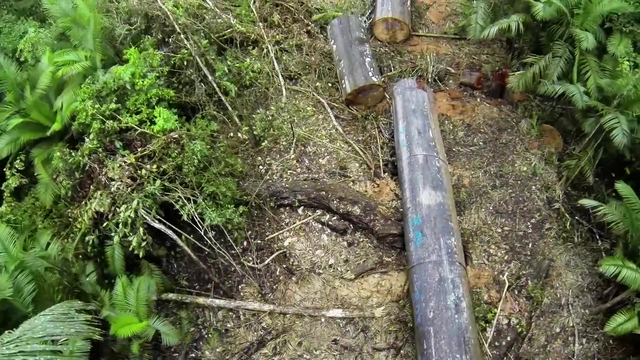 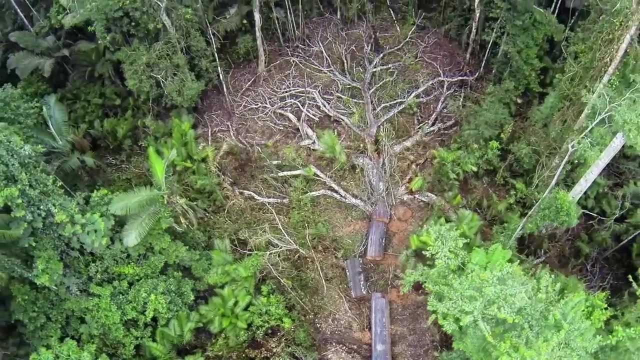 is different from those on the log: The coming of the rainy season, return of another species, a species so ingenious that, like no other, it has the power to shape the rainforest in its own image. What happened to the natural processes takes centuries to build. 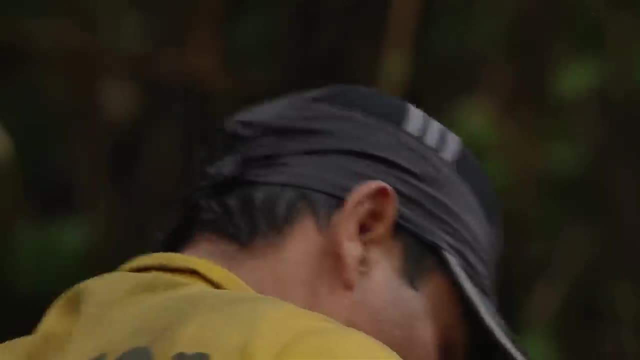 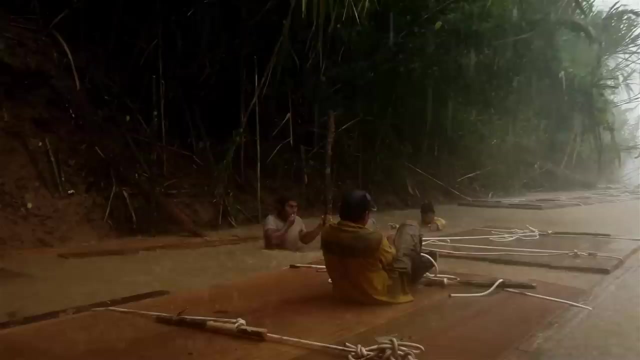 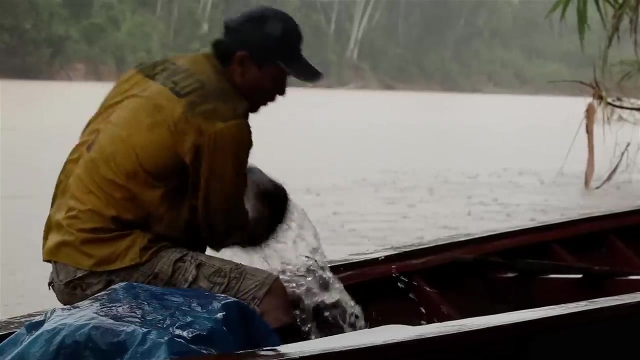 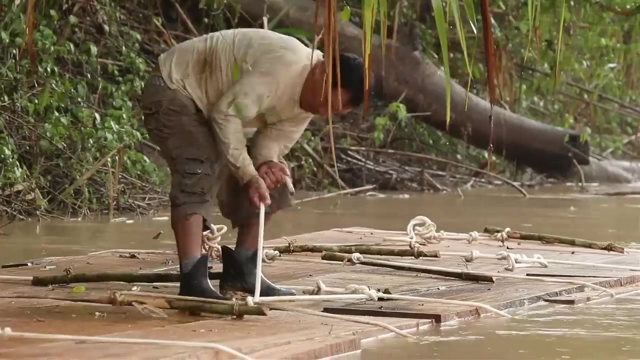 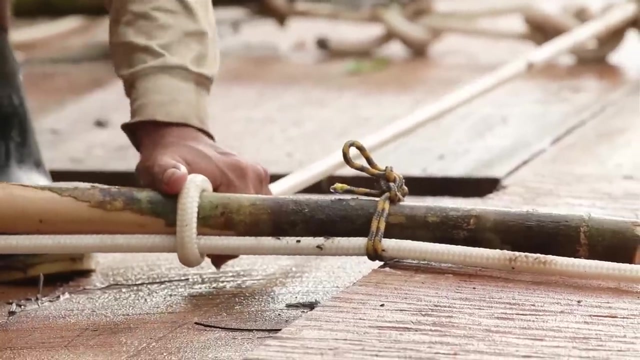 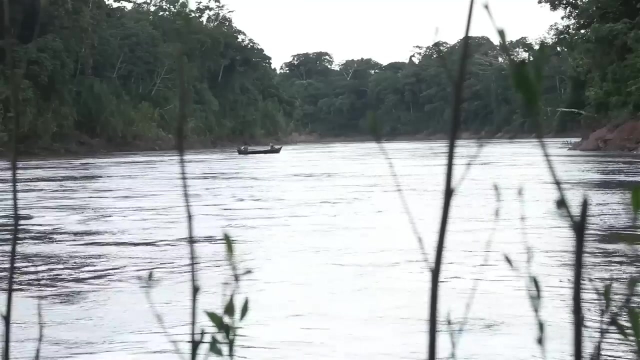 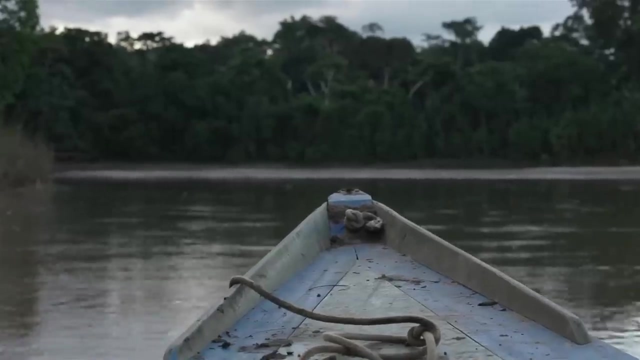 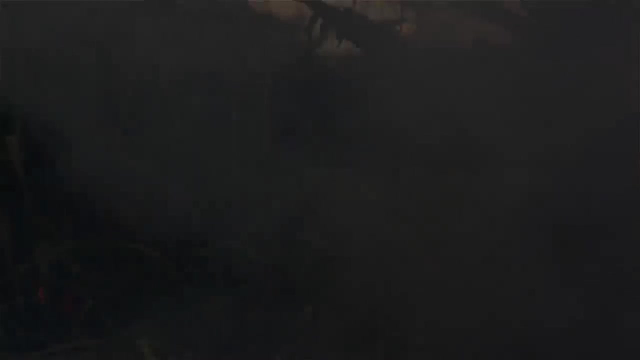 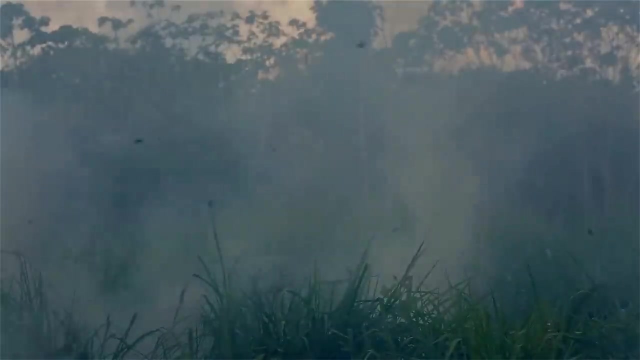 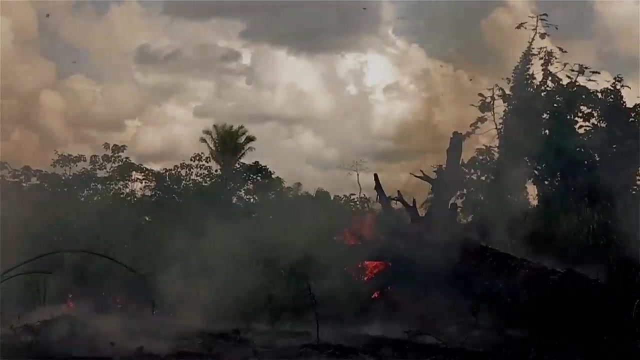 I love you, I love you, I love you. Once the rats are completed, the wood must be taken to the edge of the rainforest. But at that edge, the world is changing As the Las Piedras rainforest is burnt to make way for farmland. 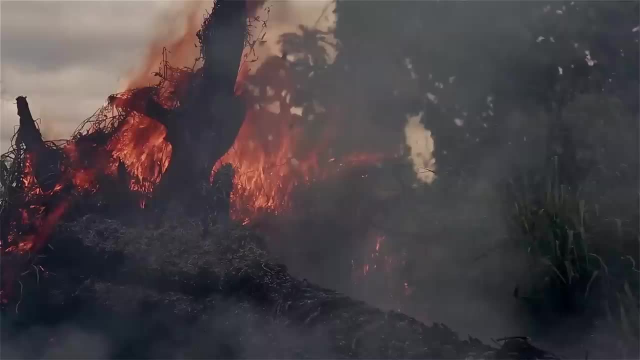 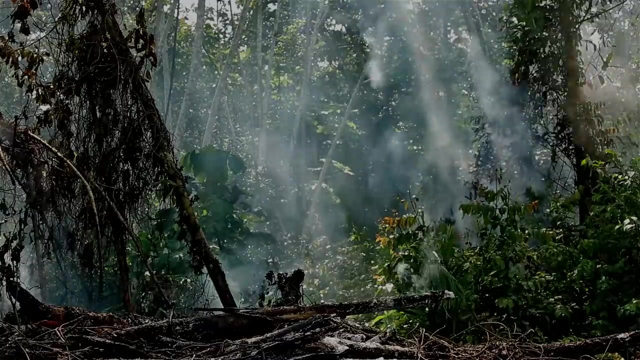 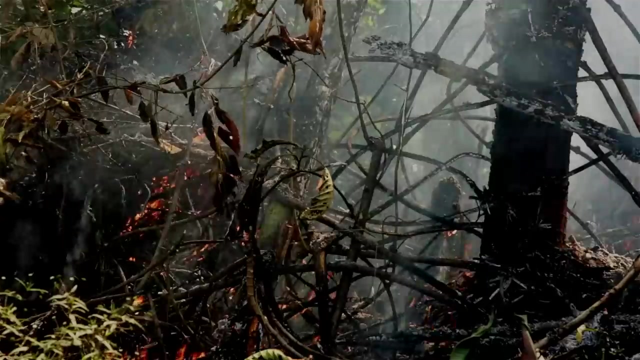 a part of our sense of wonder in the world goes with it, As the Las Piedras rainforest is burnt to make way for farmland. a part of our sense of wonder in the world goes with it, As the Las Piedras rainforest is burnt to make way for farmland. 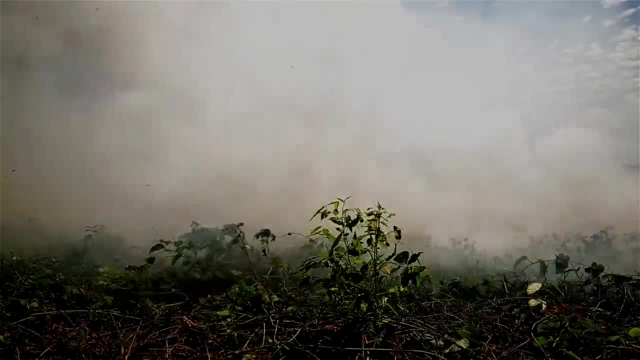 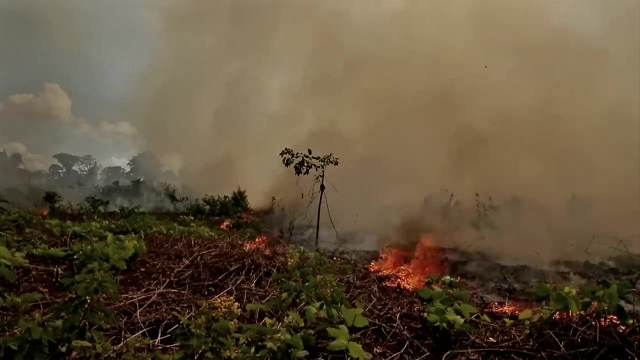 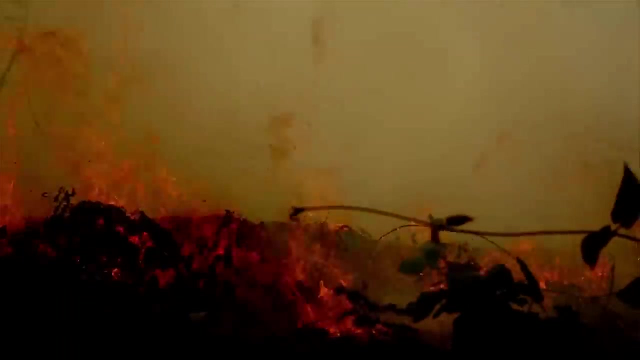 as the Las Piedras rainforest. as the Las Piedras rainforest is burnt to make way for farmland For animals, in this rainforest, millions of years have been spent finding ways to cooperate to try and beat the tide of war. All of our knowledge has been laughable, just like a pre- Benedicte's fortitude in the trotzdem brain. 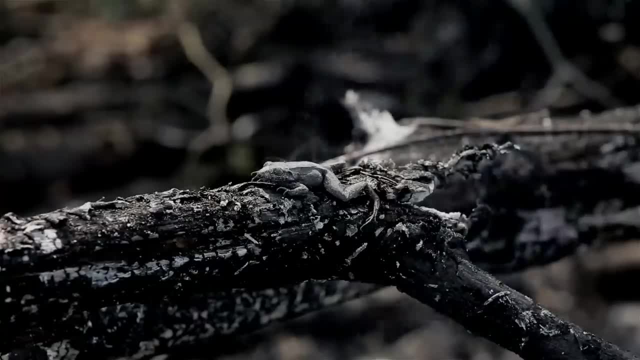 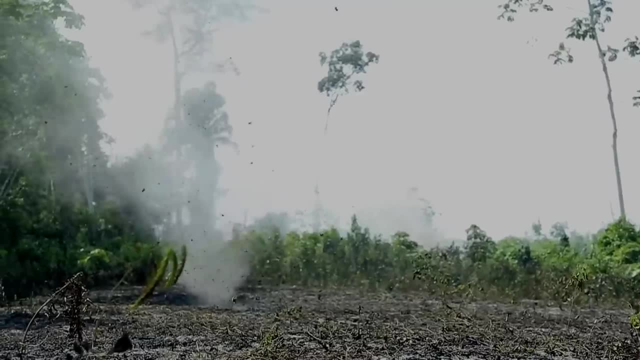 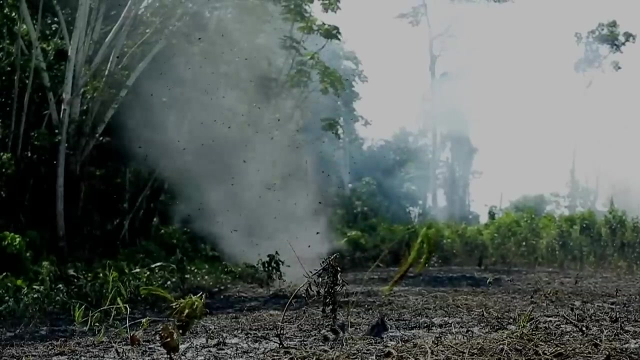 thanks to which we have an infinite opportunity to overcome the unforeseen. In Japan, wild animals are shutdown from normalization, ways to cooperate, ways to compete and ways to survive. Yet these efforts pale in comparison to such a force. Nothing in nature could have prepared them for this.